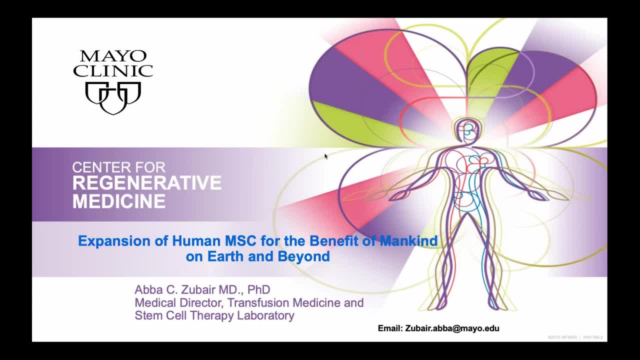 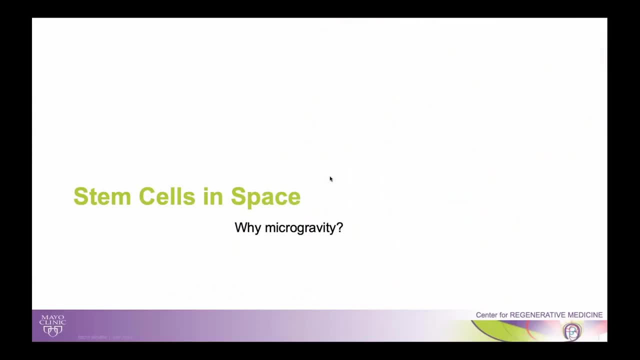 that would form a platform of future human application of space-grown cells. So why taking stem cells to space And why do we utilize microgravity? I think the short answer lies on this principle. Obviously, we're talking about growth or expansion, So at the heart of it, 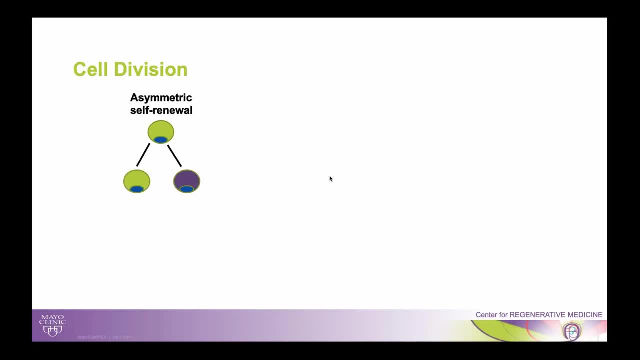 is cell division, And when stem cells in our body divide, they undergo what we call asymmetric self-renewal. Basically, one stem cell would divide into two daughter cells. One daughter cell would retain all the characteristics of the parent and stay as stem cell, while the other continue to. 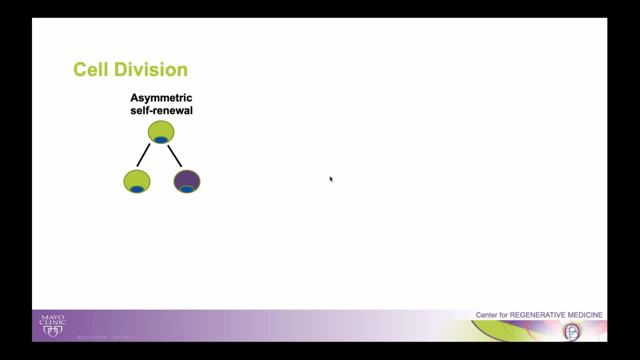 proliferate and give underweight. So in this process stem cells are able to maintain their number constantly. So it's much harder to really expand stem cells, even though we found tricks in the lab where we can expand them, but inherently they are designed to keep their numbers. 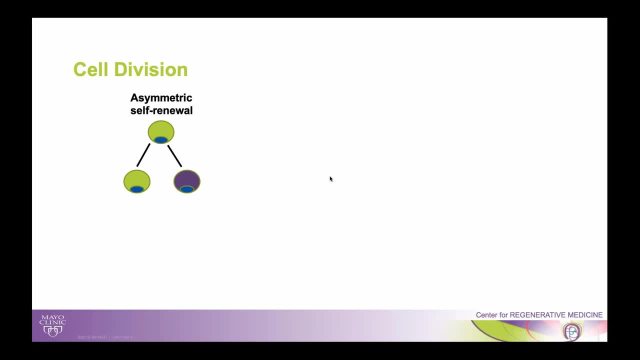 so that at any given time the proportion of stem cell is about the same, which is a big challenge if you are planning to expand and grow cells for a number of patients- not just one patient, but giving it to multiple patients. So you need to grow it, and that's the challenge. 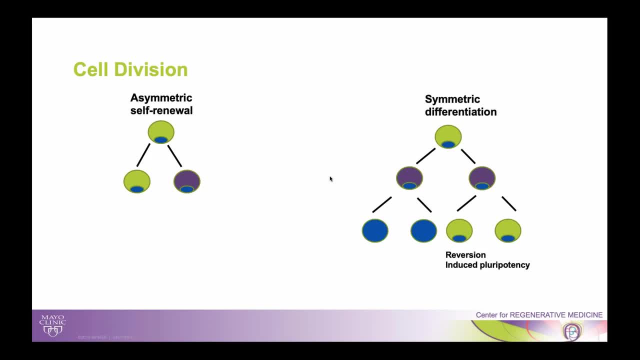 If you normally cells that are not stem cells and that will symmetric differentiation. So basically the cells divide and they do the two daughter cells. So if you look at the stem cell, you can see that the daughter cells do not have the characteristics of the stem cell And these daughter cells further differentiate to give different types of cell. 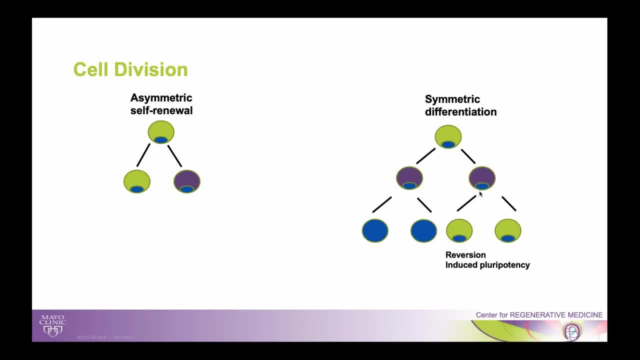 Obviously, with induced pluripotent stem cell technology you can reprogram the daughter cells to be back to having stem cell characteristics. So the main question is whether we can be able to copperけて a stimulating tissue, like in the US, or whetherażs these and the reproductive 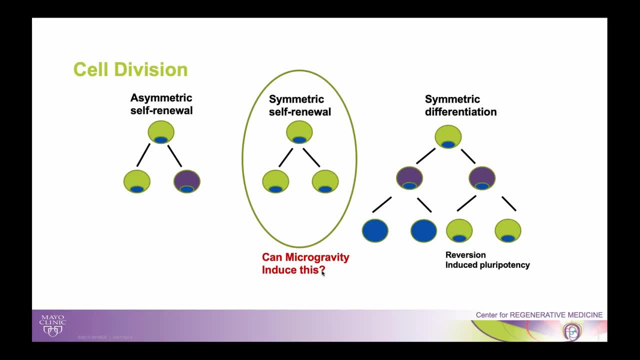 system can induce symmetrical cell expansion, stem cell expansion under macrogravity conditions. We know gravity plays a role in virtually all our physiology. political energy demands againł: How much is gravity? 10 increaseпр be a lot more like a lizard or something that is more flat, because the gravity there is. 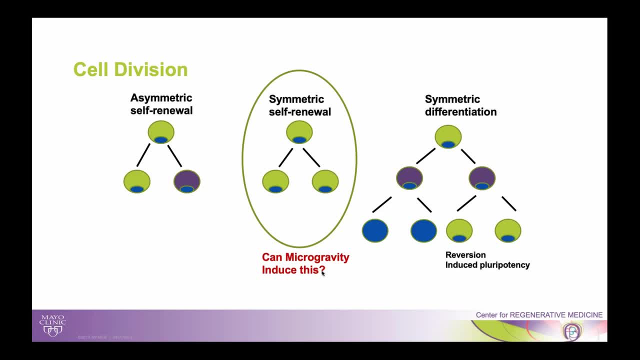 much, much more than on Earth. So we know that gravity play a role in cell division, in chromosomal segregation. We also know a gravity impact on gene expression as well. So the question is: if you take it out, would you be able to reprogram these cells safely? 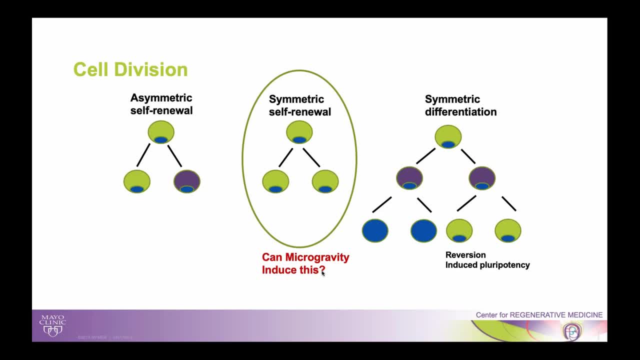 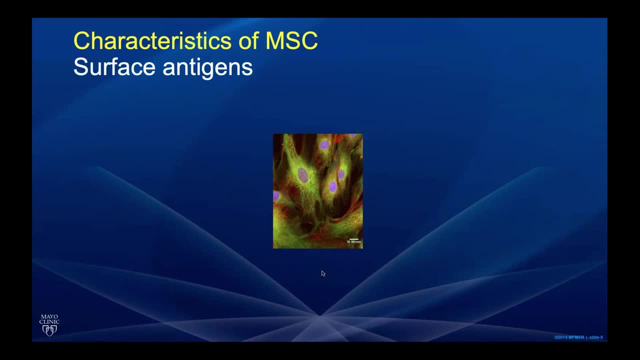 to expand without making them unsafe. So we chose mesenchymal stromal cells. Some people call it stromal cells, some call them stem cells. So MSCs are actually maybe the most common or second most common cells that are used clinically in the regenerative medicine. 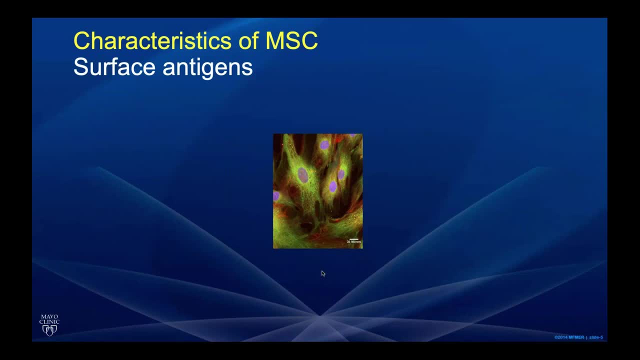 They can be derived from bone marrow or cord blood, cord tissue or adipose sites, so from fat. So the access is quite reasonable. They are defined by some markers- CD73,, CD90, and 105, or absence of some markers which are mainly differentiating them from hematopoietic. 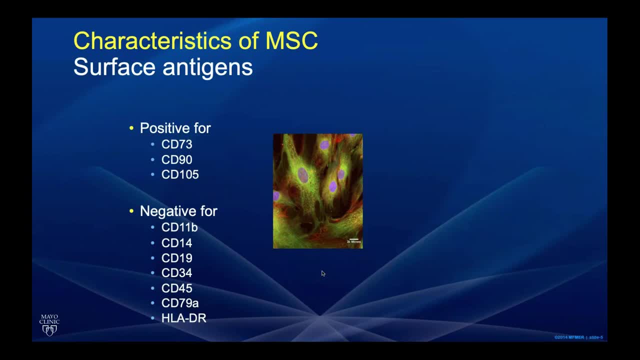 cells. Okay, That all these markers are not the same. Okay, They are not unique to the MSCs, but a combination of them. kind of define the MSC, The International Society for Cellular Therapy. also add to this definition that MSCs should have the potential. 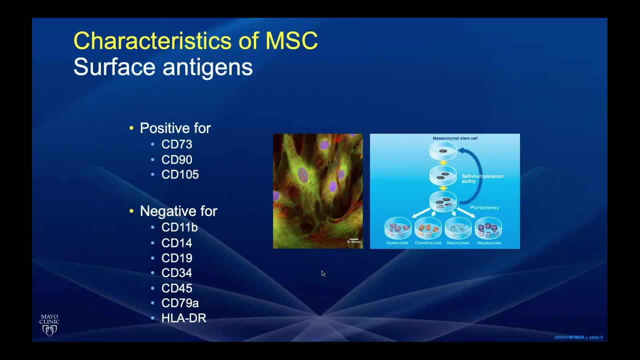 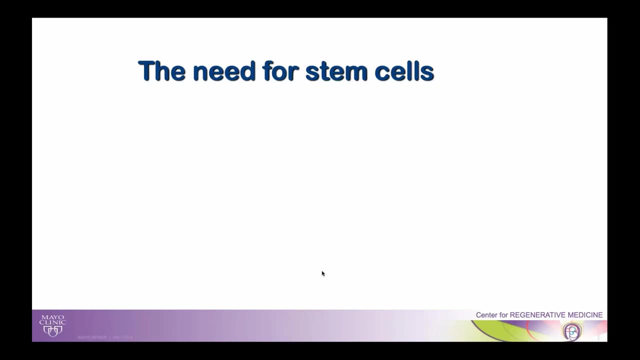 to differentiate into bone, cartilage or fat. So osteocyte, chondrocyte and adipocyte is one of the key characteristics of MSCs. So I started by mentioning that. obviously, stem cells are used clinically and so they are highly needed. Patients can donate their own stem cell, but not every patient are able. 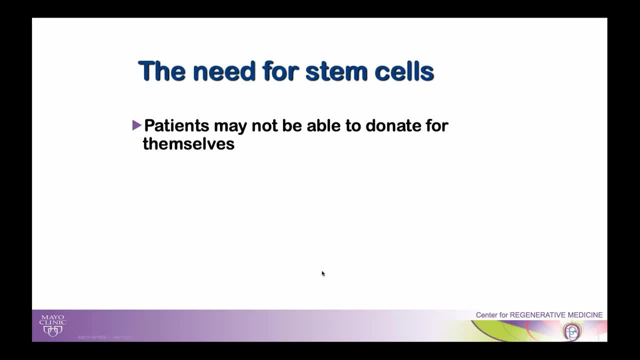 to do that. Some of the patients, for example, that have leukemia or lymphoma- they have multiple stem cells. Okay Okay, marrow may not be adequate for even donating the cells. Some cells themselves are damaged. So there is definitely need to have a donor, or a healthy donor, to donate, But there aren't. 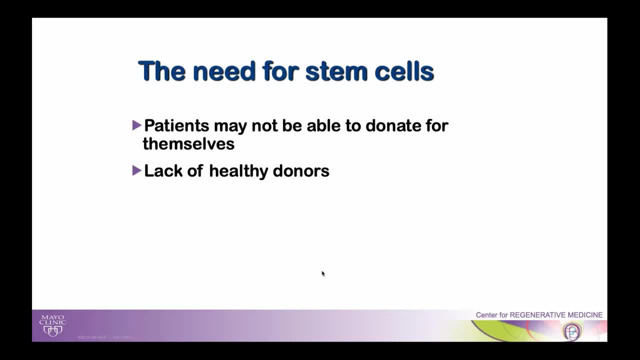 many healthy donors that are available to donate And then, even if they do, it's harder to expand the cells to treat more than one donor And we know, based on the bone marrow transplant activities that we do, we need about 200 to 500 million stem cells to achieve. 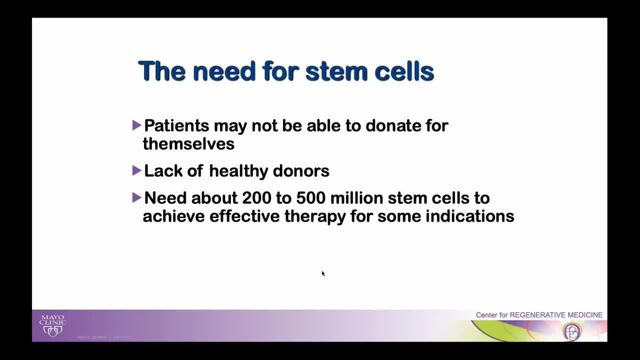 therapeutic efficacy, Again in the setting of, let's say, leukemia, lymphoma, Of course, some application where you are putting the cells locally. you may even need just 5 million or 10 million or more, But regardless, you need a lot of cells to treat a lot of people, especially if you have 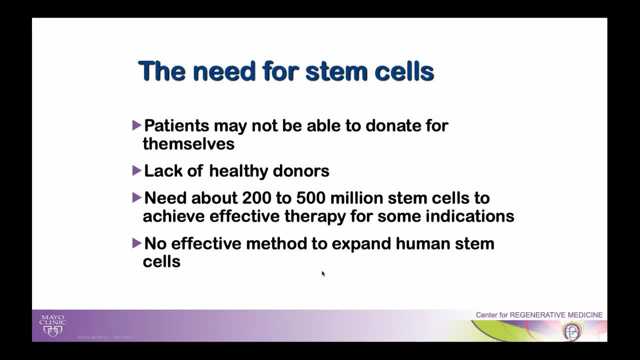 one donor donating to multiple recipients. So we don't have effective method to really expand the cells. We do have some method but it takes time. At a minimum you need about a month to grow a reasonable number of cells to treat a few patients And even. 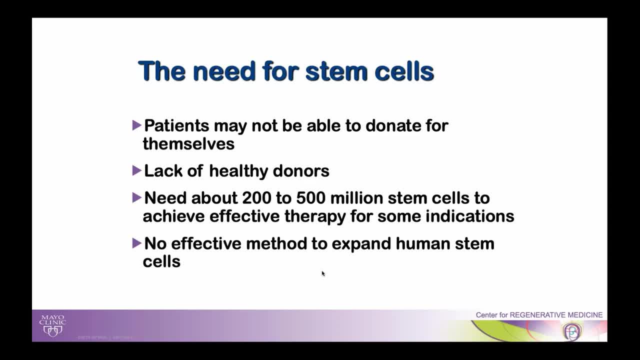 if you need up to like 200, 500,, you may need a month to grow a reasonable number of cells to treat a few patients. And even if you need up to like 200, 500,, you may need a month to grow a reasonable amount of cells to treat a few patients. And even if you need 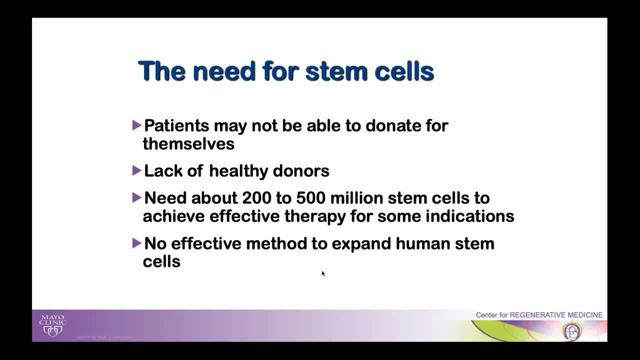 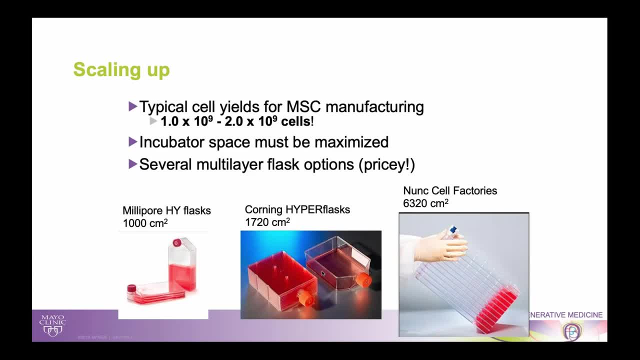 a lot more, or you need a bigger facility, a lot more sources. So scaling up is always a challenge and you can see that. you know the space are limited. you need more incubators, We are using multi layer blasts. all of that and I even automated. 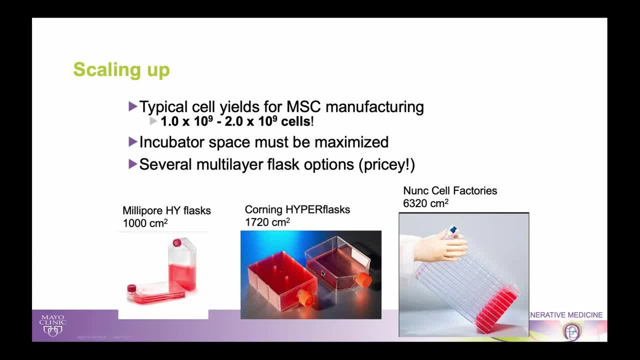 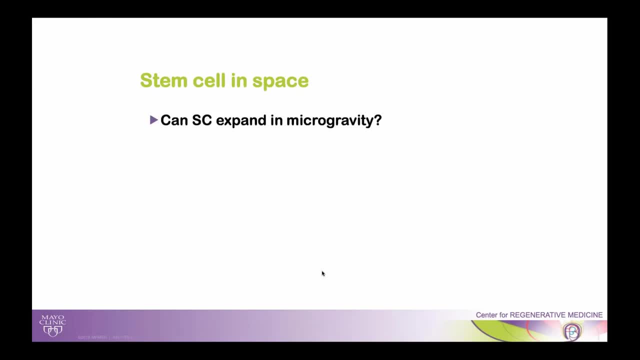 bioreactors. All of that is quite pricey and difficult and takes time. So we ask the questions in: can stem cell expand in microgravity safely? What is the feasibility of doing that, especially if you want to generate clinical grade cells, So yeah, so we want to evaluate the safety. 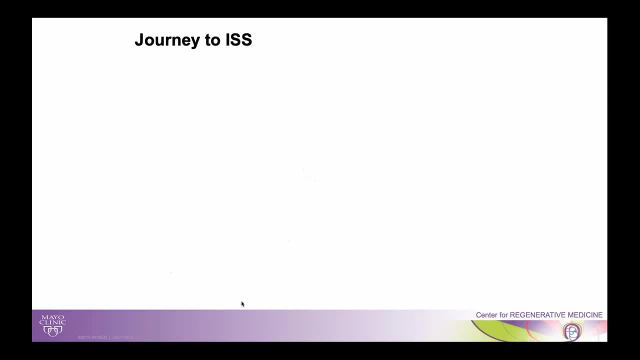 and efficacy of using these cells for clinical application. So obviously the journey to International Space Station was quite exciting. It takes time to get on the bus. What I mean by the bus? the only rocket at the time on the one is SpaceX that could take research. 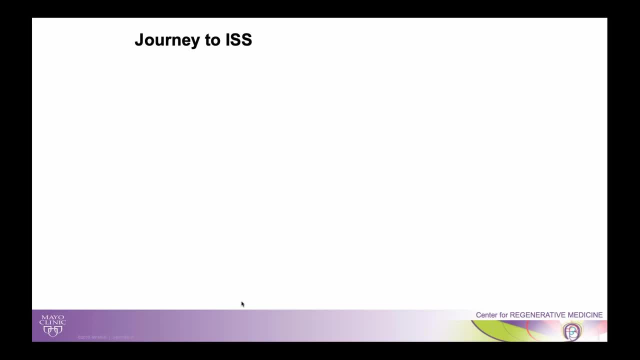 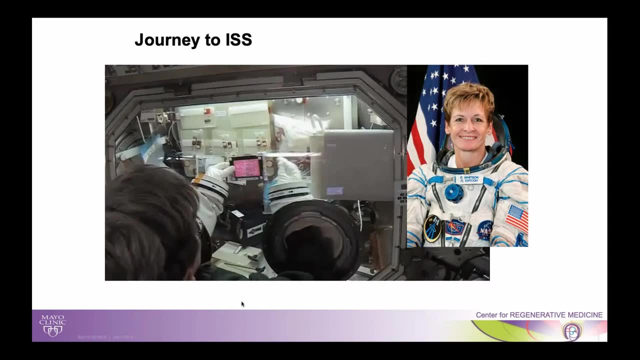 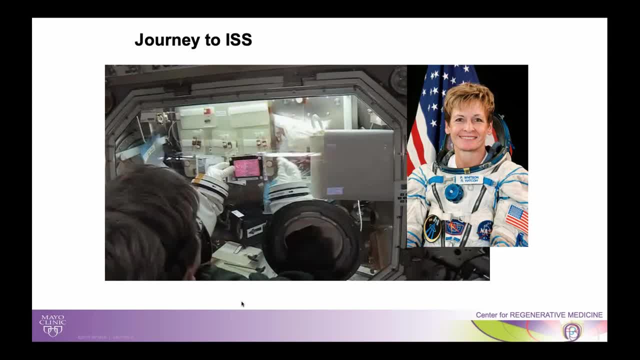 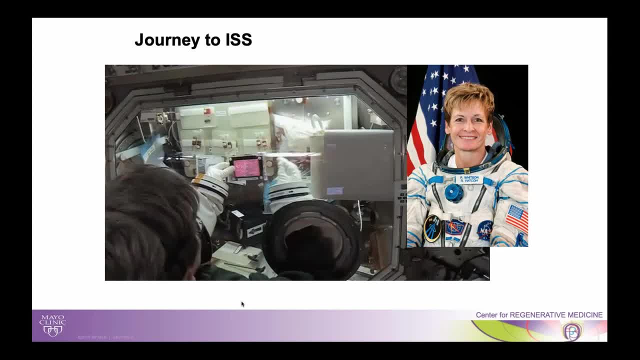 that worked on our project. so it is really a pleasure and a great opportunity to have an astronaut work on our project And luckily she also has a biology background, so that really helps. So what you are seeing is the container, that, the cassette that we use bio cell in collaboration with our implementation. 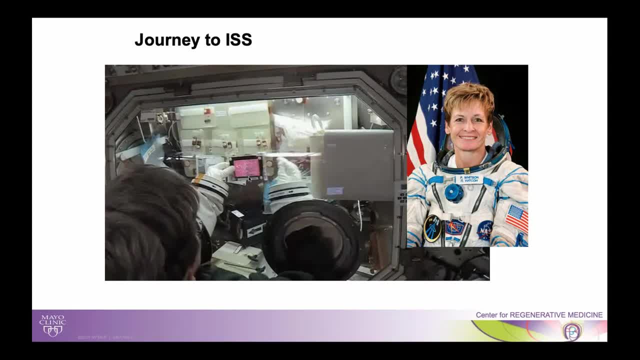 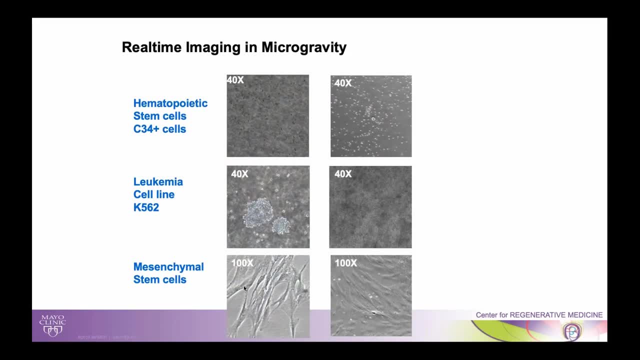 partner, which is the biocep from university of colorado. so that's how we were able to transport the cells in a p-hat and then to the international space station. um, it's quite challenging. um, we we had initially thought we can do a lot more at the station. 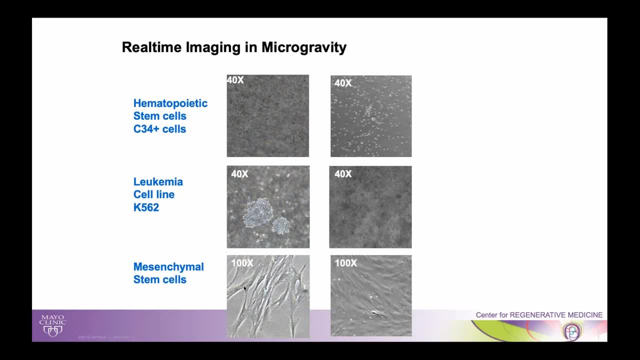 evaluating the cells. but reality set in, so we had to scale down a lot of things in part. you got an astronaut who may have up to 20 projects uh working on yours, so you are just one of the many uh who is not a really a basic researcher, who so you have to really scale down. and then the setup. 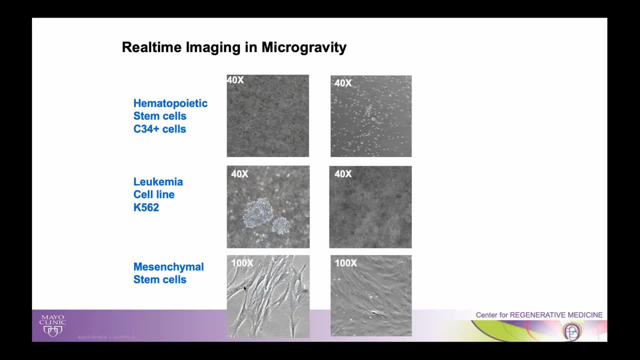 also takes quite some time, like the use of microscope and stuff like that, um, or media exchange. we have to even do away with that in space. but anyway, um, we, we took three different types of cells: hematopoietic stem cell, leukemia cell line and then the mesenchymal stem cell. 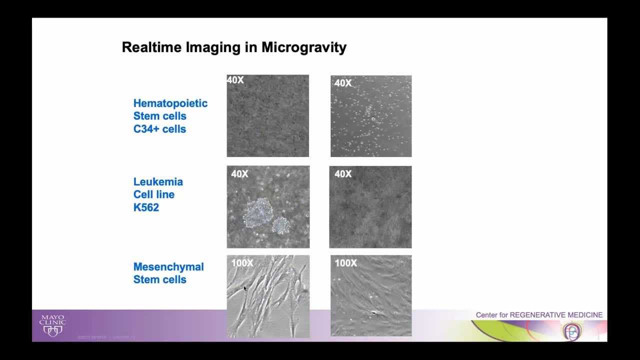 and so this presentation really focused on the mscs, but we also look at other cells. we were able to get real-time imaging as the cells grow and then we took the same pictures of the control cells in our lab and you can obviously see- it wasn't that clear, but at least for the leukemia cell line- the ones that are growing- 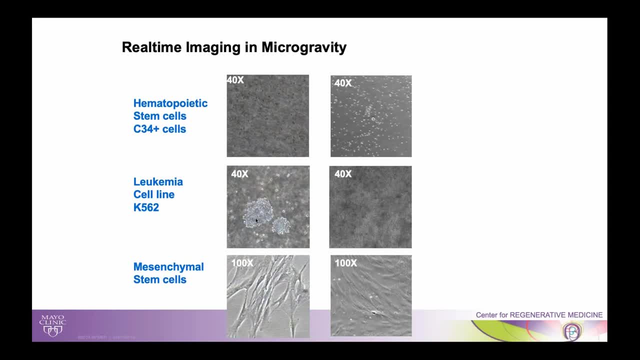 at the international space stations uh form clusters, um, while the ones that are growing in in our lab uh did it um. so, and you can see, also, it looks like the msc are kind of uh, more enlarged compared the ones that are in our lab. so, uh, but it gave us some clue, um, but that's all we could do at. 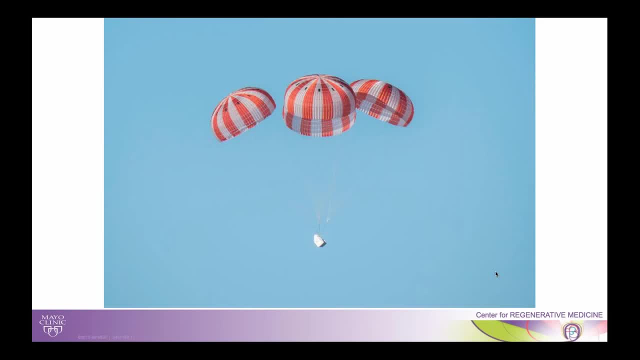 the international space station? uh, beyond imaging. we just uh, preserve the cells in multiple ways. uh, some in rna protect some because we want to preserve the cells because they're not as thin and you don't want some of the cell that's from other cells. uh, even though they have their own cells, they don't need very. 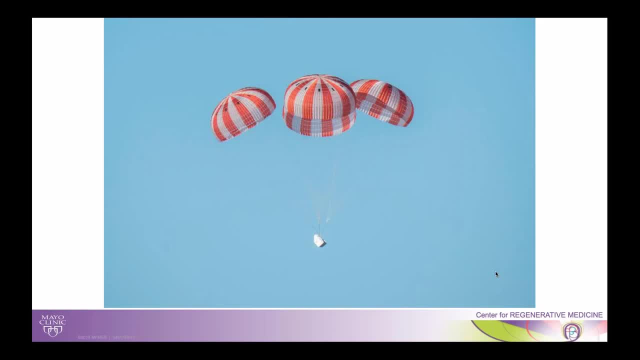 thick fat we saw on the lab they don't need to be too thin, or they don't need to be thin, or they don't need to be very thin. so now we ended up with about which cell group was going to become the highest when they came back here. so it was pretty odd. i was 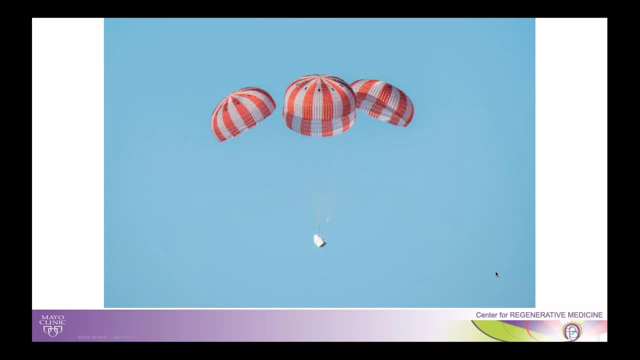 not sure if it was going to be the highest one, um, but we were suppose to be at the actual best because it is the highest level of the cells that are going to be the lowest in our lab capsule containing our product. it landed somewhere in the pacific ocean. you get fish out, i mean. 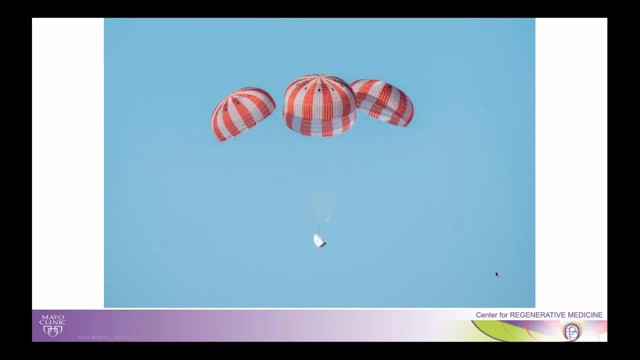 obviously using gps, and then actually our samples were mailed by pedex, so from you know international space station down to us and then the pedex pick it up and deliver the cells to us here at mail clinic florida. so it's quite remarkable that you can get yourself back by pedex and safely. 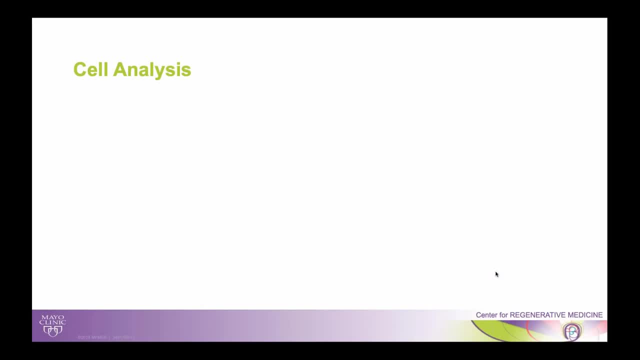 so when the cells get back to our hands, there's so much excitement and the people were asking what is the result? i tell people: well, wait a minute, that's actually. this reveals experiments that when we get the cells because we couldn't do much at the international space station, 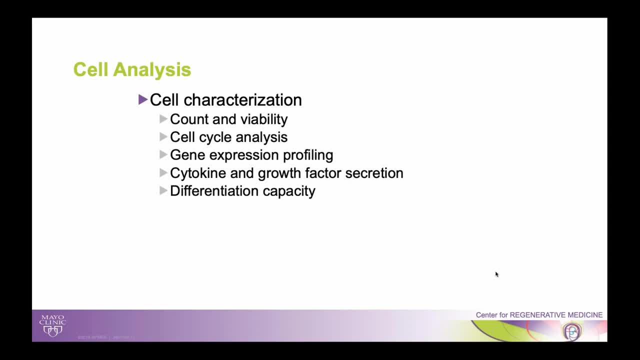 so and we were very careful not to like throw out all our cells all at the same time because these are precious samples. so we were very careful. but we we did cell characterization, looking at cell count viability, we did cell cycle analysis, gene expression profile and growth factors, and then 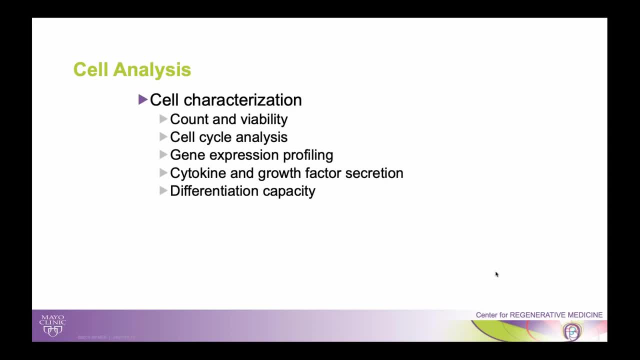 also look at differentiation. i may not be able to present all the data on this, but it was quite remarkable and more to come and we're still doing the analysis, the very important mission, for the objective for this mission is really safety of the cell, so we wanted to see whether there is any radiation damage. 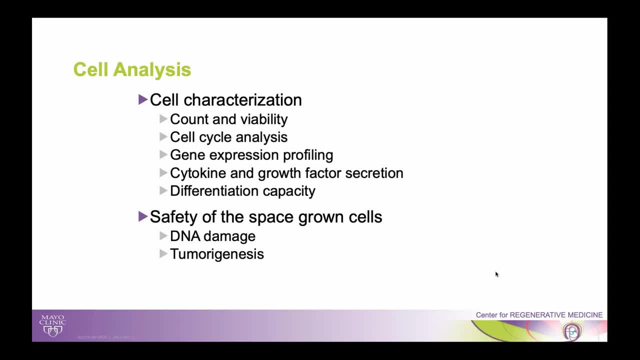 so like dna damage of the cells also what we wanted to see if they transform, so and then we want to see whether they have, they retain their regenerative capacity and induce tissue repair. so that is still ongoing and i wouldn't be able to touch on the efficacy beyond. 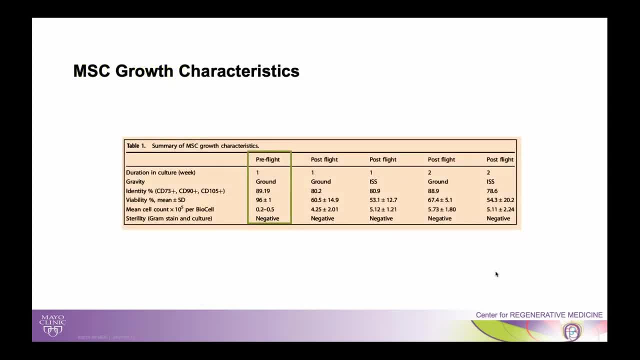 the immunosuppressive activities so quickly. um, these are the characteristic of the cells you know before flight. um, you can see the cell by uh identity that expressing those three markers is uh, quite high, 89 percent viability. uh in 96 um. and then these are the cells that we started with. 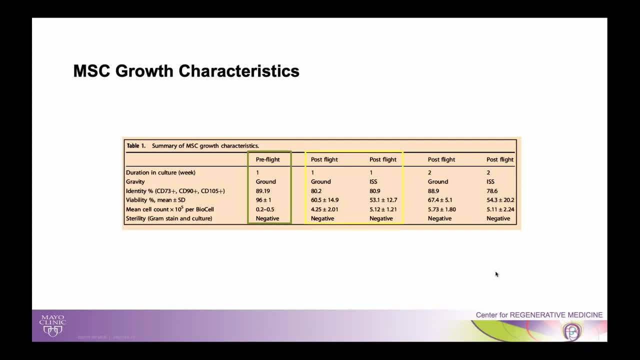 and we worked our way up here to get to the. viability is a little bit lower for the ISS compared to the one in our lab We are suspicious about. maybe this is just due to the way this has been cryopreserved. We didn't, we couldn't. 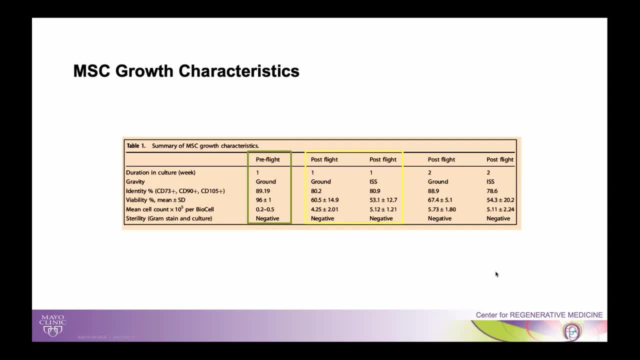 use control, rate freezing. but I mean obviously it does. it has traveled this far, so maybe the viability is a little bit less. The cell growth is also. actually we see a little bit more cells on average, but overall is within the error margin. We think that our growth 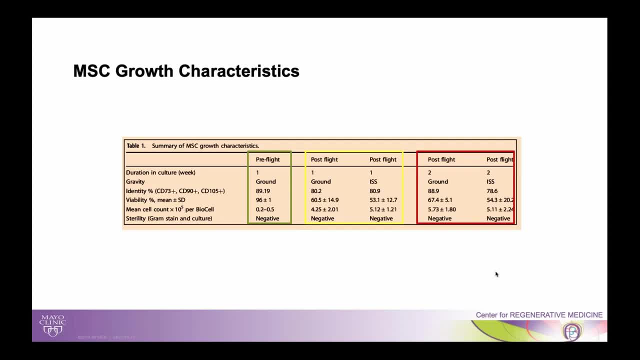 rate is comparable, And the same for the two weeks culture as well. The viability is a little bit worse, especially the ones at ISS, But again, we think that could be also related with the cryopreservation method. All of this is sterile, and that's very remarkable. We 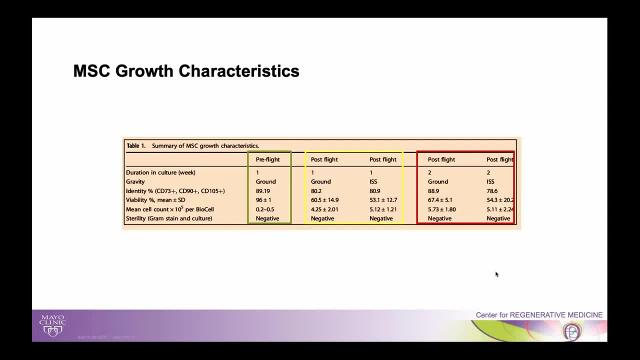 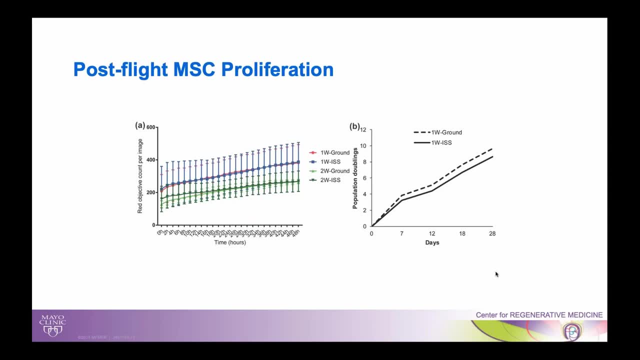 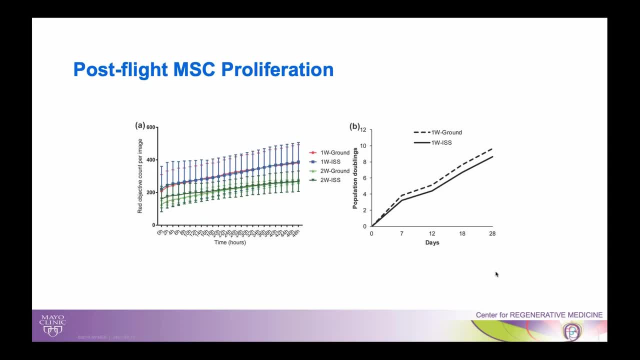 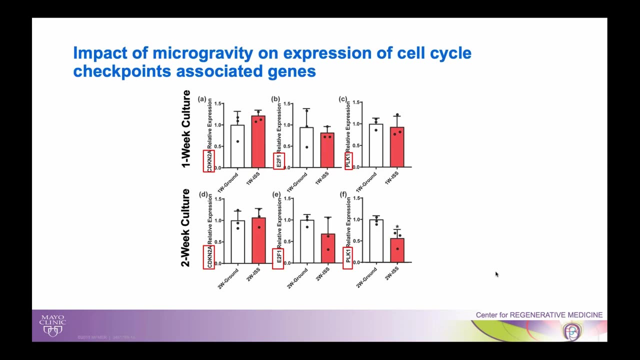 re-ativaing sensors. So now we are actually트묶 Jimmy time. The summary of it is that we didn't see any significant difference between control versus the cells that were expanded at ISS, So no impact really on chloroporation as far. 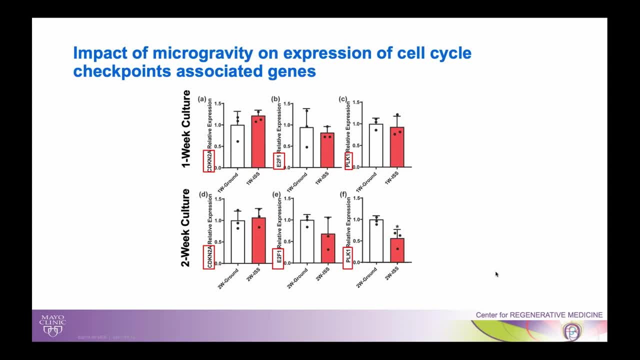 as we can tell. We also look at. of course we are talking about cell expansion, So we look at cell cycles and look for expression of cell cycle checkpoints inhibitors. So CDKLN2 is a cycle-independent kinase 2A which inhibits transition from 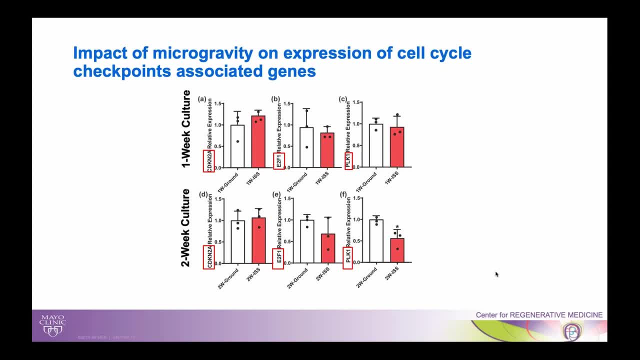 G1 to S phase. And then we also look at E2F1,, which interacts with IV retinoblastoma protein, which is a powerful cell cycle regulator, And then the folio-like kinase 1,, which is serine threonine kinase, which inhibits transition from G2 to M phase up-cell cycle. As you can, 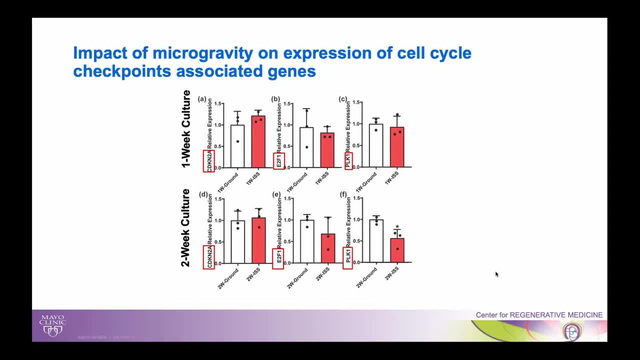 see at one-week culture, there is really no significant difference. So also in two-weeks culture other than the PLK1, a significantly decrease compared to the ground control- We really think more than ever that there is a significant difference between the two-weeks. 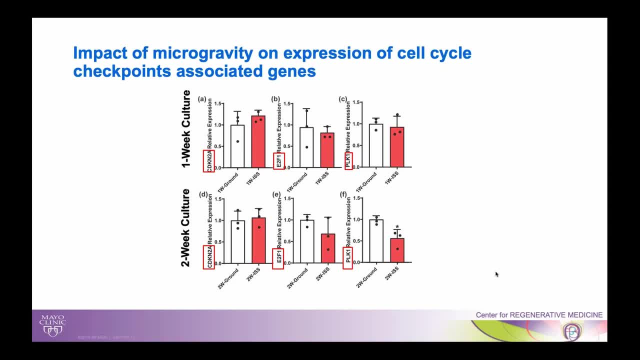 culture other than the PLK1, a significant decrease compared to the ground control. We again appreciate that more studies needs to be done. But now it looks like microgravity might be inhibiting the MSC expansion or progression in the cell cycle. But I think more studies 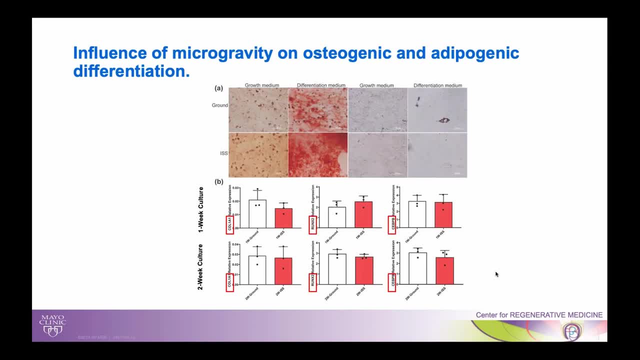 need to be done. And then we look at differentiation, both using Aliris, using stain for osteogenic differentiation and the oil red for adipogenic differentiation differentiation- The figure A on the top is just showing the normal cell grown in regular media and then the differentiation media. We also look at genes that are transcription factors, that are 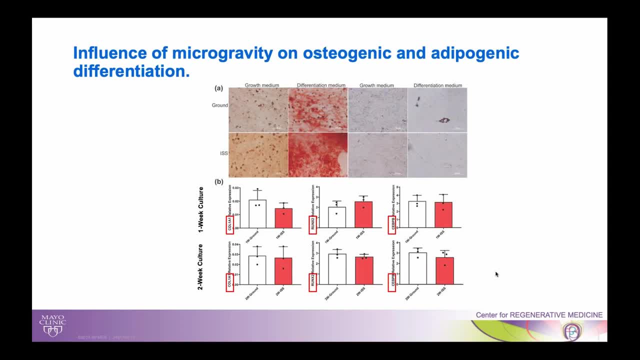 known to be associated with osteogenic differentiation, which is the first two, the CLK1A and the X2.. And then the crowd B is for adipose genetic differentiation, And the summary of it is that we haven't seen any difference between control and space-grown MSC in their 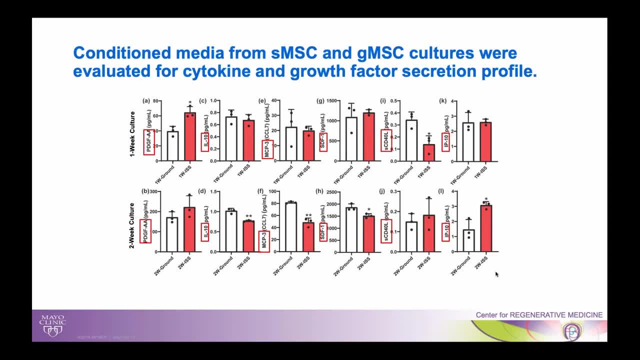 ability to differentiate. We also looked at condition media for cytokine release, looking at both ISS-grown and ground control, And the interesting thing is that we look at 65 different cytokines and we were only able to detect significant difference in two. There's SCD40 ligand. 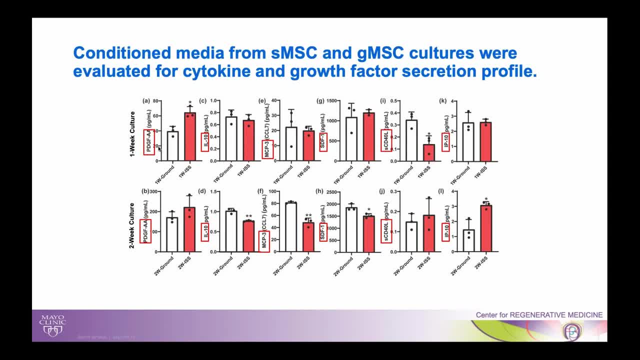 so, which is significantly decreased. And then the platelet growth factor is significantly increased after one week of culture, And the two of these are both thuraceae and the mother band hen Difusoridae, And although the défusoridae has reduced, 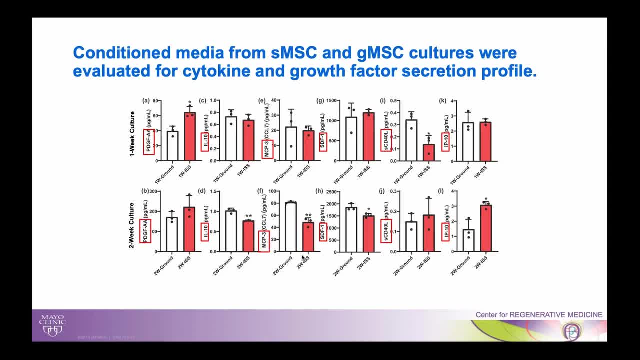 but we see more cytokines been affected After two weeks of culture, for example, the IL-10 is significantly decreased, MCP-3 also significantly decreased, So as the SDF, which is powerful chemokine, reported. So it's interesting to see our studies also confirm previous report And then also 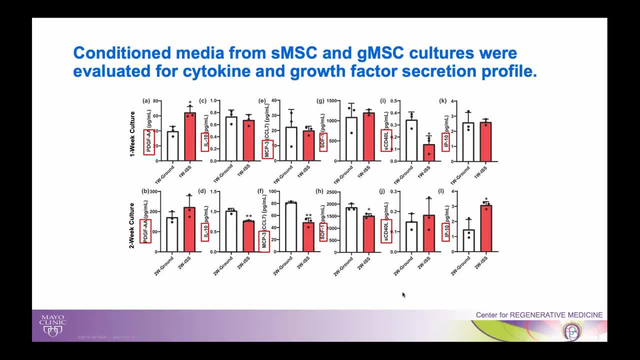 the IP10 is increased. I think again with this one, the conclusion you can only draw on this is that, yeah, cytokine and growth factor expression is impacted by the absence of gravity, but most studies would be needed to really comprehend the downstream effect. 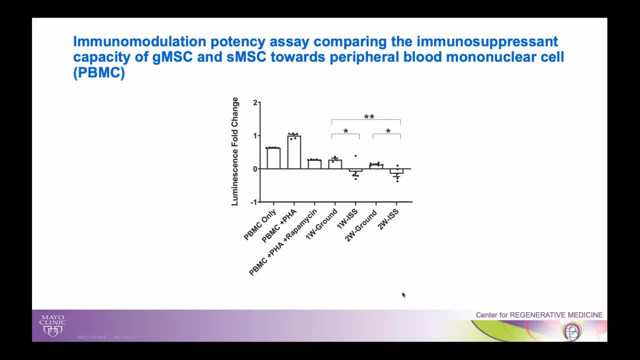 of these changes. We also look at potency assay. We wanted to see if the MSC are more immunosuppressant than when they were grown under microgravity condition. MSCs are known to be immunomodulatory And actually it's one of the primary reason that they have been used. So they are used. 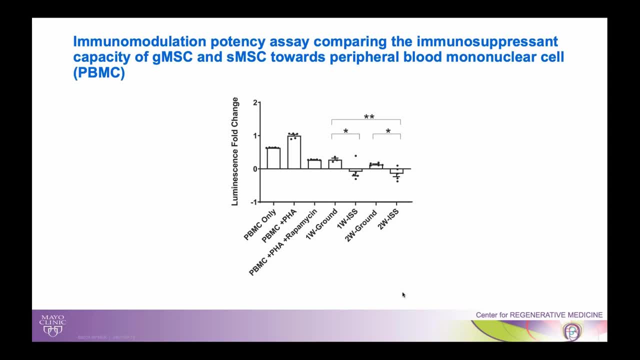 in treating rejection of organs also used in as immunosuppressant to control the graft versus host disease at carbomar or transplant. So we wanted to see whether that properties of theirs is maintained or enhanced or decreased, And the short answer is the, the, the, the. 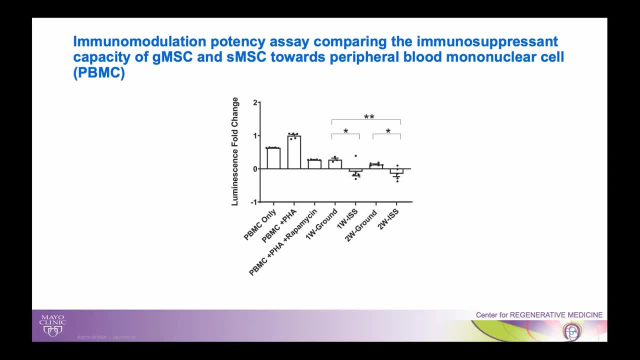 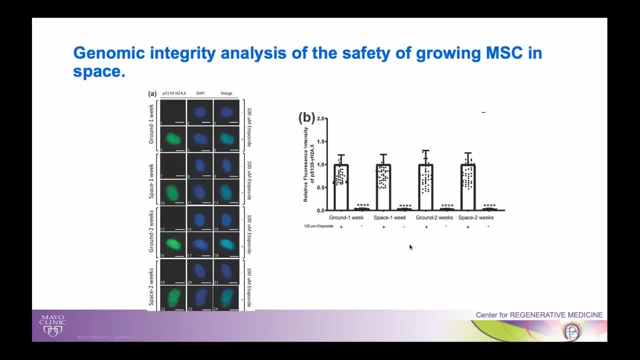 at one week and two weeks. Finally, we we come to safety. We are worried about DNA damage, So we use this marker. that is, this transcription factor is part of the histone family of transcription factors. They that get exposed if the DNA is damaged. 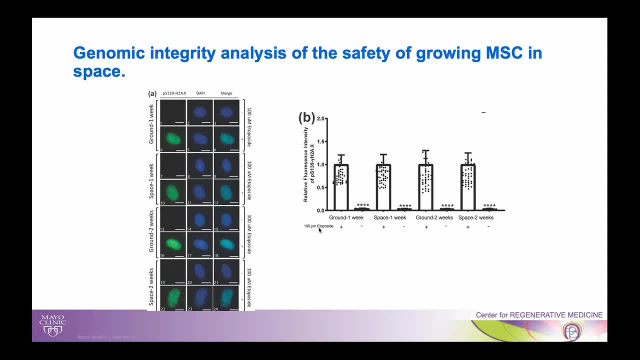 So we stain the cells and then we also expose the cells with etoposide, which has DNA damaging properties. as our positive control, We also use DAPI to stain the nucleus so that we wanted to show that the DNA damage is in the nucleus. 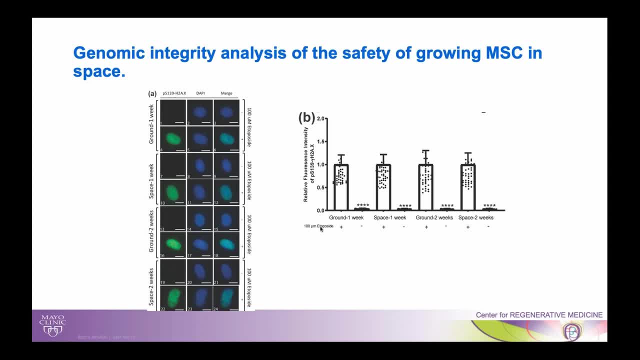 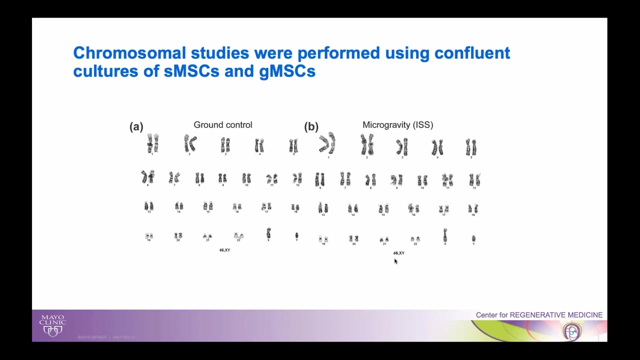 So basically you can see when the drug is used. you can see a lot of DNA damage and without the drug that is no damage. And we haven't seen difference between gram control and space for all the weeks of culture. We also did chromosomal studies and karyotyping. 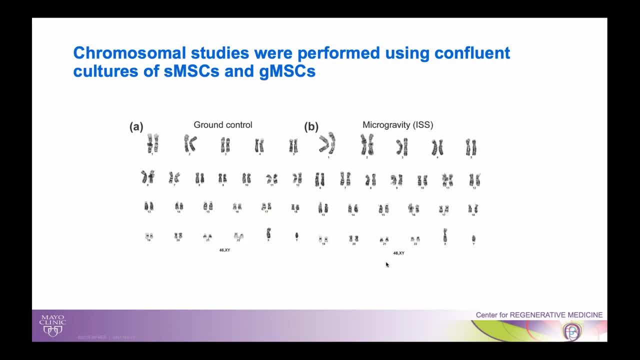 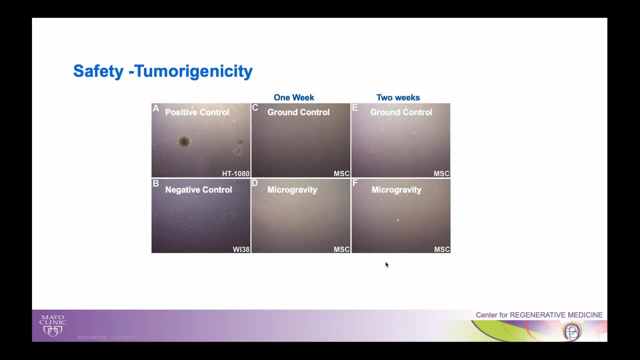 This is a gene banding And clearly we didn't see any chromosomal damage. We only saw some chromosomal abnormalities when we compare the gram control and the ISS. And then finally we said, well, what about tumor formation? So here, this is a positive control. 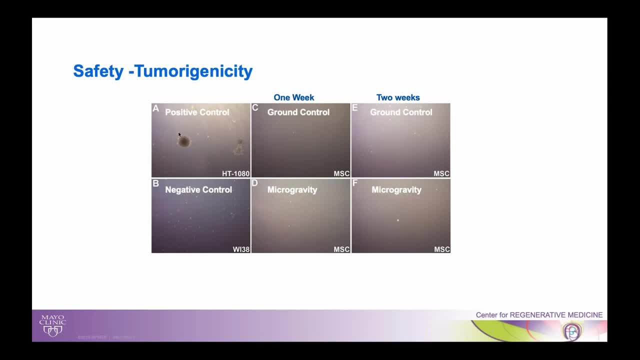 We're using a fibroblast for my cell line. You can see the colony being formed and this is what we are looking for. So, and then this is a negative control of just the cell. So we're looking for the cells that are different. 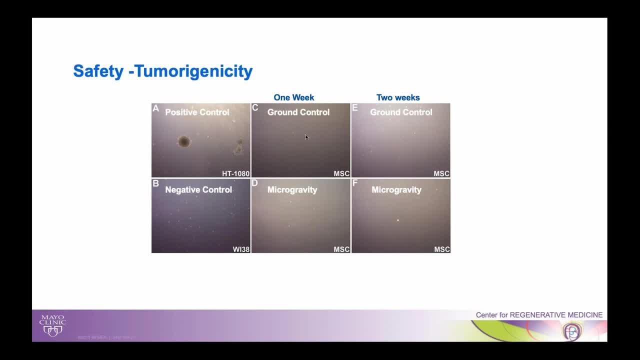 from the ones that are used in the control group. So you can see the ground in one week and then the microgravity ISS in one week and then in two weeks. Both there is no evidence of tumor formation like what we have seen in the positive control. 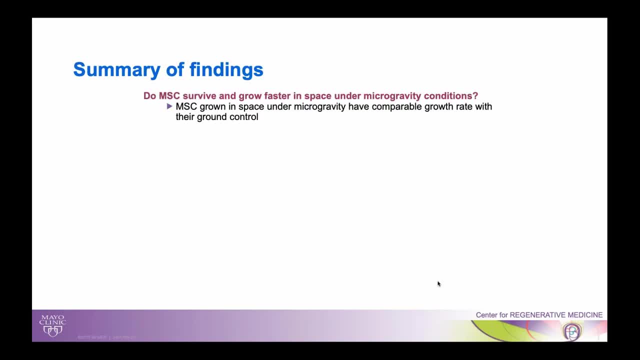 So the summary of our finding is that. so we asked fundamental question: do MSCs, do they have a good control? Do MSCs survive and grow faster in space under microgravity condition? And the short answer: yes, MSCs grow in space. 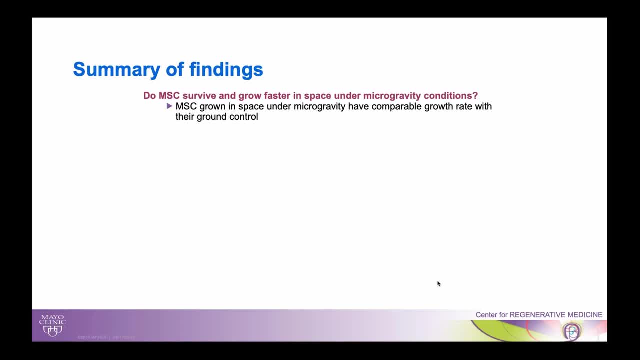 under microgravity condition and their growth is comparable to the one on the ground control. So we didn't see that further expansion where we can grow more cells, But these are the MSCs. We've seen some expansion on the HSC and there wouldn't be time. 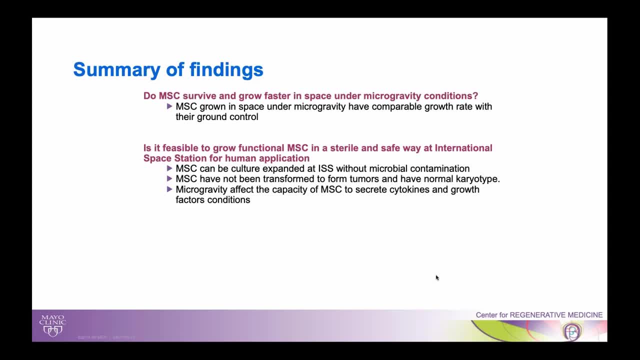 for me to go into that data more, to come down the road And then, in terms of feasibility, growing MSC in a sterile and safe way at the International Space Station. clearly we can see that we can do that. MSC can be cultured without any microbial contamination. 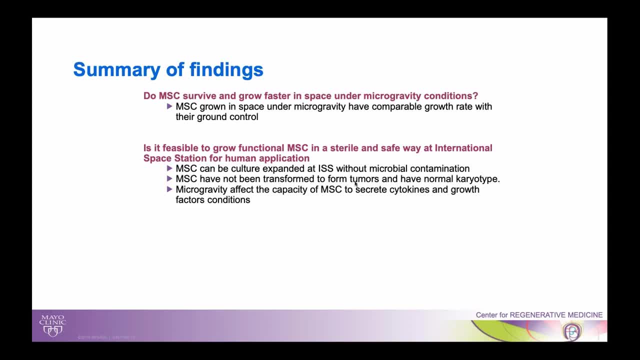 We show that they haven't been transformed to form tumors. They have normal chromosome. the karyotype is normal, no DNA damage seen. We also have seen that there is an effect of the microgravity on the MSC capacity to secrete some cytokine and growth factors. 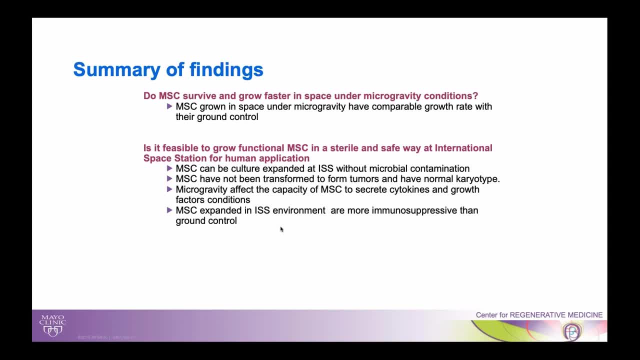 and that the MSC actually that they are more immunosuppressive compared to the ground control. So those are the main findings. Obviously, we have a lot more questions, So it's really nice to be given this opportunity And thank you so much. 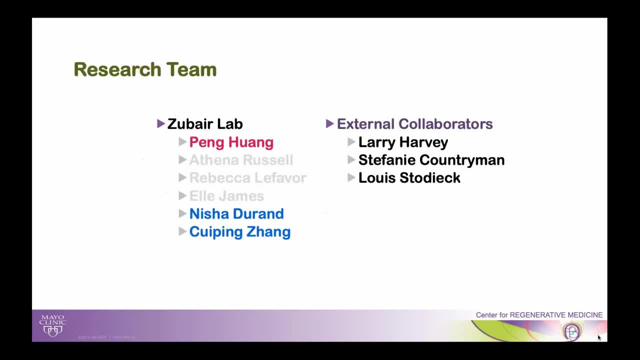 I will stop now, Thank you. Thank you, Dr Zubair. This was fascinating. Your results are very intriguing and looking forward to seeing more of them. I want to remind everybody that as you come up with questions, please enter them into the questions tab at the end. 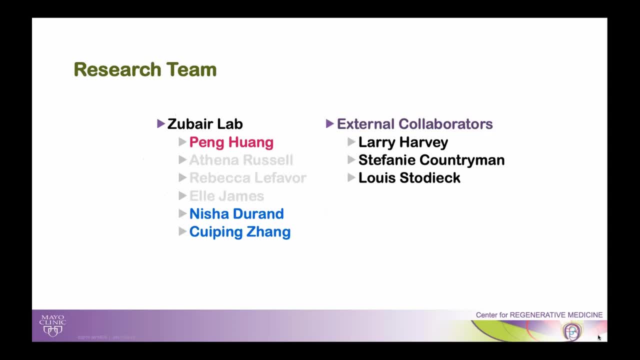 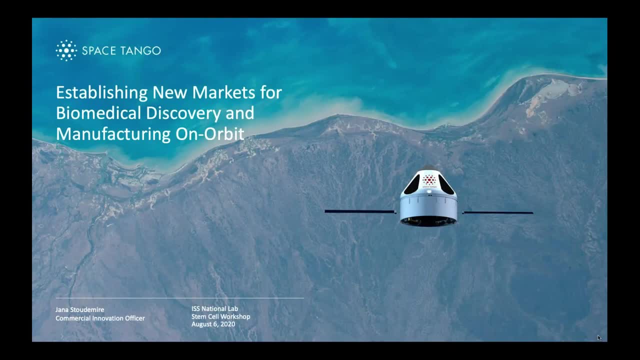 And during which we will have a panel session. we will start addressing the questions. Our next speaker is Jana Studemeier. As the commercial innovation officer at Space Tango, Jana Studemeier leads the commercial market creation for biomedical and technology manufacturing applications. 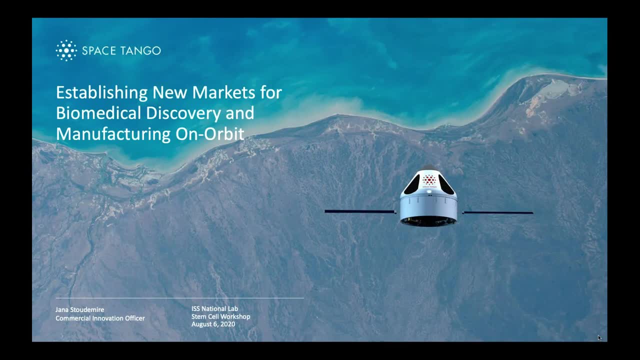 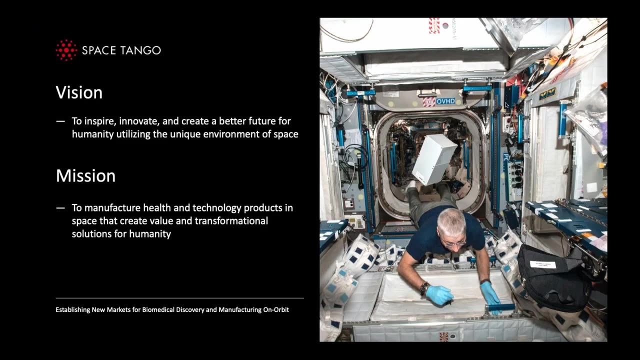 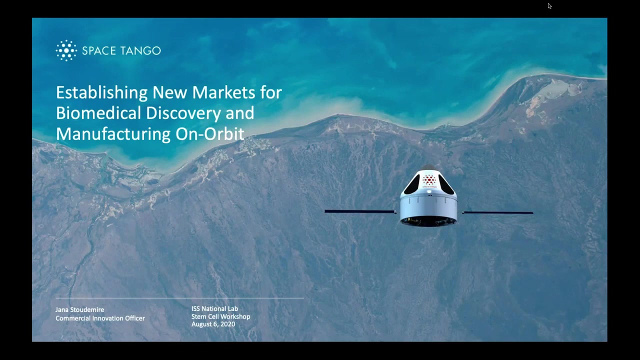 in low Earth orbit. Today you'll hear about Space Tango's work to expand capabilities and partnerships for stem cells, stem cell discovery and manufacturing applications in microgravity. Go ahead, Jana. Good morning Liz and good morning everyone. 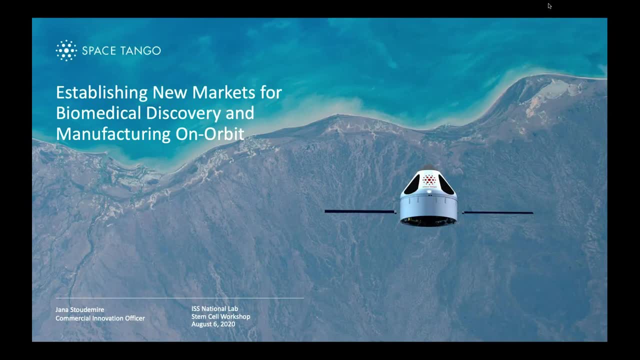 Thank you so much for this opportunity to present to the group today And thank you, Dr Zubair, for an excellent opening presentation. I'm looking forward to hearing more from Dr Sharma and from Dr Shepherd and Dr Lin later on from CIRM as well. 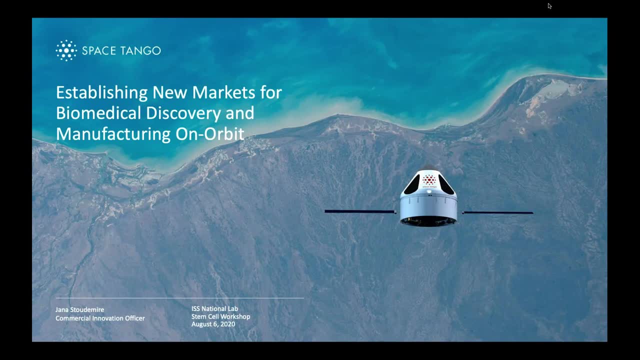 I want to start by just saying: you know, it's really an exciting time, both in space and on the ground, for regenerative medicine, And so I'm going to walk you through this morning a little bit of capabilities development that we're doing to support more sophisticated biology. 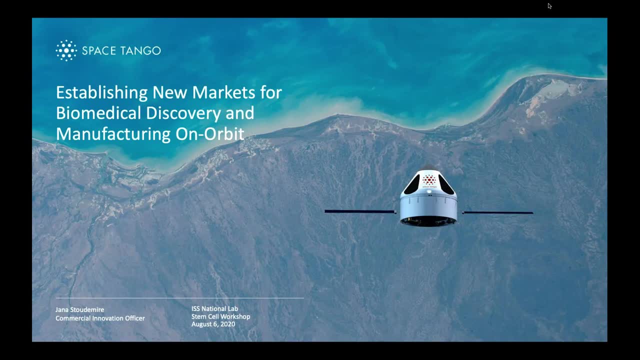 that really will help us to understand that regenerative medicine opportunity in microgravity, as well as some of the changes that are taking place on the space side that are helping us as well. So at Space Tango, our focus, as you probably know, 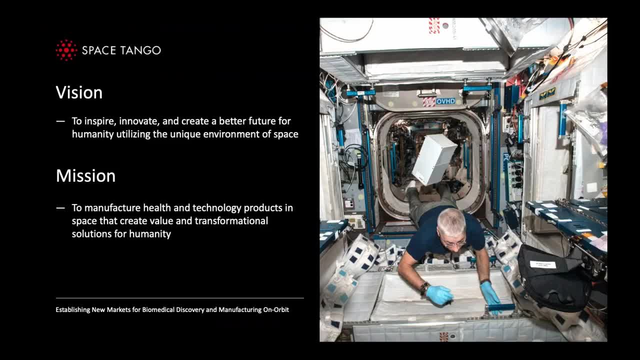 I think most of you are aware of the work that Space Tango is doing, but we're really looking to inspire, innovate and create a better future for humanity utilizing the unique environment of space, And our mission is really to manufacture health and technology products in space that create value. 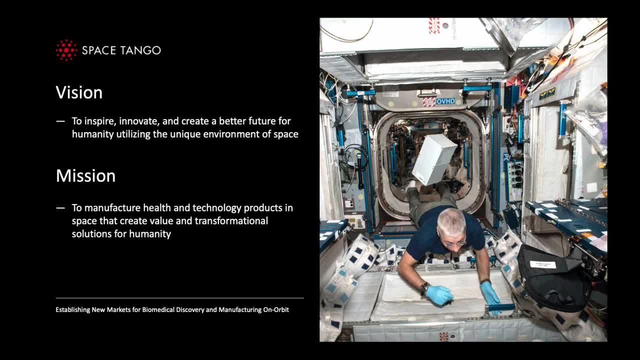 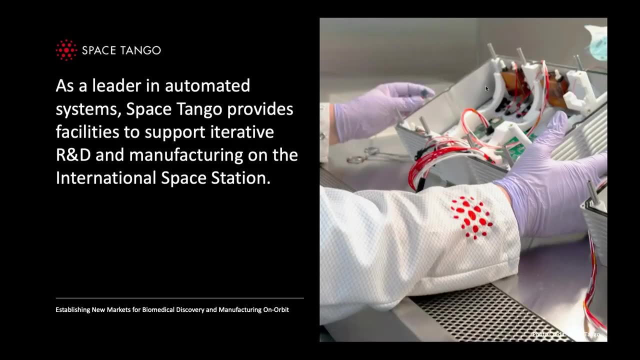 and transformational solutions for humanity. So we're very focused on opportunities to not only understand the fundamental science but to look at how we can build a robust commercial space economy that has a new market segment in it for biomedical products. In terms of the automated systems, 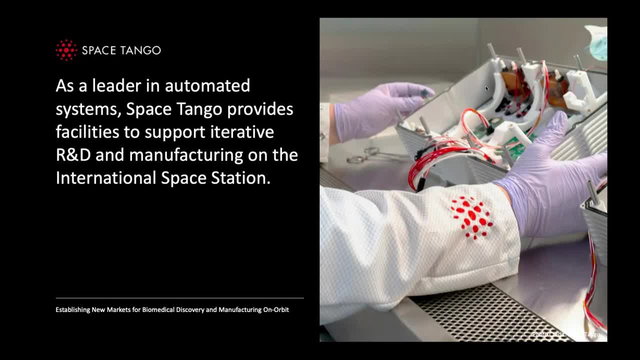 so we put together facilities that really support iterative R&D and manufacturing on the International Space Station, And part of the focus for us is to be looking at sort of you know, more than one opportunity to be able to understand some of the complicated biology. 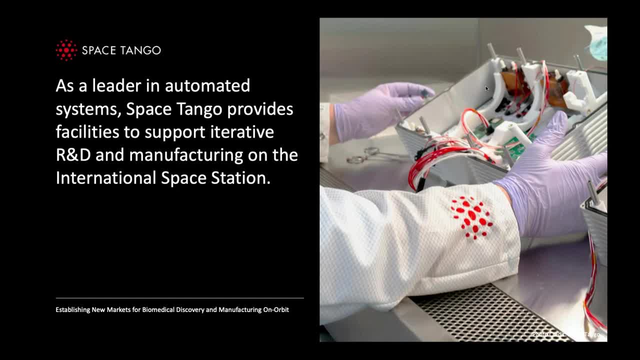 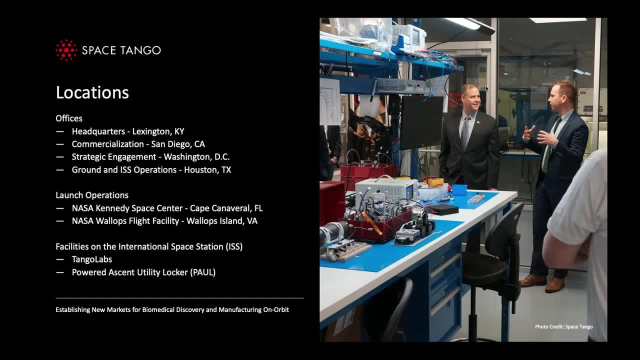 It's complicated on the ground and it's even more complicated to sort out in space, as you were just hearing from Dr Zubair. Just briefly, I think everyone probably knows we're located. our headquarters are in Lexington, Kentucky. 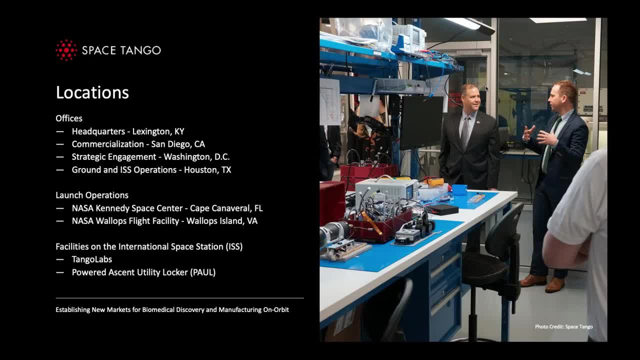 I'm actually based in San Diego, California. We have also part of our team in Washington DC for strategic engagement With our congressional representatives and we have ground operations in our Houston facility satellite facility in Houston, Texas. Launch operations are performed out of. 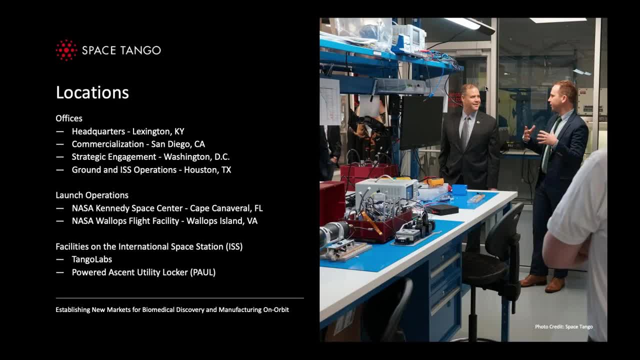 NASA Kennedy Space Center at Cape Canaveral and Wallops Flight Facility, Wallops Island, Virginia, And on ISS we actually have our two Tango Lab facilities and our Power Descent Utility Locker, which I'm gonna talk a little bit more about. 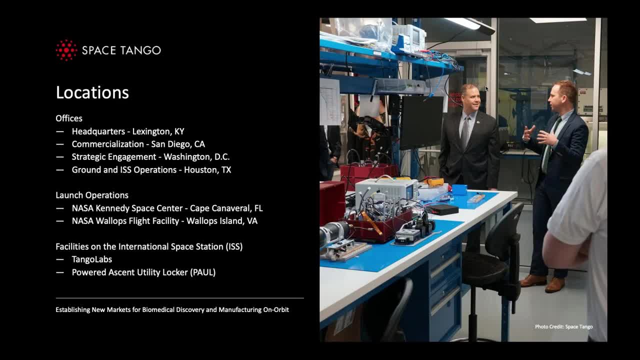 in this presentation, but it's a newer capability that has been developed by Space Tango to allow us to have power on ascent, so that we can actually maintain the biology as we transit to the International Space Station, as well as while we're on orbit. 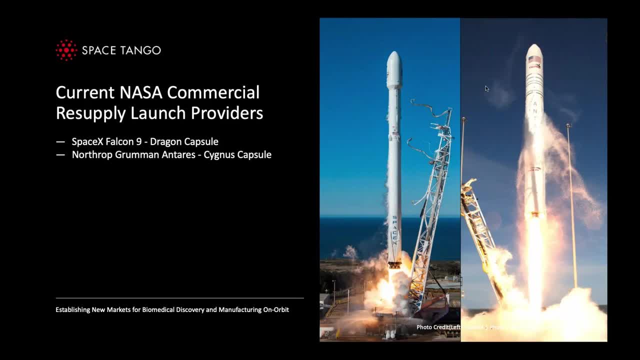 So you heard a little bit about rockets and I know that we talked that. Dr Zubair mentioned the splashdown Just for background here. for anyone who is not aware, there are three fighters for commercial resupply missions, which is where the science that goes up actually flies in. 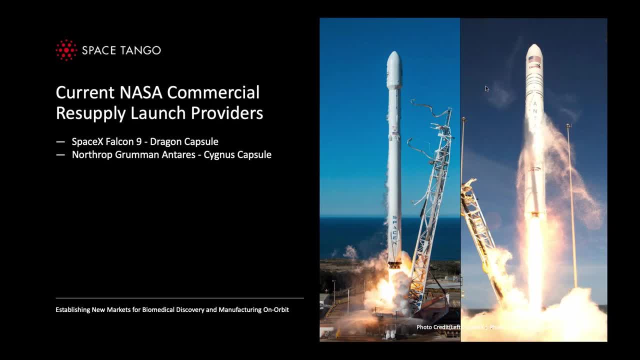 One is SpaceX, the Falcon 9 and the Dragon capsule, which everyone, I think, has seen quite recently, even with American astronauts on American rockets from American soil, which is fantastic. and Northrop Grumman also has the Cygnus capsule. 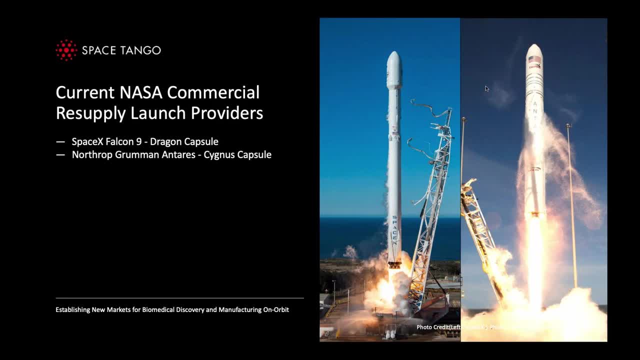 the Antares rocket and the Cygnus capsule. Just a little bit of background here for anyone who is not familiar with these vehicles. and space Dragon capsule is the only one that returns back to Earth with samples in it. The Cygnus vehicle. 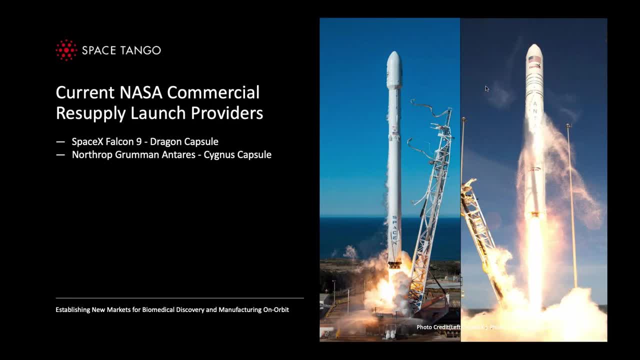 goes to the ISS, delivers science and supplies, but actually is the trash vehicle that is designed to burn up on re-entry. So when we talk about biological payloads- and you know Dr Zubi mentioned SpaceX- is really the only capsule where those samples can return. So often we try. 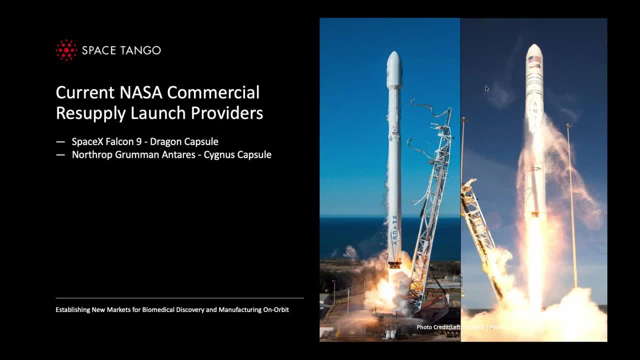 to fly biological payloads on a SpaceX mission because they can go up and back in the same vehicle. You can actually go up on a Cygnus vehicle and come back on a Dragon, but there's a little bit of time between those launches and so the sensitivity of these payloads. 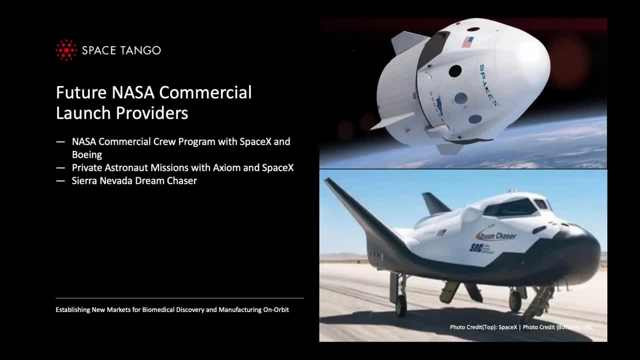 we try as much as we can to put them in the same mission. The exciting part of what's happening on the space side is that, in addition to those two vehicles, we are now having new vehicles come online and new opportunities for flights. So where it's been. 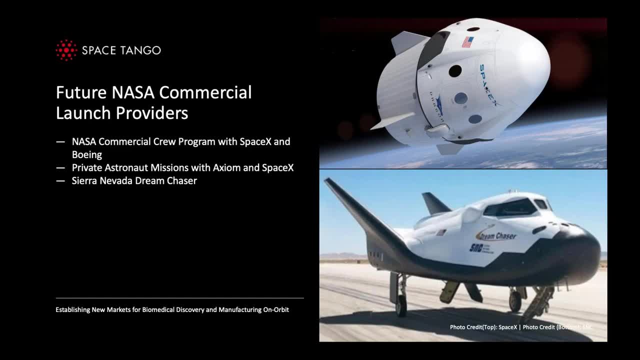 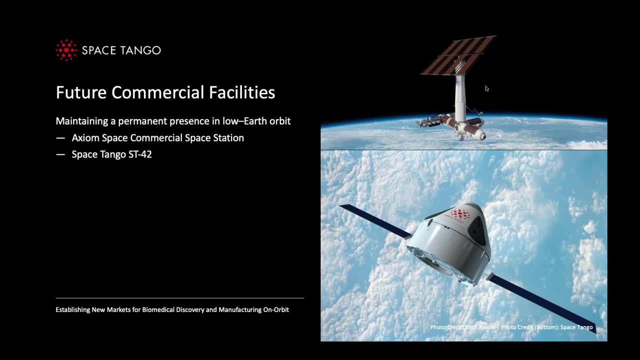 difficult and sometimes a long time frame to be able to get to an opportunity for launch these additional vehicles and providers will be able to give us an opportunity to really have the increased access that we need. There's also some future commercial facilities that are being 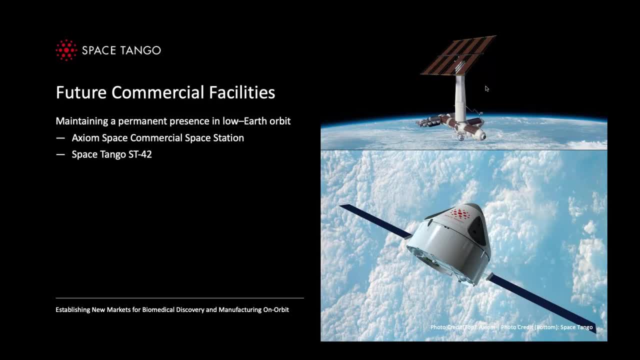 developed. so ISS? as everyone knows, this is the 20th anniversary year. It's been in orbit for quite a while as a laboratory, but recently NASA actually awarded the docking port to Axiom Space for a commercial space station that will be used to really maintain. 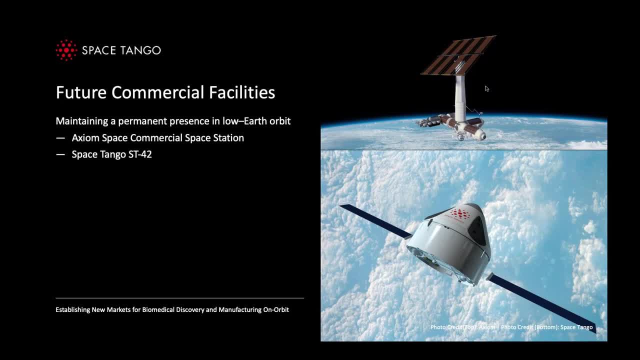 our presence in low Earth orbit once the ISS is decommissioned. Space Tango is actually working also on our own free flyer, an automated facility that we will be able to use for manufacturing on orbit of both technology and biomedical products, And it will give us the ability to 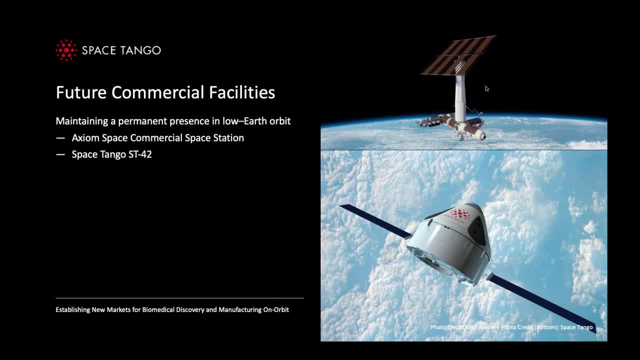 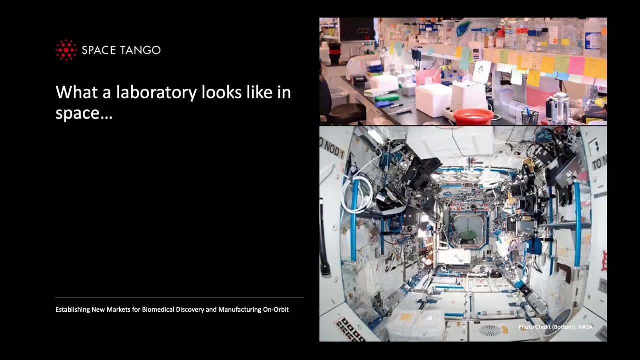 really be on a schedule that we'll be orbiting, we won't be docking, there won't be people on there, so we can kind of control the time frames of up and back micrograph. So that's a little bit about capabilities and it's good to see the increased access, but I want 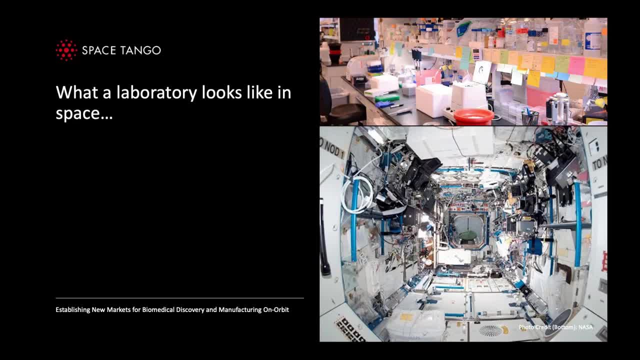 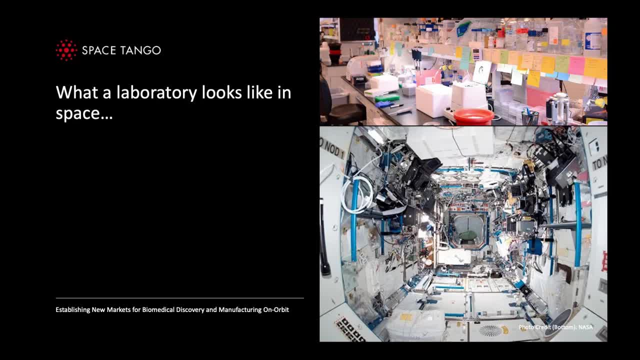 So I thought I would start first with just sort of the basic overview for an understanding of what a lab actually looks like in space. On the top here you see your typical lab bench with everything out on it and lots of bottles and reagents and all kinds of equipment. On the bottom you see the 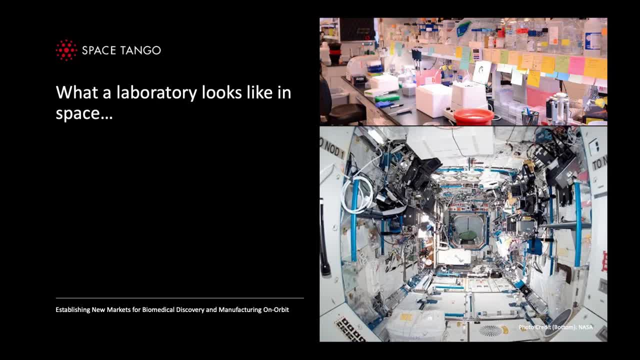 inside of the ISS, Everything is bolted to a wall or put into a locker format, obviously so that it doesn't float away, And it's a little bit more complex than what we're used to seeing in space, and this really is one of the big differences about working in space versus working on the. 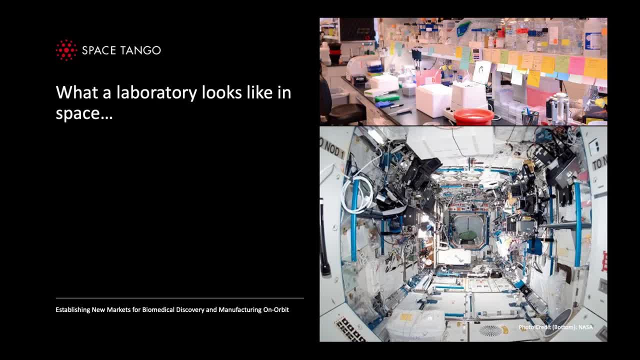 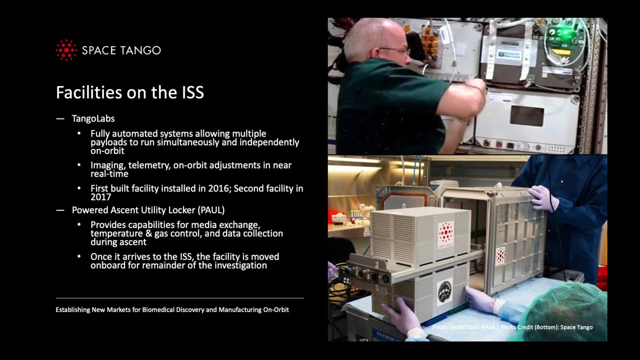 ground. Simple things that you would do in the laboratory, like a media exchange that would take maybe 45 minutes in space manually takes several hours, So it's really a very different process. Our facilities on ISS. we have two Tango Lab facilities, as I mentioned. The first one was 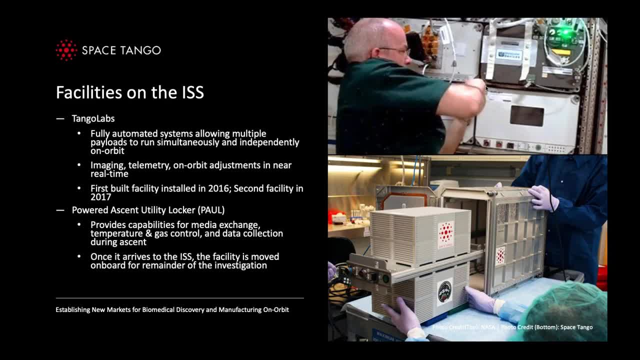 actually installed in the Tango Lab facility, and the second one was actually installed in the ISS facility in 2016, and the second facility was actually put up in 2017.. So these facilities give us the ability to collect data from payloads that are automated and remotely control those. 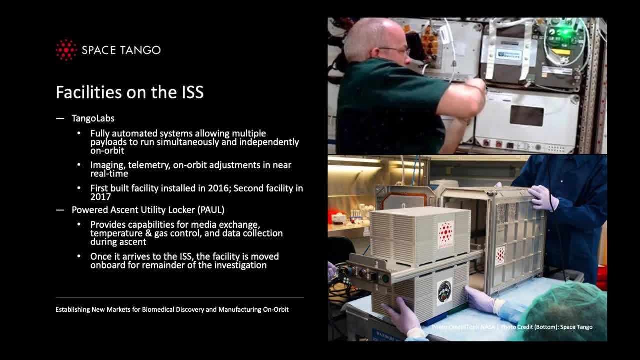 payloads from the ground. It removes the astronaut hands and time. that is very expensive and can at times be difficult to manage. The crew's schedule, as you may be aware, is very busy while they're on ISS. Not only the research that they're doing, but the work that 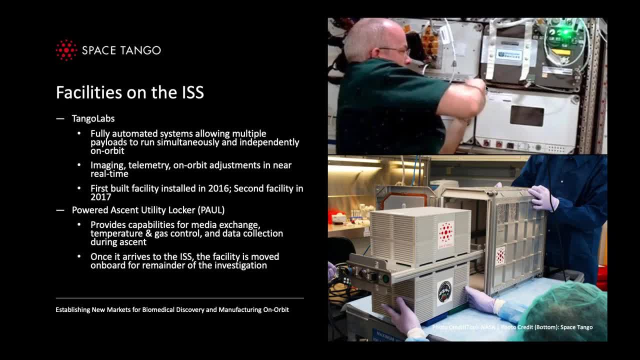 they're doing on station and the exercise that they need to do just to maintain their own physiology. So when we think about ways that we can help to accelerate that science, automating it and taking astronaut hands out of the process is something that we see can really help. 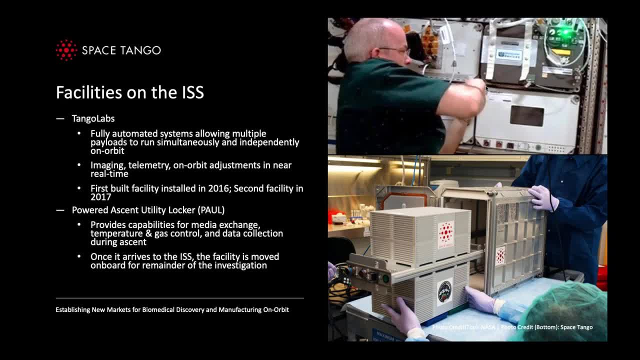 The Power Descent Utility Locker which is shown in the bottom picture. here is the locker that I mentioned at the beginning, that we created to help us on ascent really control the conditions that you need to maintain cell culture on the way to the ISS And once this facility is installed. 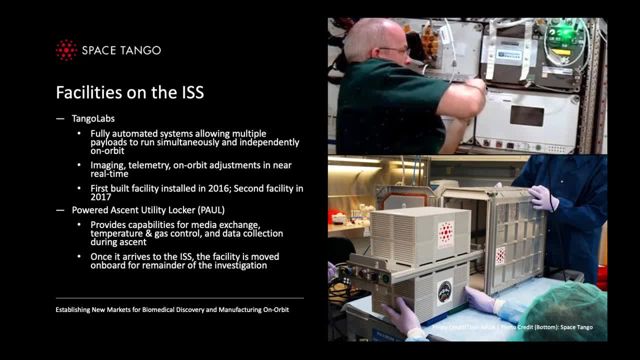 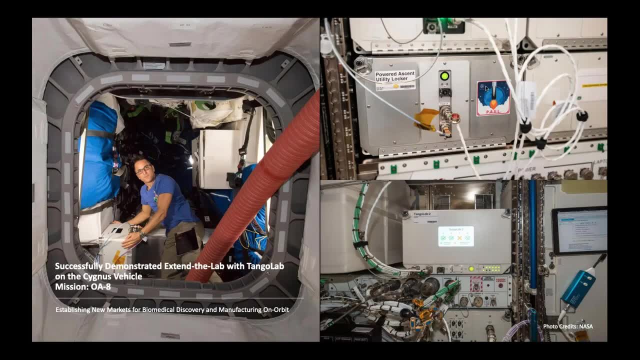 on board we can downlink the data that we retrieved during the ascent of the vehicle and actually continue the experiment. Just a brief mention here of the facilities and sort of the flexibility. The Power Descent Utility Locker is a very, very complex facility. It's a very 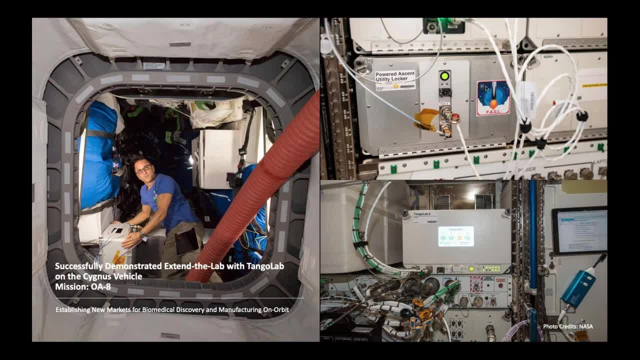 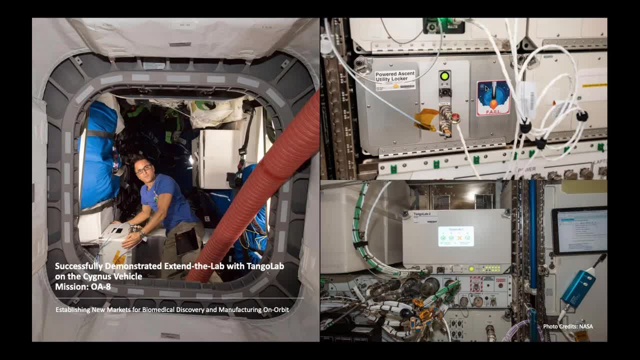 capsule, the Cygnus capsule, while it was docked to the International Space Station, really showing that we can kind of extend the laboratory that exists. Space is at a premium on ISS, as you can tell from the pictures, when you see everything. every space is used. So to have the opportunity. 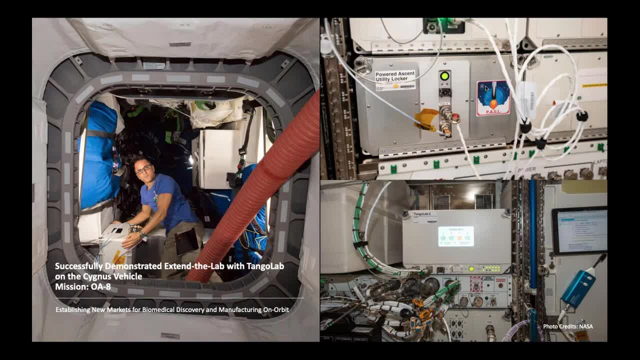 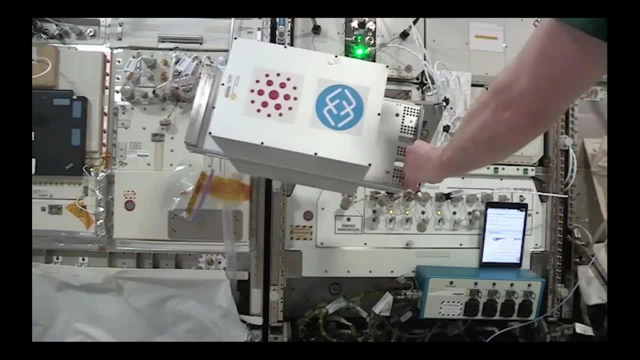 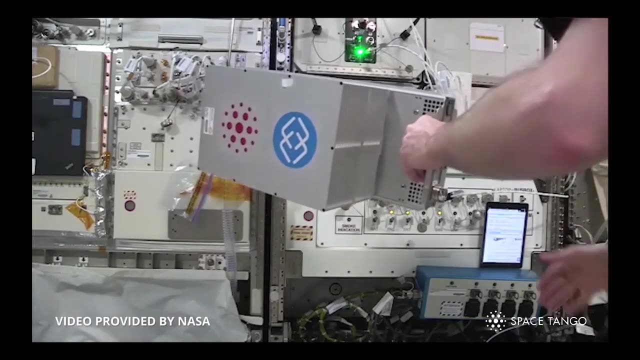 to be able to extend the laboratory, to be able to extend the laboratory, to be able to extend our facilities to a vehicle that's docked to station also increases our capability. This is just a short video of what the actual uninstall. These are two of our CubeLab automated. 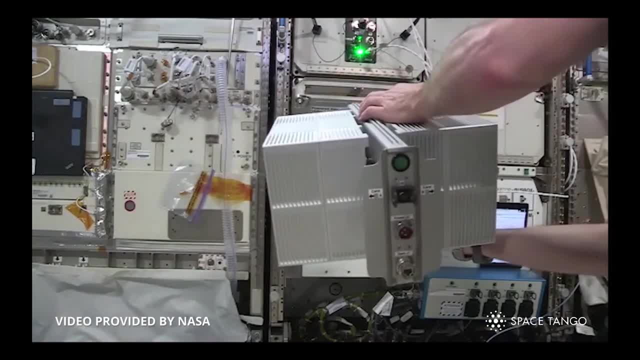 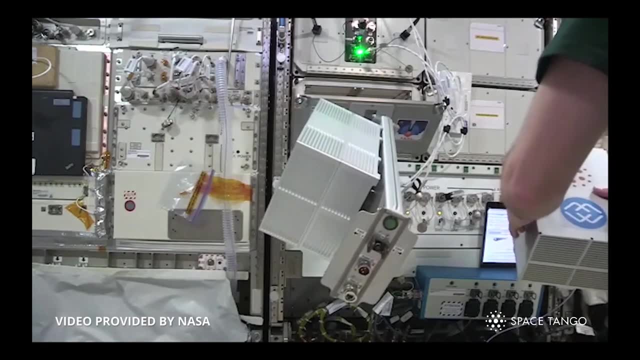 facilities- which I'll give you a little more detail on in just a minute- that are being removed from that Paul facility and put into cold storage. So each of these CubeLabs contain this is one of our tissue check payloads for the NIH. 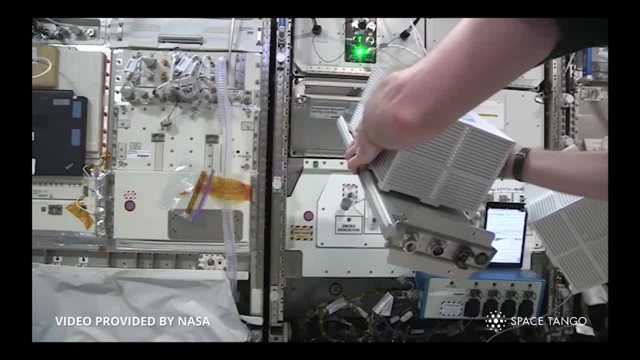 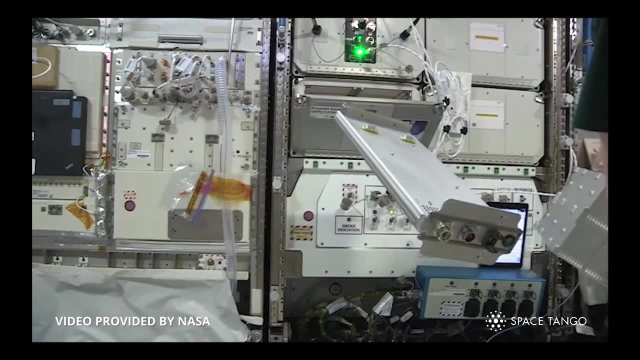 So each of these CubeLabs contain- this is one of our tissue check payloads for the NIH- And each of these CubeLabs contain science that has been now conducted, you know, cell long duration, cell culture on station and now being moved into cold storage for return. 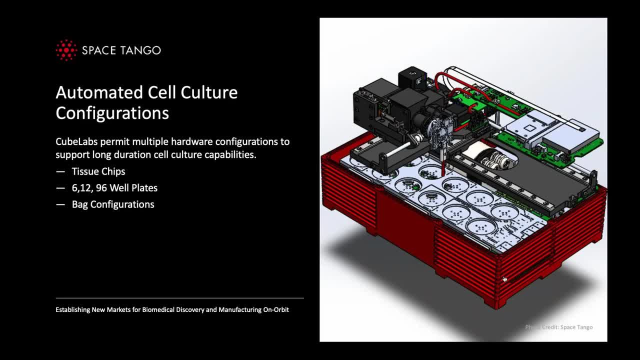 So a little bit about what's inside the CubeLabs And, as I mentioned before, you know the automation for us is something that we understand. to be able to support the sophisticated biology that is now a focus of regenerative medicine, We really need to have systems that allow us to look at different 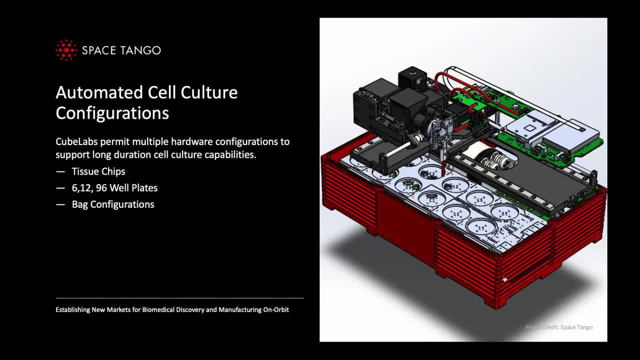 configurations of cells that can be grown in an automated way. So the CubeLabs that we've designed are they permit long duration cell culture for things like tissue chips. We have six, 12, and 96 well plate configurations as well as bag configurations, And we've added to the CubeLab an automated 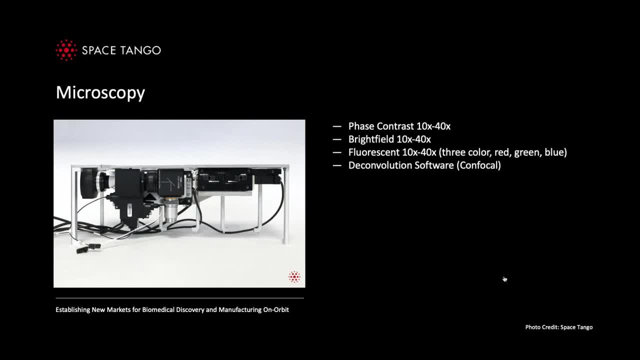 microscopy system. This is a great group from San Diego and I have to sort of give a shout out to San Diego because they are local, But Edeluma is a company that we see actually have optics from Edeluma. It's a perfect scope for ISS because of the fact that it is not only very compact and can 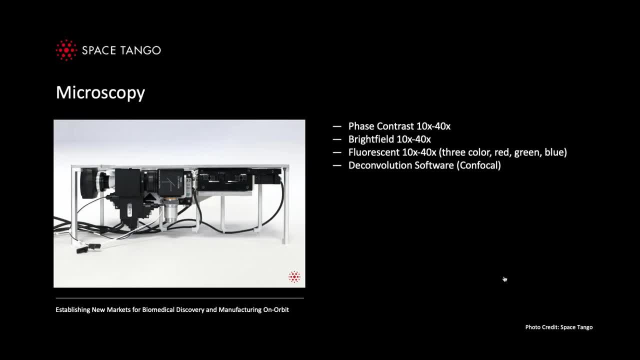 fit into the CubeLab, but it also has a unique vibration resistance, And so we're really excited about the future of the CubeLab. And so we're really excited about the future of the CubeLab. And so we're really excited about the future of the CubeLab, And so we're really excited about the. 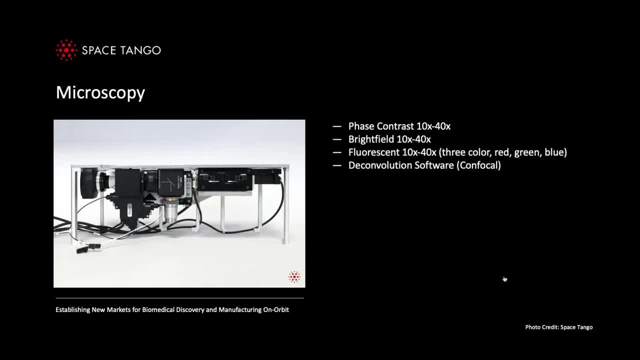 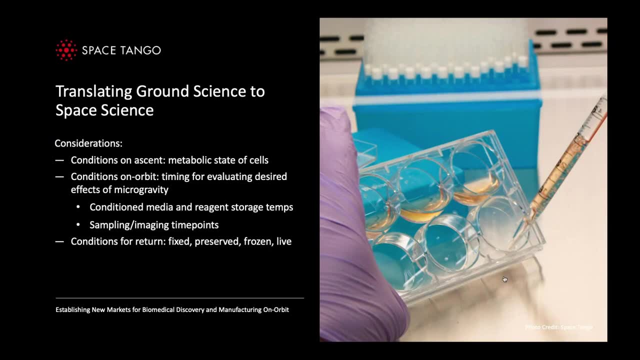 increasing capabilities to do on-orbit measurements with a scope like this in an automated way. So let's talk a little bit about translating ground science to space science. And you know, when I talk to the teams that we work with, I always talk about the fact that 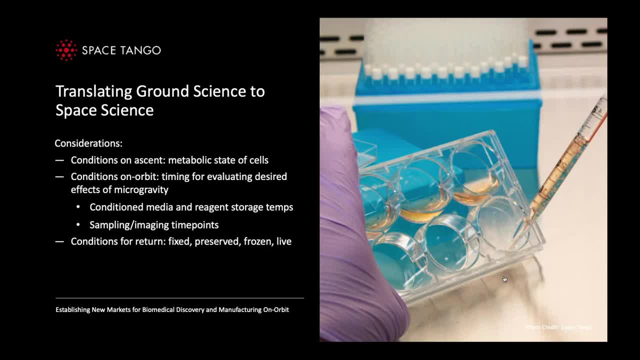 it's not really just the translation of ground science to space science. In our case, it's the translation of ground science to automation and then to space science, And there's lots of things that we need to think about. So the conditions on ascent, for example. 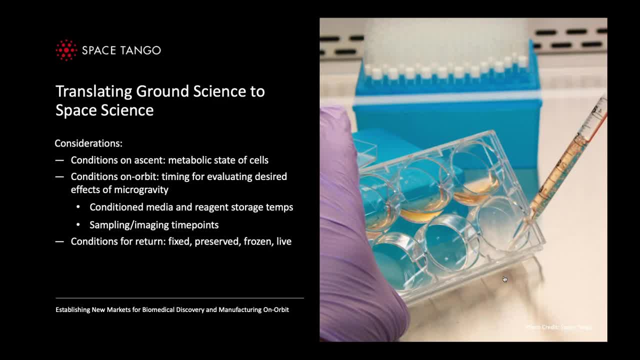 what's the metabolic state of your cells and how do you want them to arrive at the ISS, so that you can really make sure that the data that you're capturing is data from a microgravity environment, The conditions on orbit, the timing for evaluating the desired effects of 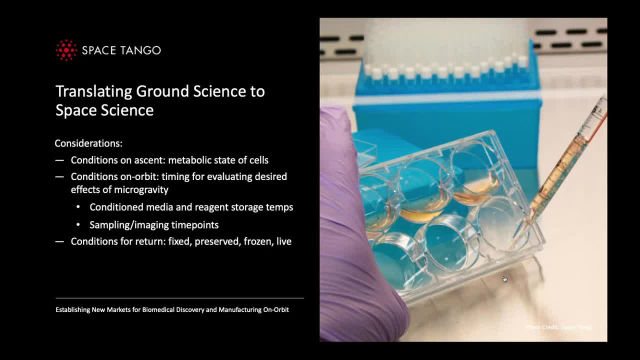 microgravity that you're looking for. So media samples and reagent storage. you know temperature- temperatures that need to be maintained for conditioned media that has growth factors in them within the same automated system as an incubator that keeps the temperature of the cells at 37. 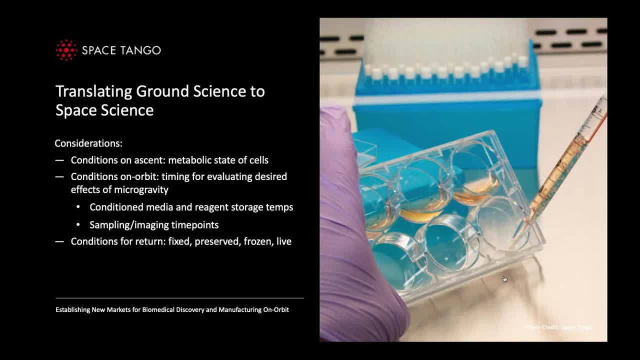 degrees, And then, of course, the sampling and imaging time points and how we can download that data and look at that during the course of the cell culture that goes on on orbit, so that we're able to make any adjustments that might be needed in near real time. And then the return of your 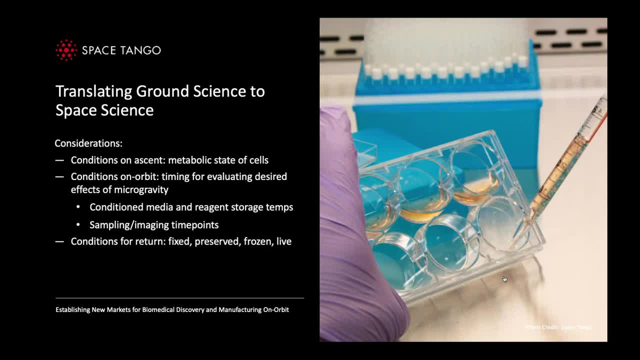 cells So fixed and preserved, frozen live. those are all capabilities that we have And in conjunction with doing on orbit measurements, you know, we want to make sure that we bring back cells that allow some additional post-flight analysis as well. 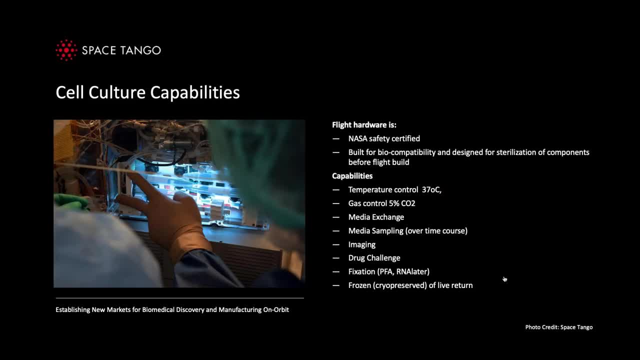 In terms of the cell culture capabilities that the automated hardware we're developing is designed to provide. So NASA Safety Certified. obviously, the systems that go up on ISS are at least two levels of containment. They're all built for biocompatibility and designed for. 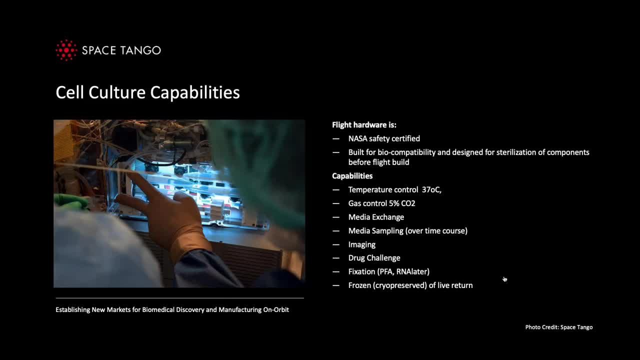 sterilization of the components before the flight build. They have the ability to control temperatures. standard conditions for cell culture: 37 degrees, 5% CO2,. do automated media exchange, media sampling over a time course, imaging drug challenge- if that's something that 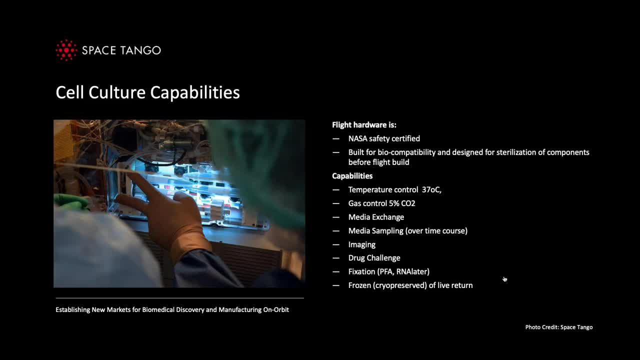 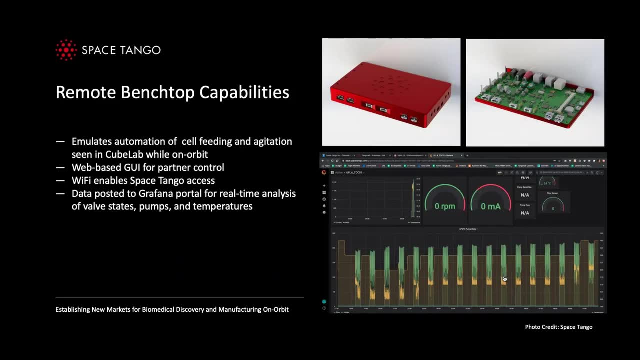 you want to look at as well, And then, obviously, the things that you're able to control, like the fixation and cryopreservation or live return of cells. We've also, because of COVID-19, developed some additional benchtop capabilities. 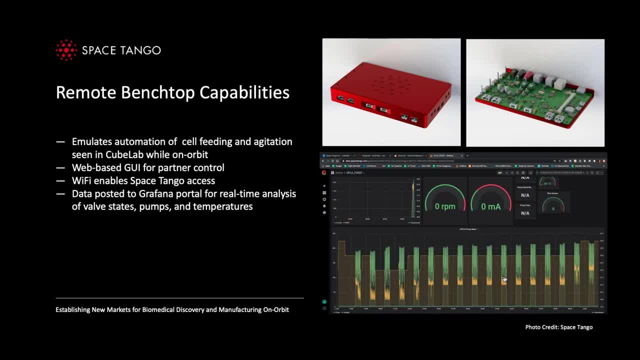 Everybody knows it's a little bit difficult to be in the lab right now- and those that are in the lab you know- for us to be able to visit and sort of be right there with some of the scientists. that's been a little challenging under the current travel restrictions as well. 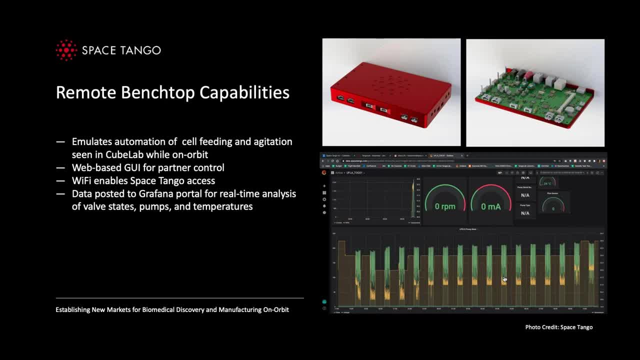 So what we've done is put together a benchtop capability that really allows the basic sort of self-feeding and agitation that you would see within the cube lab while it's on orbit, to be remotely controlled from the ground. So we have a web-based GUI for our partners to control and for us to control from Space. 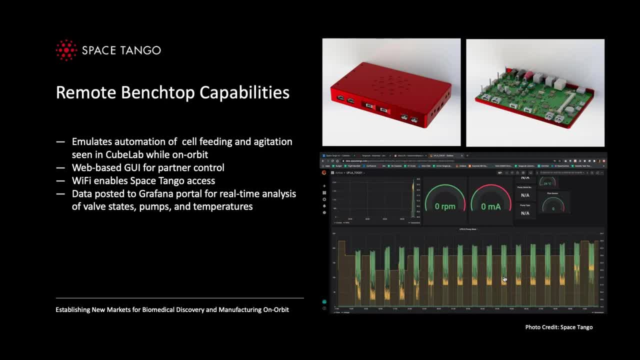 Tango at our remote access points And we have data that we can pull from that and put into a portal that we're able to share with the researchers. and we can all watch as we're working through the validation of these systems to make sure that they're working the way they need to. 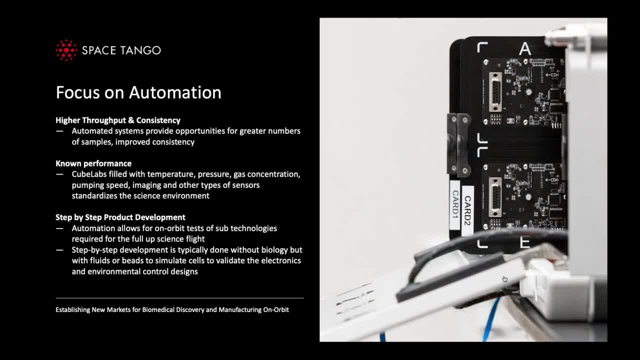 So the focus on automation. for us, there's a lot of reasons why. you know, in addition to the fact that astronaut time is expensive and sometimes difficult, you know, to make a change on a near real time is often a little tricky and challenging. 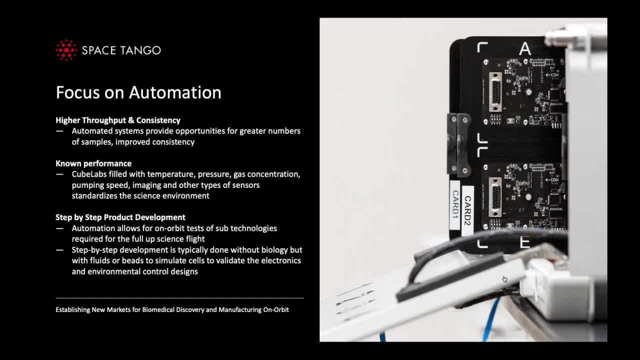 And that's because the crew schedules are so full, but also for the consistency. You know, we're very lucky to have people like Peggy Whitson, and you're going to hear from Dr Sharma next. I think about the work that was done by Kate Rubins, which is phenomenal. 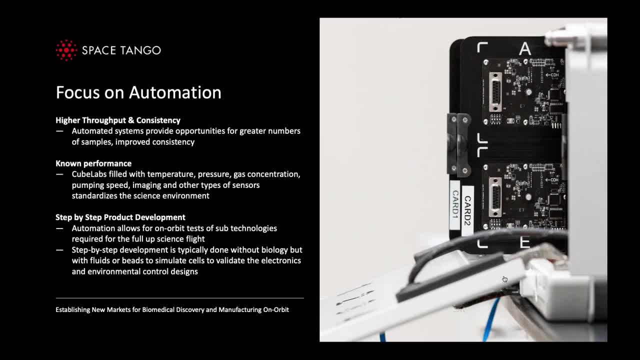 And someone like Kate Rubins is an amazing biologist here on the ground, But not every astronaut that is on station is Peggy Whitson or Kate Rubins, And so we feel like the automated systems not only give us the ability to control the space, the ability to have higher throughput, but also the improved consistency. 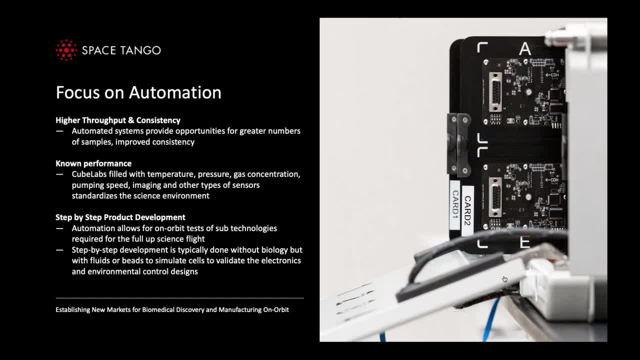 And we really focus a lot on making sure that those cube labs really have temperature pressure, gas concentration, pumping speed, imaging and other types of sensors that standardize the science environment. We take a step-by-step approach to project development. The automation allows for on-orbit tests of technologies. 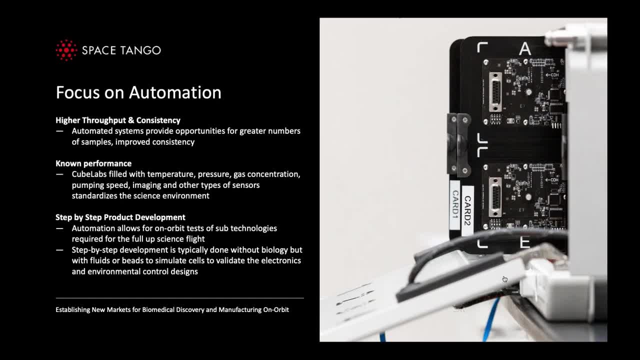 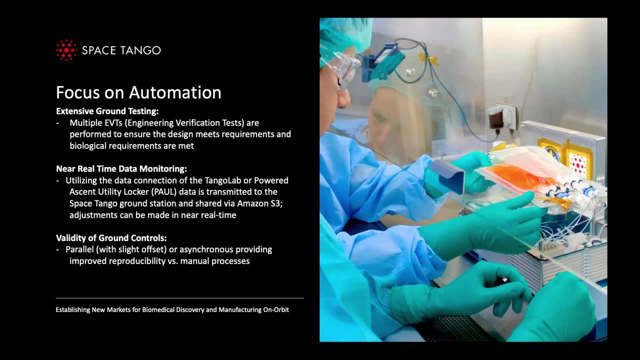 So We will look at each piece of the different part of the payload that's going to be automated, And sometimes we actually even look at that in a microgravity environment with things like beads or other ways to simulate, before we actually put cells in and fly it. 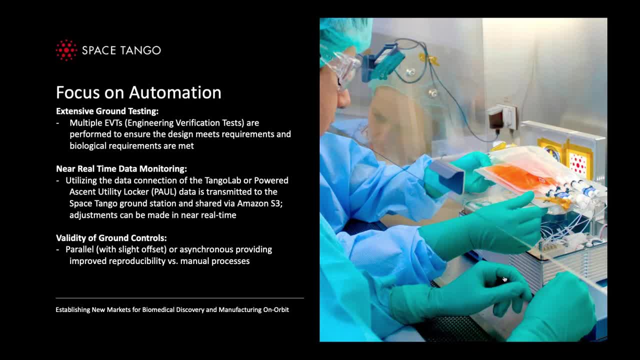 There's never enough testing that can be done on the ground to get ready for these types of experiments. The translation, as I mentioned, from bench to automation- So Bench to automation- really does require that we grow the cells in the system and make sure. 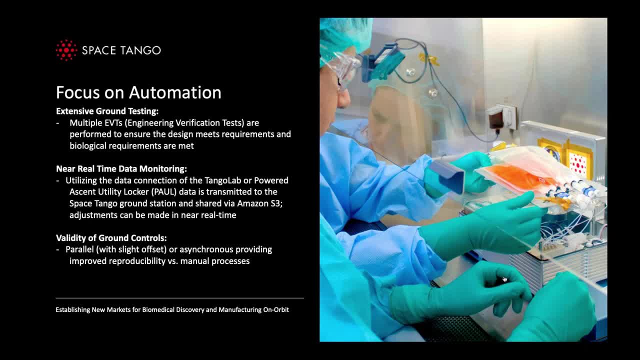 that not only the engineering design meets the requirements, but that the biological requirements are met as well, And the ability for the near real-time data monitoring that I mentioned. you know, downlinking data to our remote station allows us to have the ability to even do things like make changes. 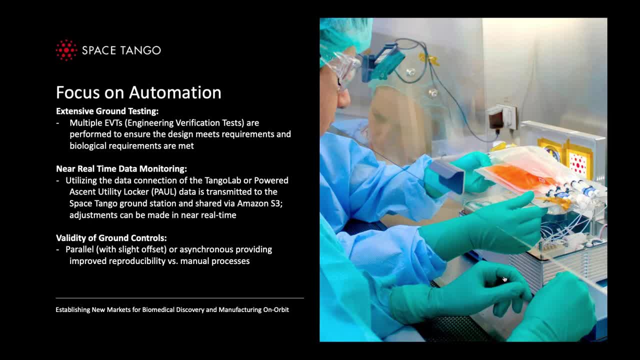 to the ground controls. So We have Options When we're doing either parallel controls with a slight offset, so that we can pull that data from what's happening on orbit and make adjustments if we need to, or at times some payloads- actually an asynchronous control, you know- done after the work is done on station. 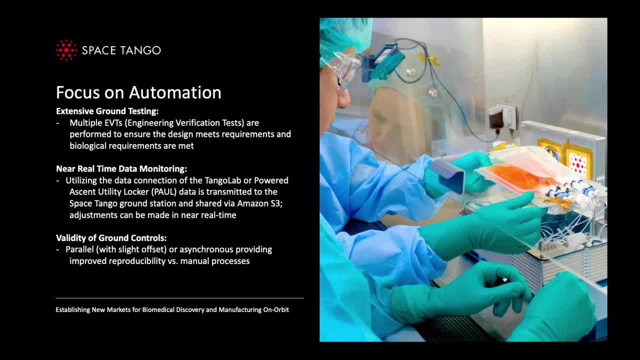 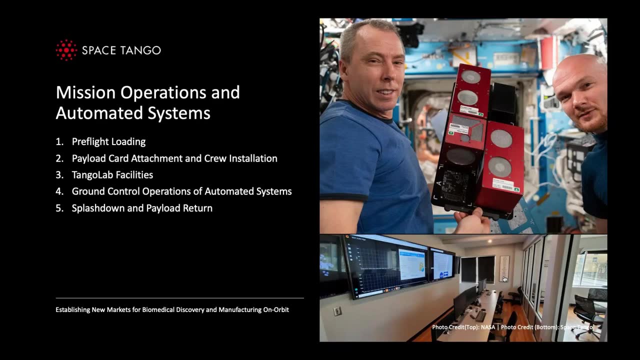 to match those conditions exactly. you know makes sense Most of the biological payloads. obviously you want to load them with the same cells that you're flying so that you limit the variability there. but there are opportunities to look at controls kind of from both perspectives. 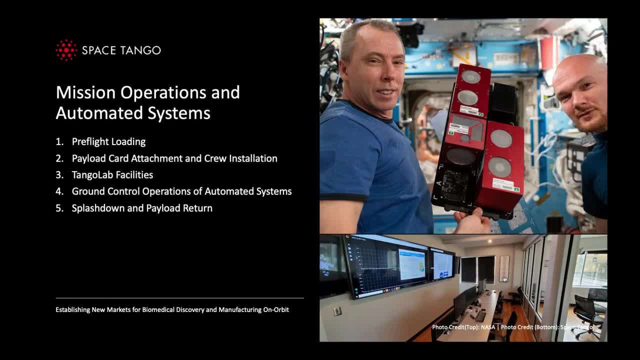 So now you know a little bit about what it's, what the hardware looks like, What happens when we actually now have tested the system and are ready to fly. We have pre-flight loading that goes on at Kennedy space center, So most of our teams will come down and be with us for several days before the launch. 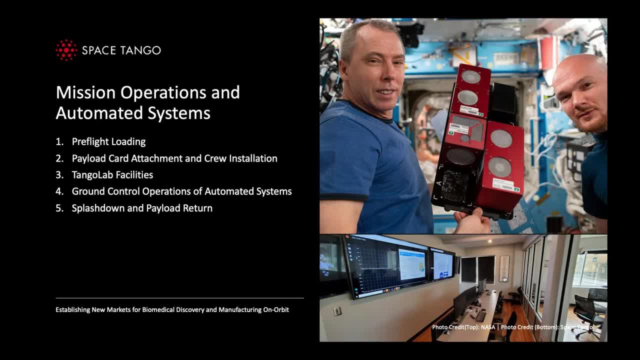 getting ready And, as anyone who has flown knows, launches are always called launch attempts because they Sometimes move and with biological payloads, you really need to be prepared to have other sets of cells that are available to you in case there's a launch slip. 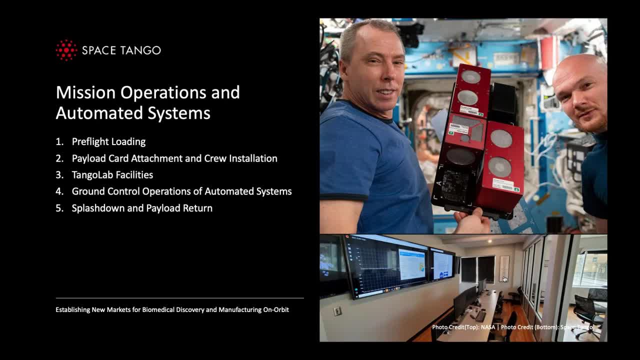 Once the actual pre-flight loading is completed, the payload is then turned over to NASA, It is loaded into the rocket and actually sent to the international space station. Once the vehicle docs, it's unloaded and the cube labs are then attached to payload cards that give us that remote capability. 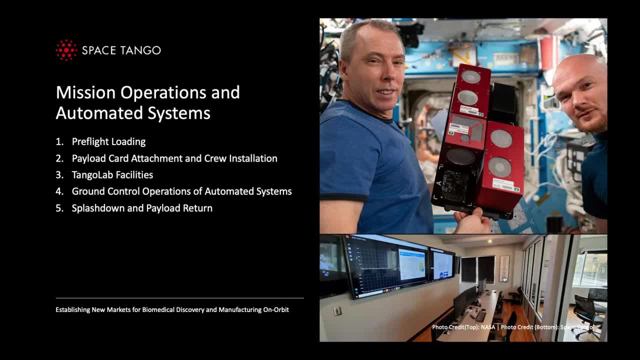 To control and see what's happening on the ground while we're on orbit and loaded into the Tango lab facilities. Once the ground control operations and the cell culture period is completed, then the reverse happens. The cube labs, as you saw in that video, are actually detached and you know, returned. 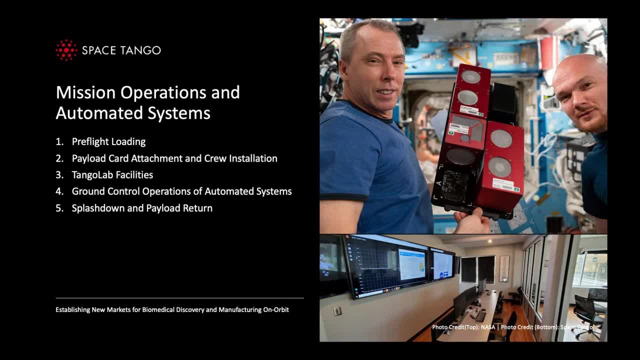 to us in the vehicle and then splashdown payload return, as Dr Zubair mentioned. you know we were picking payloads up, Since I'm here in California, right at Long Beach, and now this year we're going to actually be at in the Atlantic, so closer to the Kennedy Space Center where there are facilities to 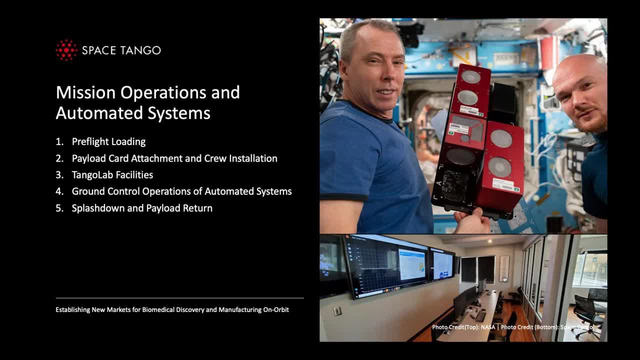 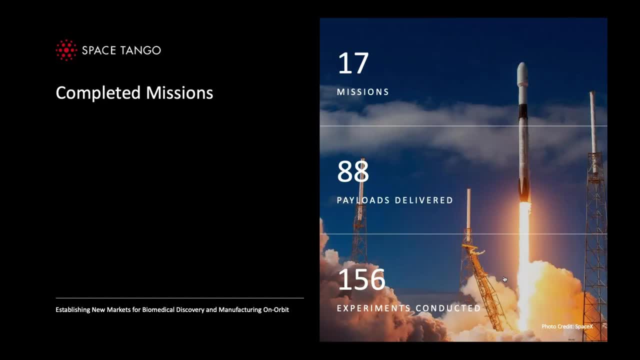 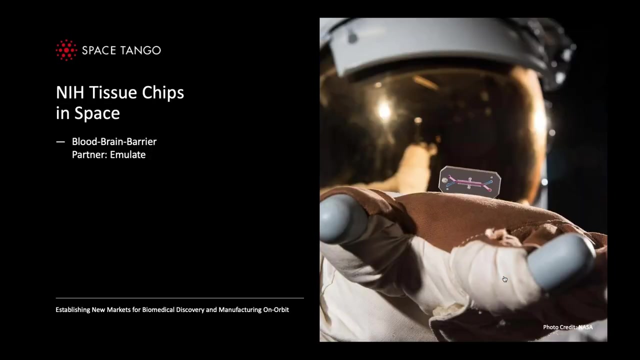 actually take your payloads and samples and right at return into those same facilities where you loaded previously. Just briefly so, we've 17 missions so far since our Tango labs were installed in 2016 and 2017.. 88 payloads and 156 experiments, and I'm just going to briefly give you an overview of the 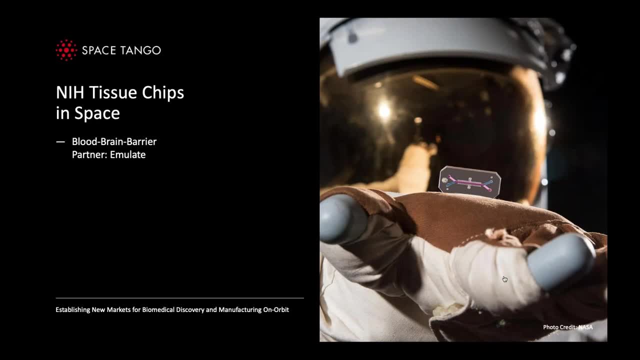 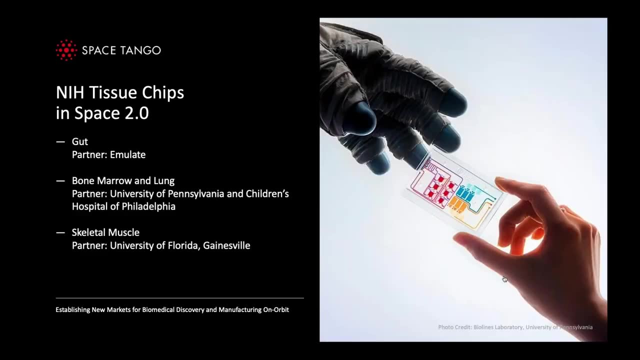 types of projects that we're working on right now. So I mentioned NIH tissue chips in space. we have a partnership with emulate doing a blood brain barrier chip. We also in the tissue chips in space 2.0, are working with emulate on a gut chip. 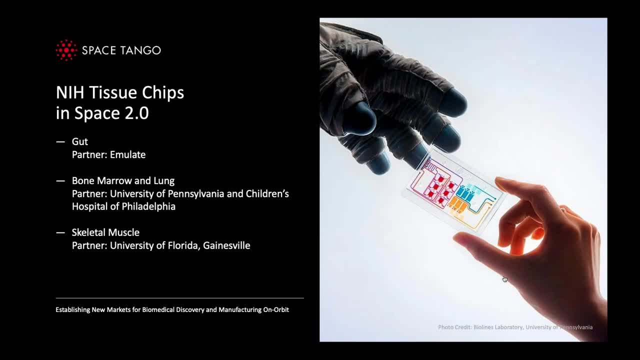 And we also have two other projects, one with University of Pennsylvania and Children's Hospital of Philadelphia for bone marrow and lung and one with University of Florida, Gainesville for scalable muscle. Really excited, These payloads are coming up on SpaceX 21.. So we're we're going to be very excited to see a lot of this work starting to bring. 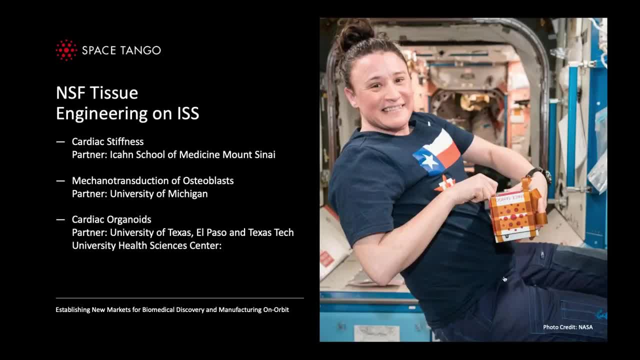 data back to us as well. In terms of the NSF tissue engineering collaboration that CASES has put together with NSF, we have three payloads that we are at We're actually supporting: one from Mount Sinai on cardiac stiffness, one from University of Michigan on mechanotransduction of osteoblasts. 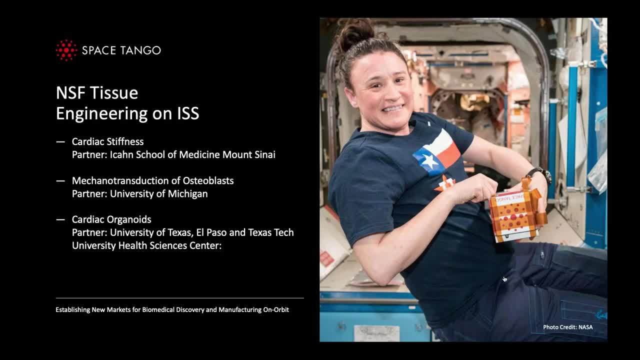 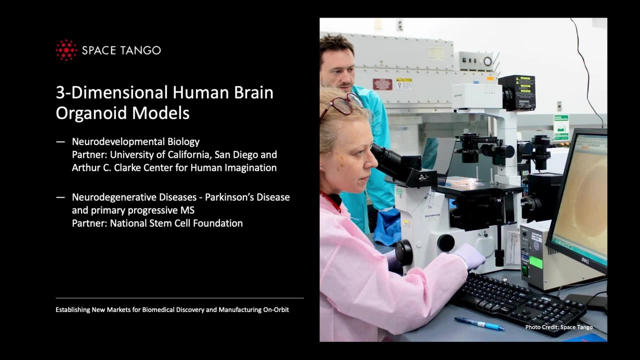 And then one from University of Texas and CASES is actually looking at cardiac organoids. So we're very excited to be working on several of the projects with NIH and NSF, And recently we also flew brain organoid models which you may have seen some information. 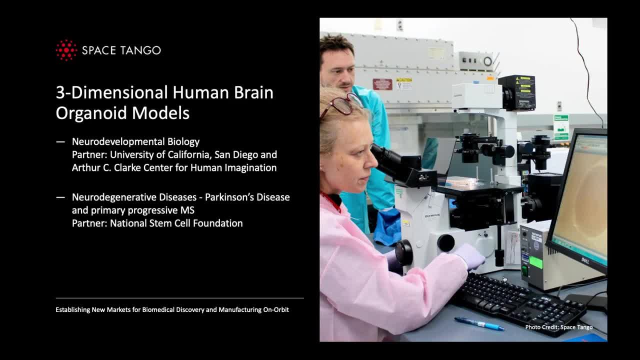 on these payloads as well. We're very excited to work with National Stem Cell Foundation and also with University of California and Arthur C Clarke Center for Human Imagination. These two organoid payloads- one actually looked at neurodevelopmental biology, so very. 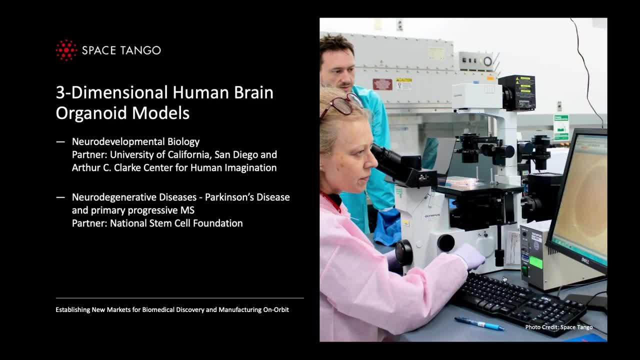 early stage organoids and the other one looked at neurodegenerative disease using iPS cells from patients with Parkinson's and primary progressive MS. So in addition to the more two-dimensional tissue chip work, we're also looking at the biologic models. 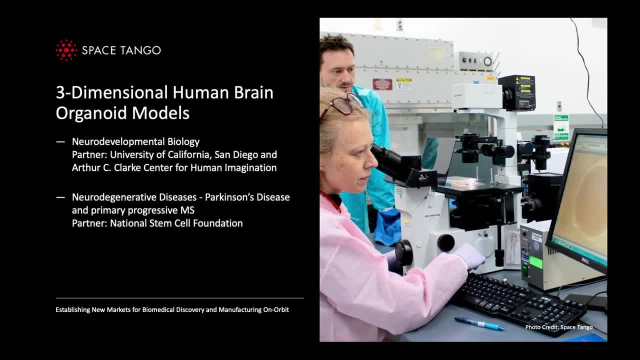 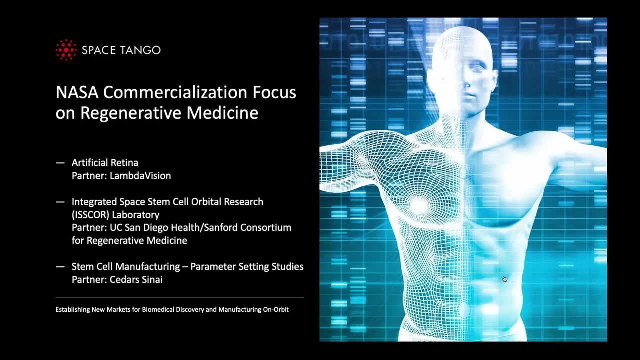 Moving up to three-dimensional stem cell models is something that you know again takes the biology to yet another level of sophistication, And recently, in April of this year, we actually were very pleased to be awarded by NASA three projects that are really focused on commercialization for regenerative medicine. 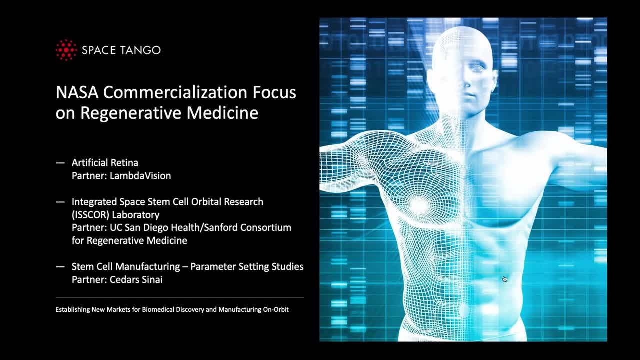 You know, the support of the public-private partnerships is really what will drive the development of stool cancer, but also the high risk of cancer sites, and so it's going to be nothing but a question and error for us to fund. We're really excited to be working with lots of the other activists from the joint efforts. 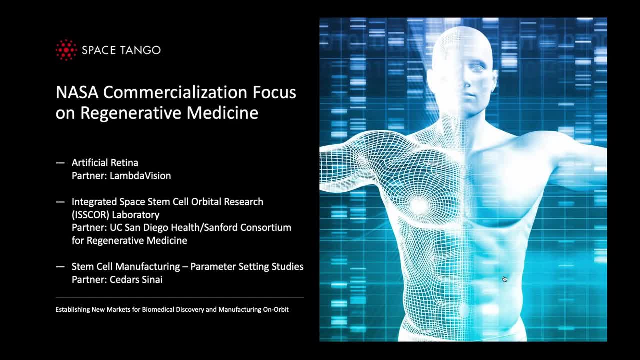 with the National Stem Cell Foundation and we're going to be able to incorporate some of those projects into this transition and to then bring attention to the natural health of young people who are getting those two projects. So I would be really excited to be working with Dr C Clarke, Dr C Clarke and Dr 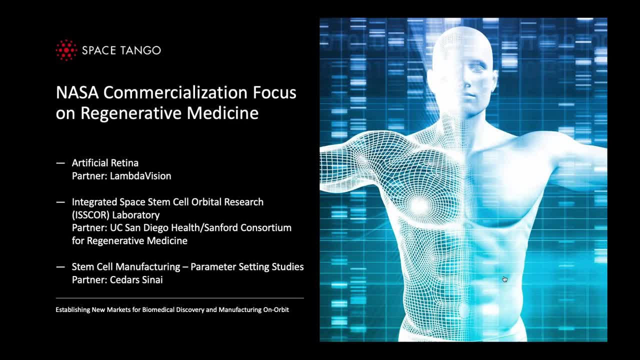 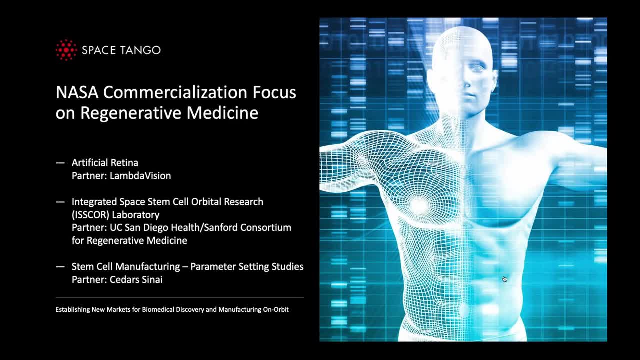 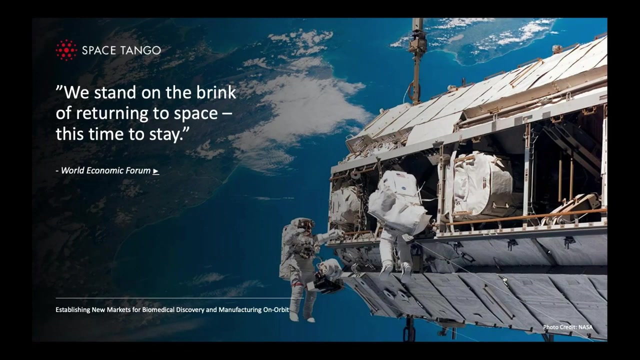 C Clarke, Dr Clarke, Dr C Clarke manufacturing. so these are all really exciting and part of the foundation that we're laying for these types of products, with the- you know- opportunities to manufacture, is setting up gmp capabilities for manufacturing as well. so to close, you know we really are on the brink of returning to space. 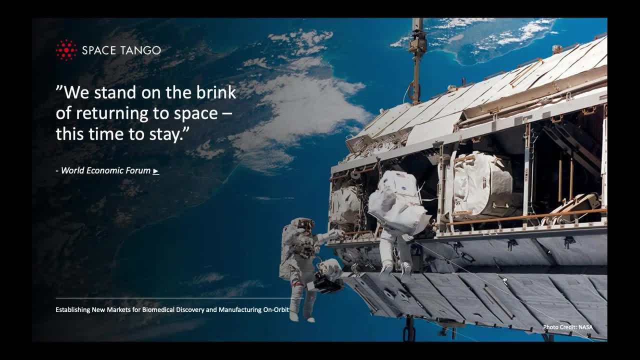 and this time it's going to be to stay. so i'm super excited to have the opportunity to work with all of the teams that we work with the great science that's being done for space tango to continue to contribute capabilities that are automated, that support sophisticated science. 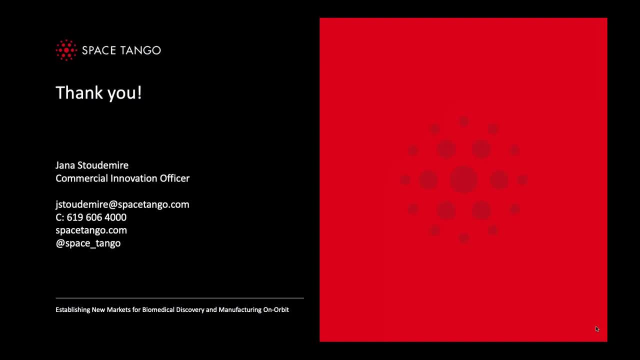 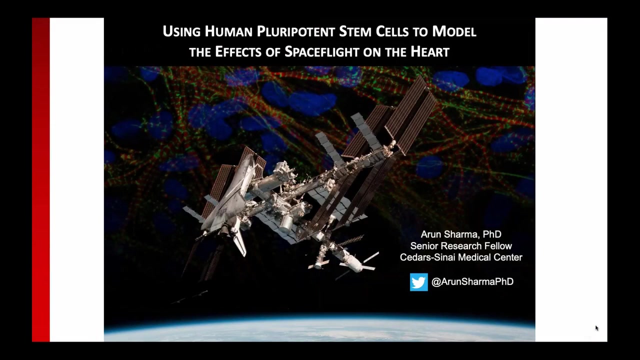 thank you, janna. as you can tell, space tango has thought a lot about how to conduct research in low earth orbit. again, if you answer, if you enter your questions in the questions tab, we'll get to them during the panel session. our next speaker is arun sharma, stem cell and heart biologist at cedars-sinai medical center's regenerative. 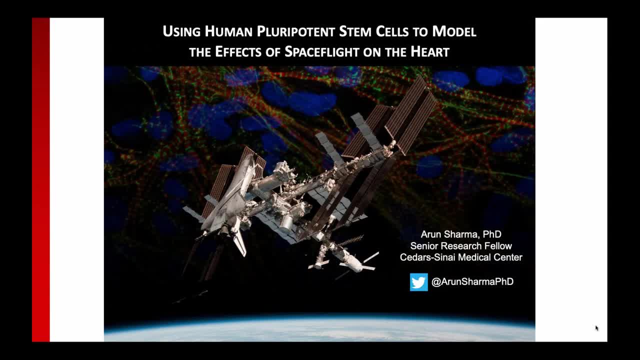 medicine institute arun, will tell us about using pluripotent, human pluripotent stem cells to model the effects of space flight on the heart, a paper that was published late last year and was conducted on orbit just about four years ago this month, arun. well, thank you for that kind introduction, liz, and 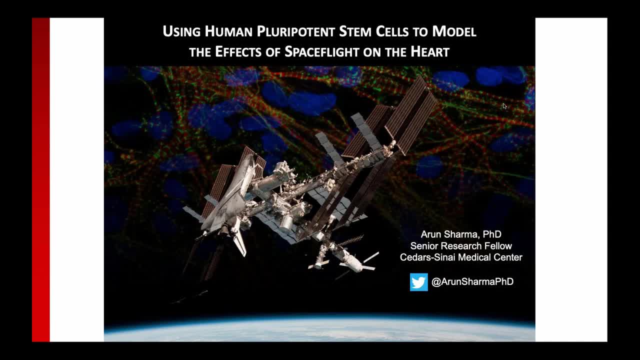 thank you for giving me the opportunity to talk a little bit about our work that we've done over the last few years utilizing human pluripotent stem cells to model the effects of space flight on the heart, and i'll be recapping some of the work that i conducted as a graduate student at 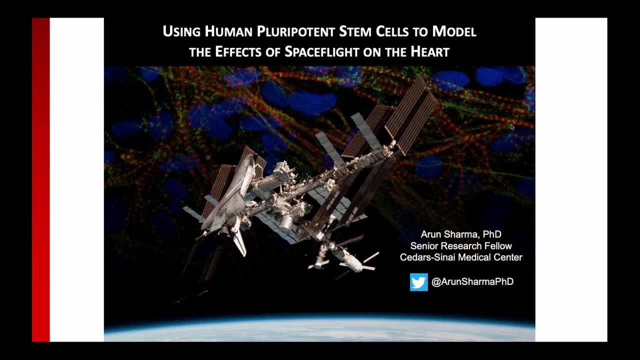 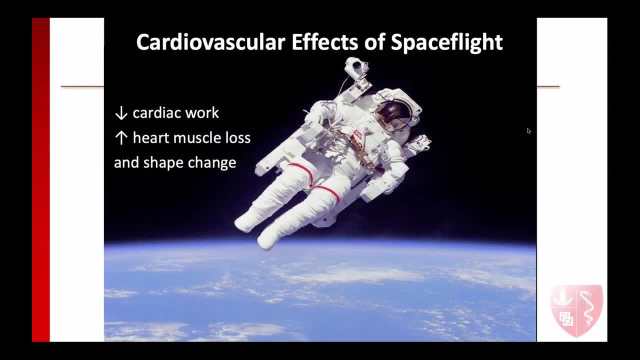 stanford university, in the cardiovascular institute, but i'll also briefly touch on some of the ongoing work that we're doing here at cedar-sinai: cardiovascular effects of space flight. why are we actually interested in doing this work? well, we have an understanding as to what happens to the heart as a whole, as a as a tissue. 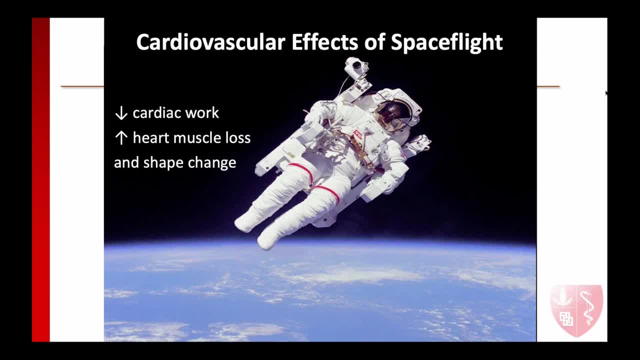 during extended microgravity, there's an understanding that there's a reduction in overall cardiac work as well as an increase in heart muscle loss, and this is as a result of that reduced cardiac work and also as a result from that muscle loss there's a shape change. that actually occurs. 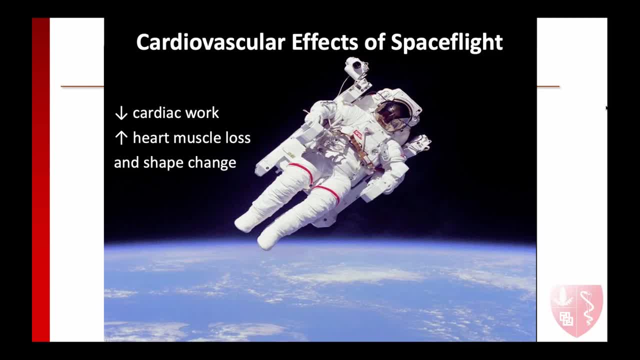 in the heart. the heart actually assumes more of a spherical shape on orbit as opposed to the traditionally fist shaped structure of the heart. so we have an understanding of what happens to the heart at the organ level, but we have less of an understanding of what actually happens to the 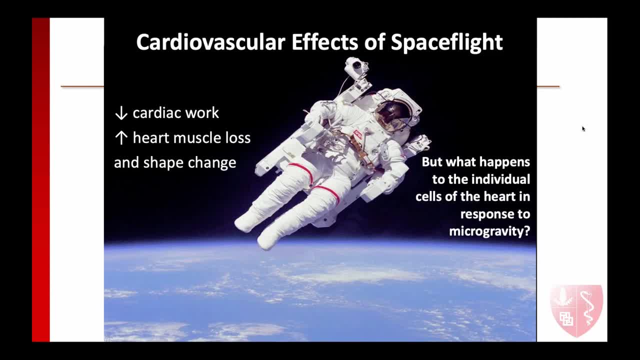 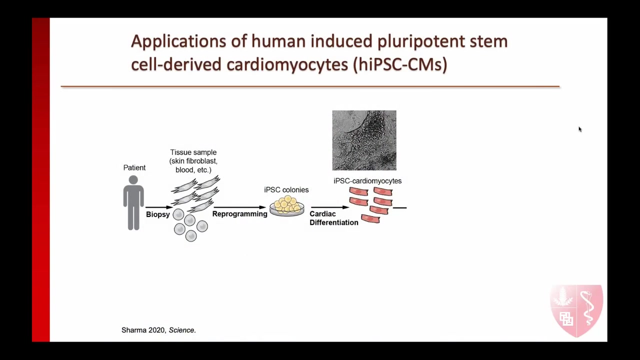 heart at the cellular level, and so we are using a couple of revolutionary pieces of technology in stem cell biology to really help address some of these, these issues and help us better understand what happens to the body at the cellular level in microgravity. okay, so we are using induced pluripotent stem cells and, for those of you who are on this call, 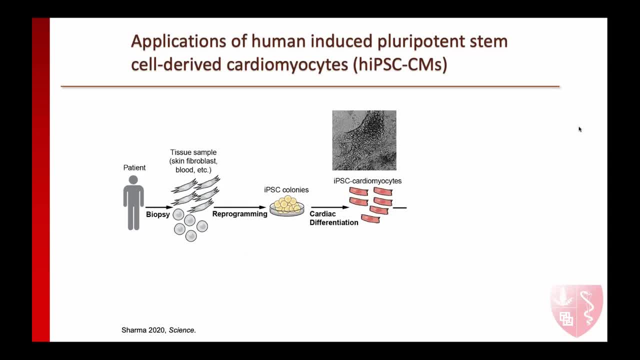 and have an interest in stem cell biology. these cells are, of course, no surprise and nothing new to you. but just as a quick recap, induced pluripotent stem cells are a cell type that is largely equivalent to the embryonic stem cell. these are cells that are able to be produced from a small sample of an individual's own skin or 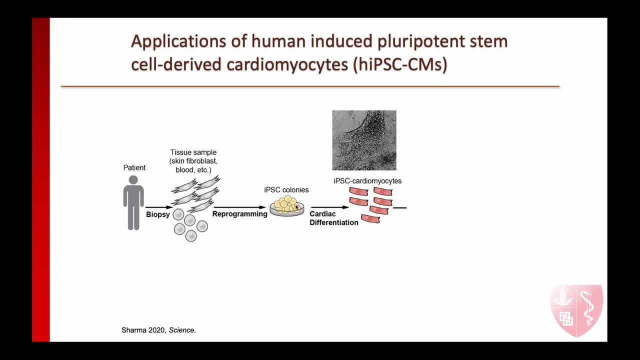 blood. they can be reprogrammed to induce pluripotent stem cell colonies and then from there differentiated into a variety of different cell types, such as cardiomyocytes, the muscular cells of the heart and, of course, the- uh the fun thing to the fun thing to note about these cells. 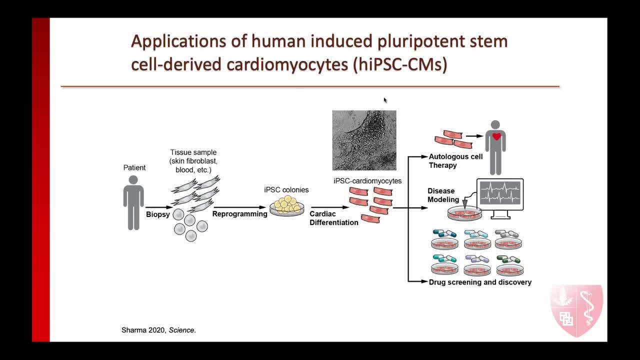 is that, since they are cardiomyocytes contracting heart muscle cells, they're able to spontaneously contract in a dish. there are a number of different applications for these cells, including potentially for autologous cell therapy, but the focus of this presentation and the focus of most of my work has been on using these cells for disease modeling, as well as for 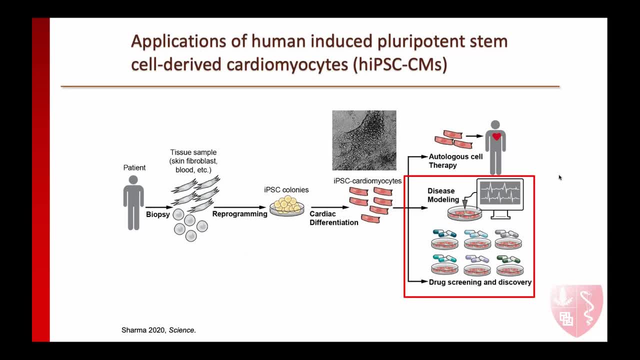 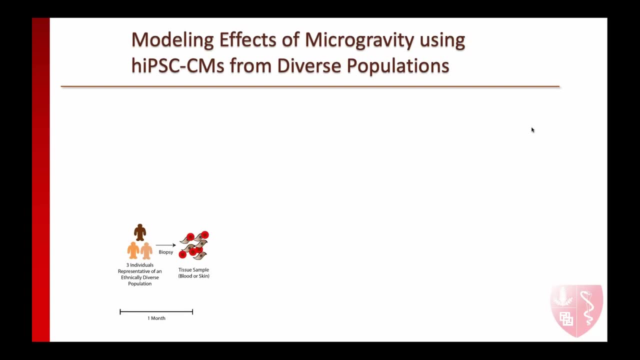 drug screening and drug discovery, and this using these cells for examining the effects of microgravity as an analog for the human heart. so i'll give a brief overview of some of the work that we did over the last few years. we have the good fortune to receive some funding from the center, from the advancement of science and space. and caseis to uh to arrive ipe to healing with breast implants with a right mnie paragraphs to Analog's Canal. obyyard, John Williamson. Love Island is an international research center leading a breach of the art and privacy guidelines within the National Lynch. The Three Path чуть reward from the Center for Advanced Science and Space and Case interns. 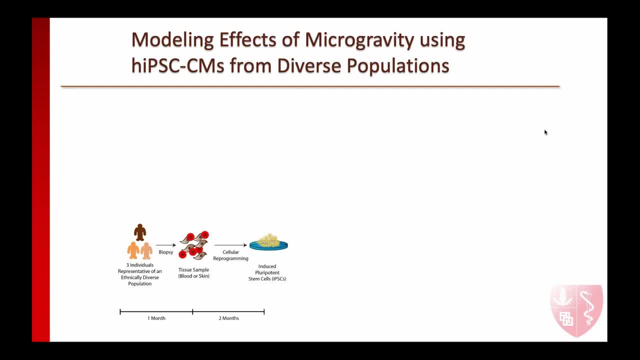 coleonえ links you to go reyne euberlca. in terms of treatment, co tone end ref carp tu moncler induced pluripotent stem cells from three separate individuals and then differentiate those cells into contracting cardiomyocytes, then transport those cells to the International. 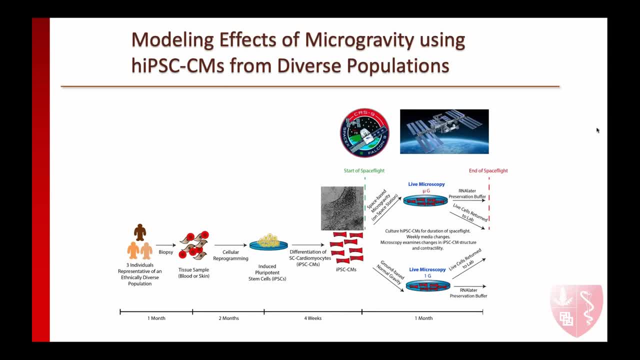 Space Station via a SpaceX Falcon 9 rocket. Of course we also had a parallel set of groundside control samples here on Earth so that we would be able to compare the effect of microgravity on our IPS cardiomyocytes on space to a parallel set of conditions. 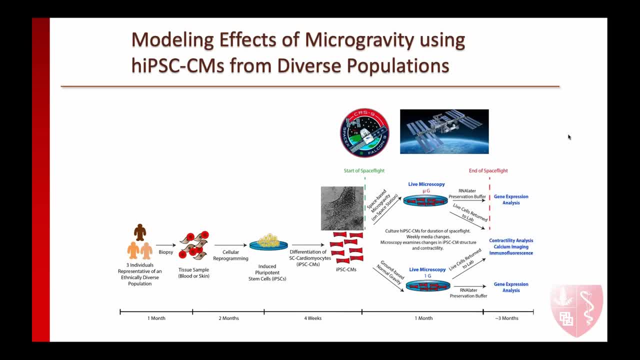 Once we were on orbit, we conducted a number of analyses, including gene expression analyses, looking at how these cells change in terms of their gene expression, as well as functional analyses for contractility, calcium imaging and structural cellular analyses using immunofluorescence. We also returned a sample of these cells back live to the planet for 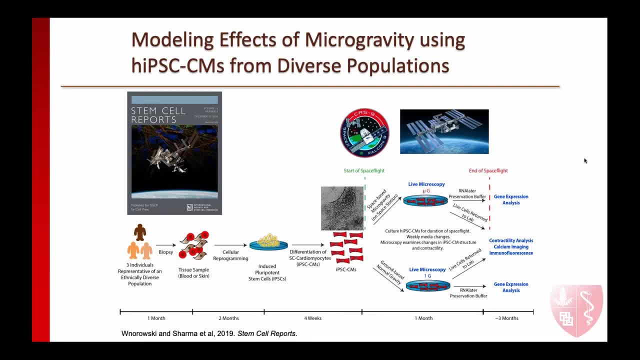 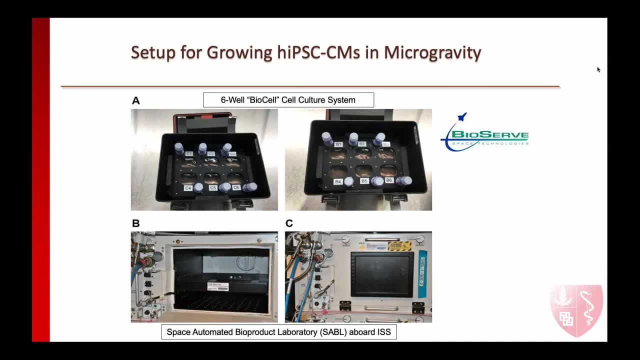 further analysis, And these results were actually recently published in stem cell reports- at the end of last year- so feel free to take a look. I'll give a brief overview of our approach to actually culturing these cells and also I'll talk a little bit about some of the data that we got from our experiment. This was 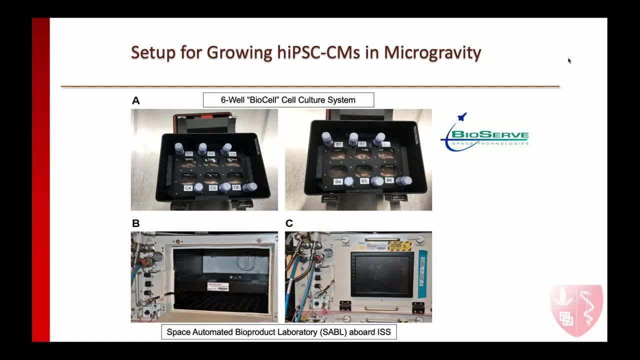 a very collaborative effort and our implementation partner in Biosurf Space Technologies helped us develop a custom set of standards to be able to have these cells cultured and able set of cell culture growth plates. These are fully enclosed six-well plates that have individual wells isolated to prevent cross-contamination. They're fully enclosed, of course, because 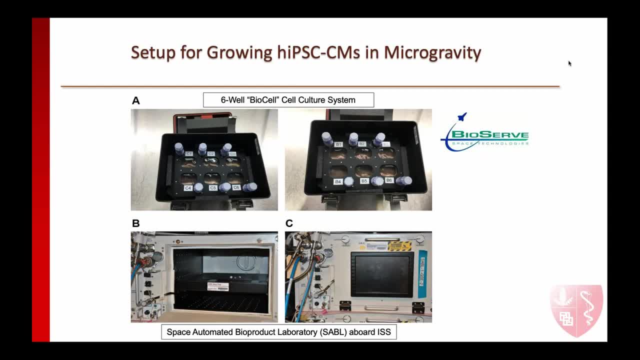 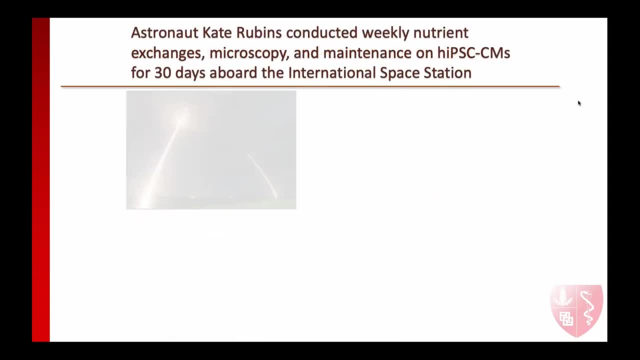 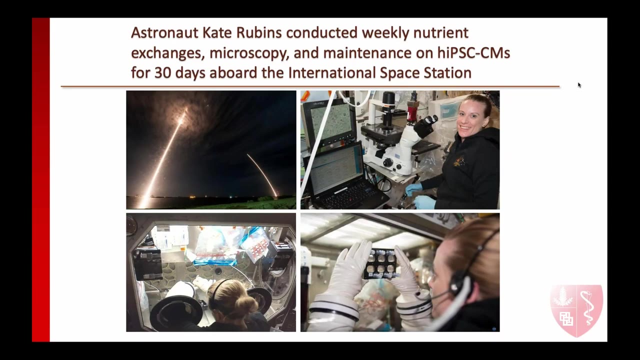 we want to avoid media and nutrients and cells from escaping aboard the microgravity environment of the International Space Station. So these were the culture systems that we actually used aboard the International Space Station. Perhaps the greatest assistance and the greatest help that we had for this entire project was from Dr Kate Rubins, who is not only a NASA. 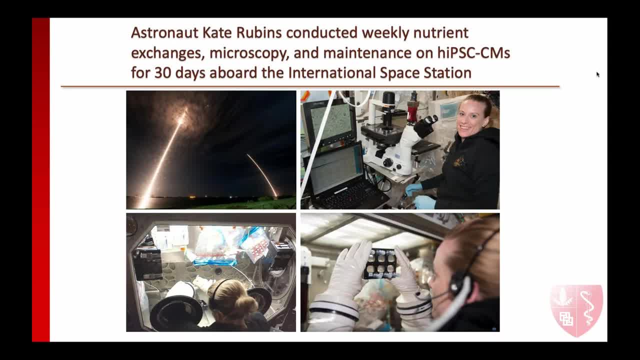 astronaut, but also a very talented cell biologist, as Jana alluded to in her talk. We had the very good fortune of working with Dr Rubins over the course of a month in the summer of 2016.. So that she could, so that we could actually examine the effect of microgravity on these. 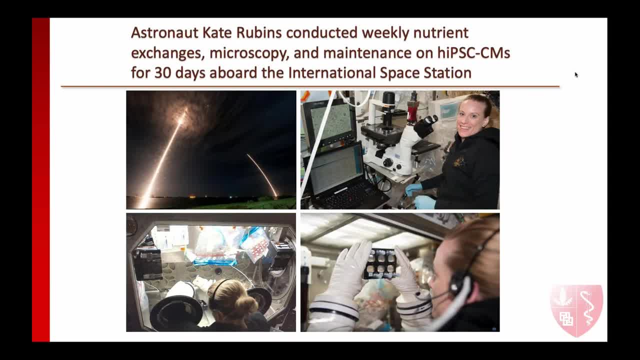 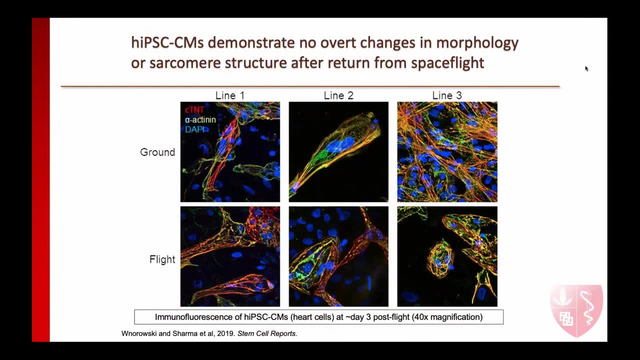 IPS cardiomyocytes, And what Dr Rubins was able to do was to conduct weekly nutrient exchanges on these cells to maintain their viability, also conduct microscopy and maintain the IPS cardiomyocytes for 30 days aboard the space station. So what did we find? I'll walk through some of the data and some of the results, but I 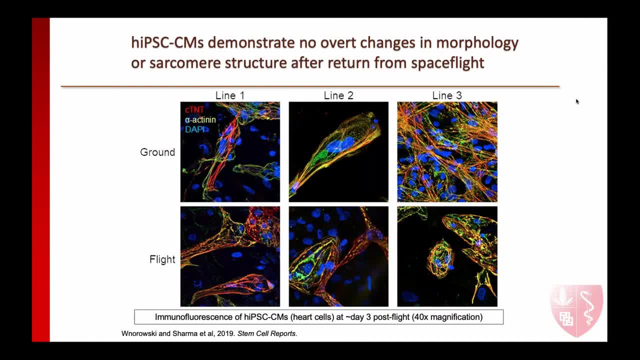 think we're going to talk a little bit more about what we actually obtained from these experiments. Well, first, we found at the macro level, the IPS cardiomyocytes did not exhibit significant overt changes in cell morphology or sarcomere structure after return from space flight. 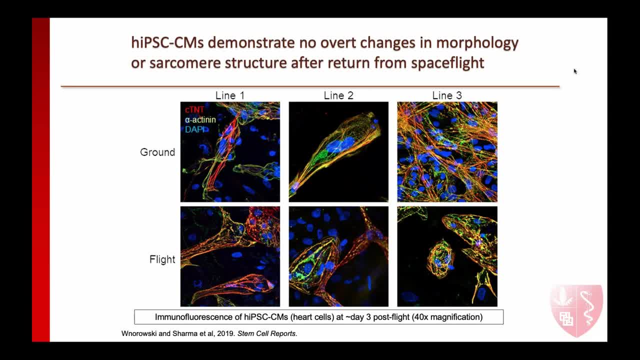 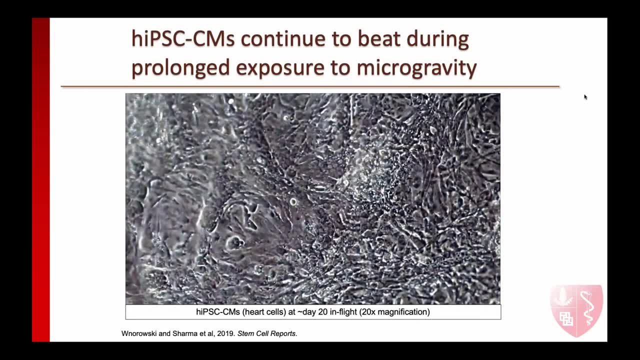 Sarcomeres are the individual contractile components of cardiomyocytes that actually enabled them to contract at the cellular level. As you can see here in this video, the IPS cardiomyocytes did continue to contract during prolonged exposure to microgravity, although there were some changes in the way the cells 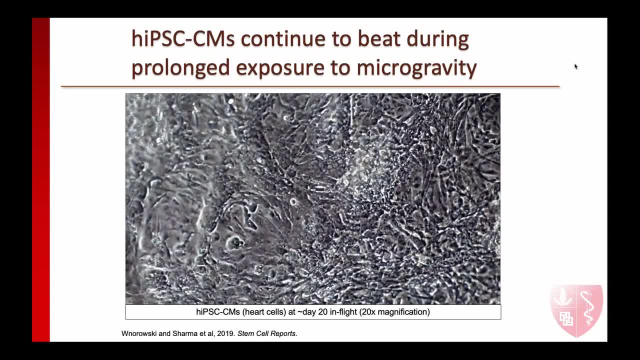 actually contracted on orbit. So this is. this was the first demonstration of long-term cell culture aboard the International Space Station. Again, as I mentioned, we cultured these cells for 30 days, And one other thing to note is that these are relatively advanced cells, As you can. 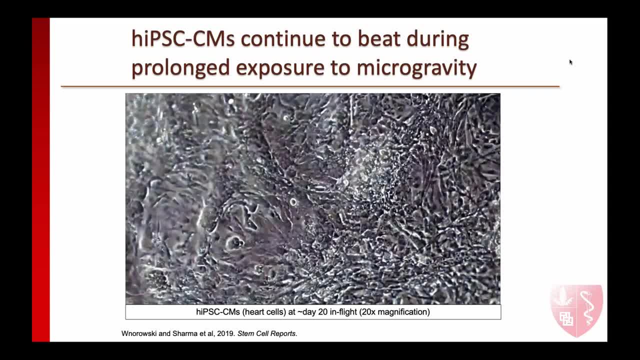 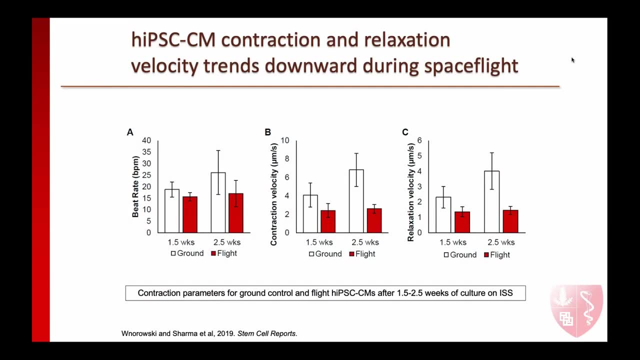 see here. they're functionally active, they're contracting, they're electrophysiologically active cells. So another important aspect of this project was to demonstrate that long-term cell culture is indeed feasible aboard the International Space Station. As I mentioned, we observed some changes in the way the cells actually contracted on orbit. 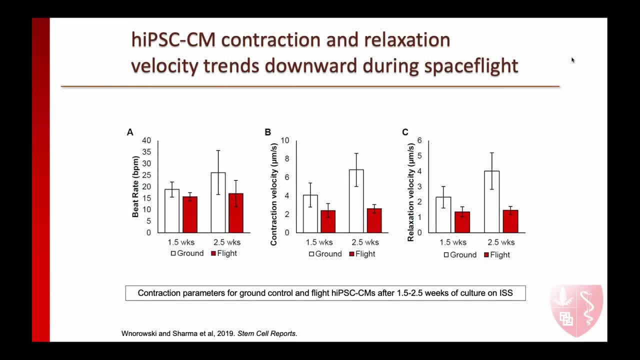 There was a trend downward in time In terms of their overall beat rate after up to two and a half weeks on flight. there's also a trend downward in their contraction and relaxation velocities as well, And so this may be a result of the cells adapting somewhat to their microgravity environment. 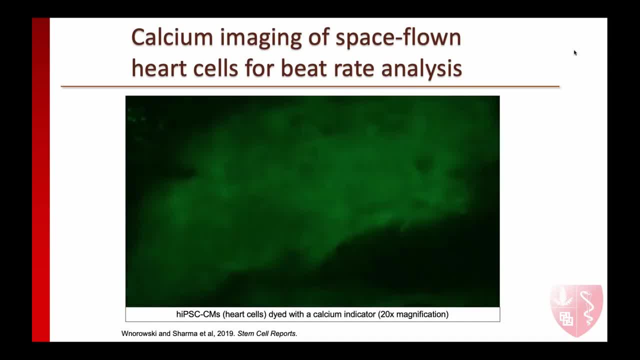 These are functional cells, as you can obviously see through the contraction of the other cells. And then there's also the separation, There's a split, there's a split in the contraction, and then there's a split in the contraction. And so, to elicit the contraction, cardiomyocytes have to undergo a, an excitation-contraction. 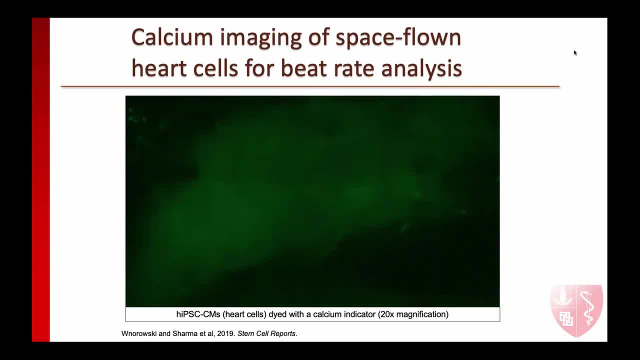 coupling process, where as whereby the calcium ions within the cells are actually activated and ultimately these ions are what leads to the individual contractions of the cardiomyocytes, And because of that reason, you can track calcium flow and calcium flux in individual cardiomyocytes. So we did calcium imaging on the space flow and heart cells After the contraction. what is what we did is we added a little bit of calcium to the cell and we had low calcium flow and calcium flux. So we did calcium imaging on these space flow and heart cells And 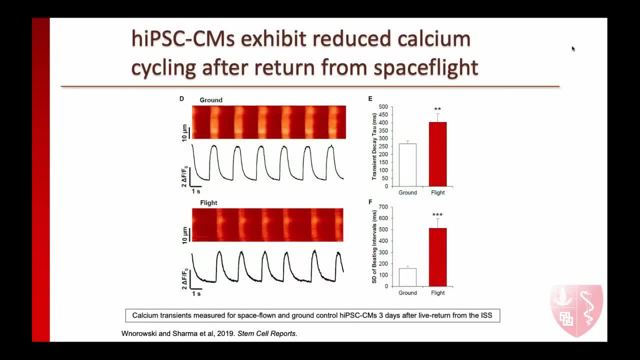 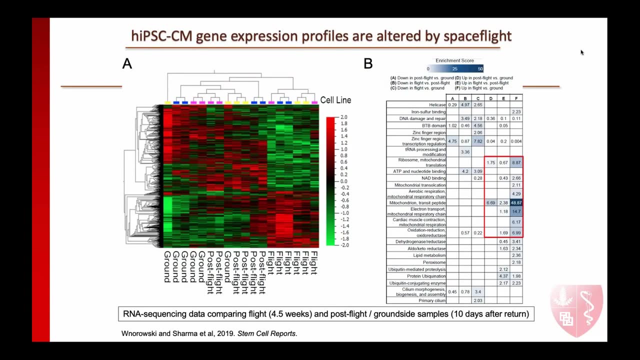 after they return back to the planet, as another functional indication of how the cells are behaving, And what we did observe is that these cells exhibit reduced calcium cycling after return from space flight. Finally, we're able to preserve a sample of iPS cardiomyocytes at multiple time points. 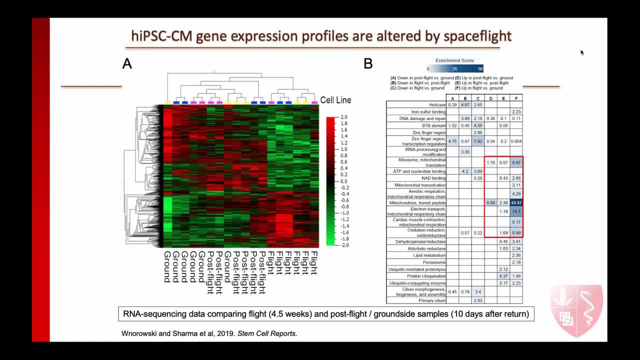 during space flight for RNA sequencing. So this is conducting gene expression analysis of space flown samples and compare them to ground-side controls, as well as post-flight samples- samples that were preserved after the cells returned back to the planet- And what you can see is that the samples 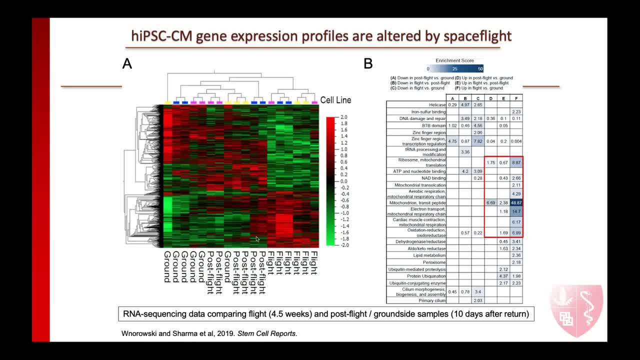 that were returned to the planet in the post-flight set of samples here largely show a similar gene expression profile to the ground-side controls, whereas the flight samples exhibit a slightly different gene expression profile based on the cells that are activated. based on the genes that are activated in these cells. 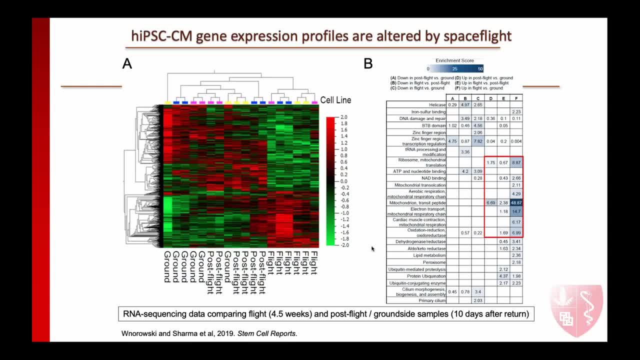 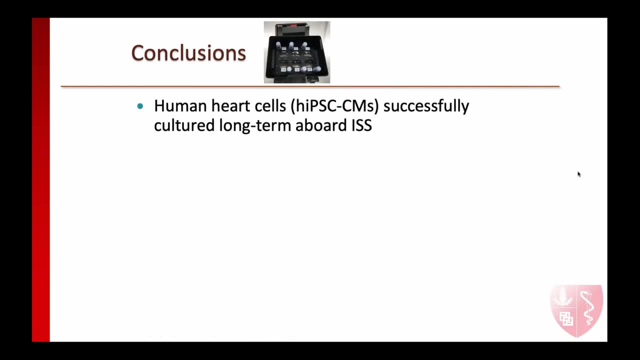 And if we took a closer look at some of the gene pathways that are actually altered in those space flown samples, we identified a number of genes related to mitochondrial and metabolic function. So, to conclude, we were able to demonstrate that human iPS cardiomyocytes, human iPS cardiomyocytes. 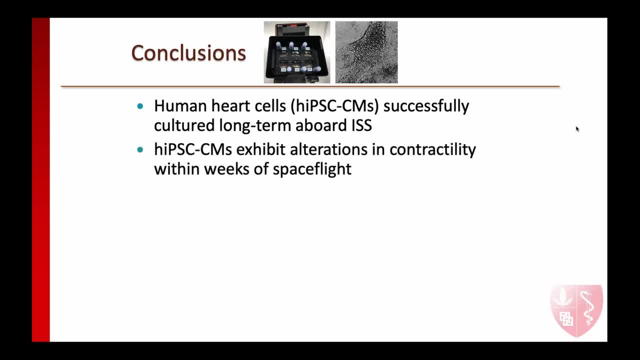 and human heart cells could be successfully cultured long-term aboard the International Space Station. As I mentioned, this was the first demonstration of long-term cell culture aboard the International Space Station and also a culture of a complex cell type a, functionally active, electrophysiologically active. 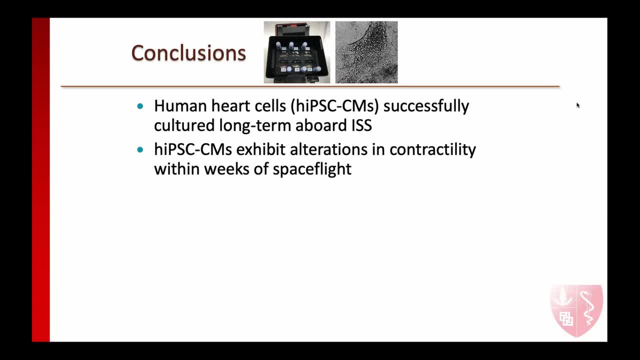 cell type in human cardiomyocytes. These cells exhibited some alterations in contractility within weeks of space flight, although did it not change their overall structure. as shown by immunofluorescence, They also show gene expression changes and, in particular, changes in pathways. 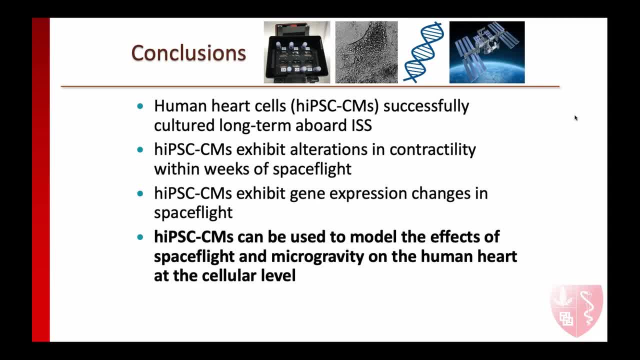 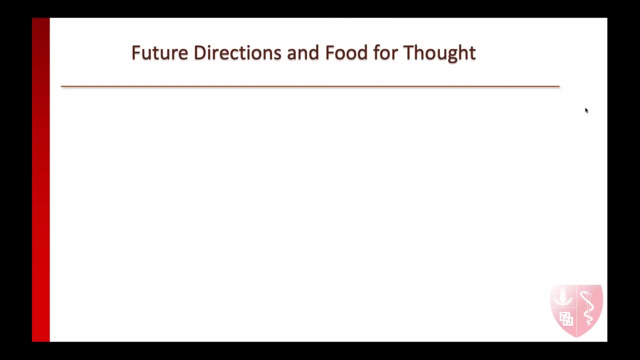 related to mitochondrial and metabolic function. And, ultimately, we believe that this is a useful model system that could be used to model the effects of space flight and microgravity on the human heart at the cellular level. So I'll leave you with some future directions. 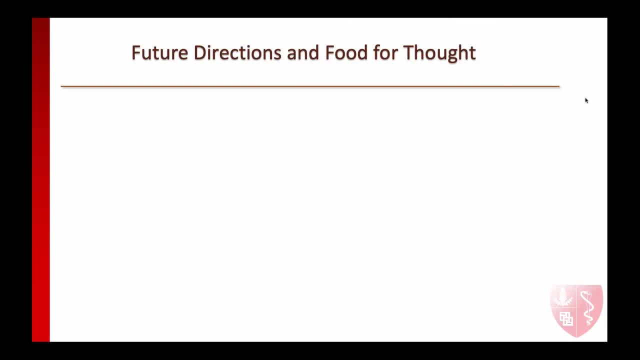 projects that are in the works and some food for thought, for additional analyses that will need to be done. How can we improve this particular experiment and this particular model? Well, this was a two-dimensional cell culture system. Everything that I showed you, all the data that I showed you. 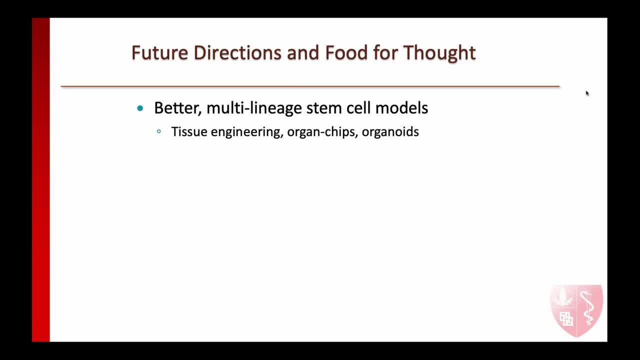 was from two-dimensional cardiomyocytes, cardiomyocytes grown in a monolayer. Ultimately, the human heart has a variety of different cell types that are important to its function: not only the contracting heart and muscle cells, but also endothelial cells. 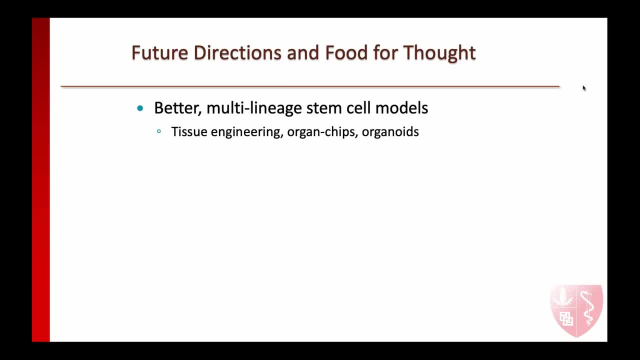 the support, fibroblast cells and so on, And a better model system- a better multi-lineage model system- would be able to leverage these other cell types as well. There are a variety of different improved model systems that are being developed right now, utilizing, for example, 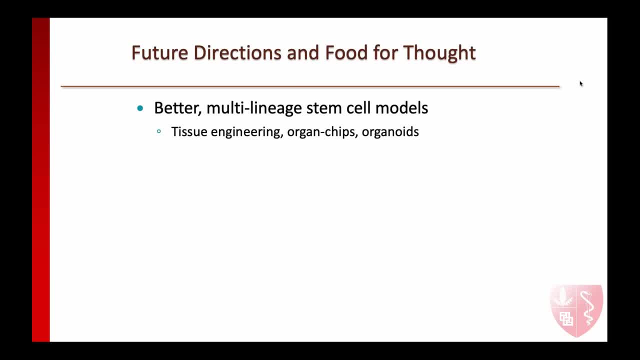 tissue engineering approaches that can artificially print multiple cell types into a single system organship, which is one of the approaches that Jana talked about briefly, where you can grow multiple cell types on an integrated organship which is connected through a pseudovasculature. 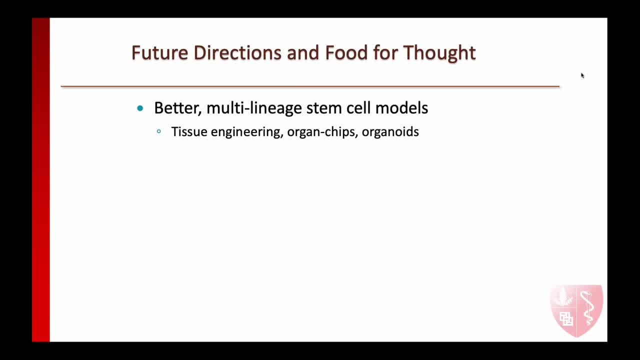 And also organoids. these three-dimensional collections of stem cell-derived tissues would also be a useful model system to better understand the effect of microgravity on the human heart. Additionally, there's a need for an automation of processes again, as Jana alluded to in her talk. 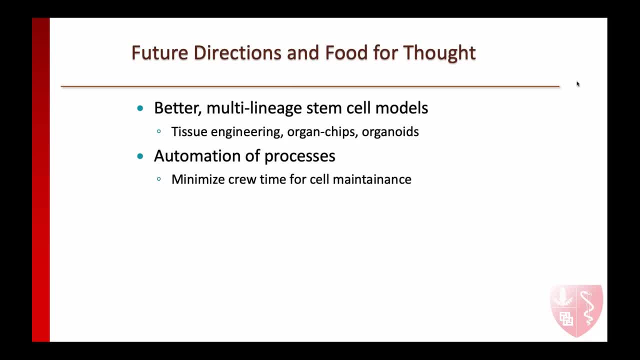 And this is also a very important part of the international space station's mission. So the international space station is a very important part of the international space station's mission, And so crew time is very precious on the international space station And although we were very fortunate- 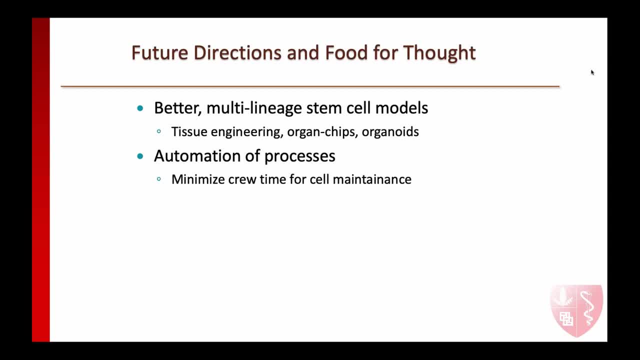 to have an astronaut working with us and Dr Kate Rubins, who has a background in cell biology. that's not always the case. Of course, the astronauts have a variety of other tasks to attend to, but this is a very important part of the international space station's mission. 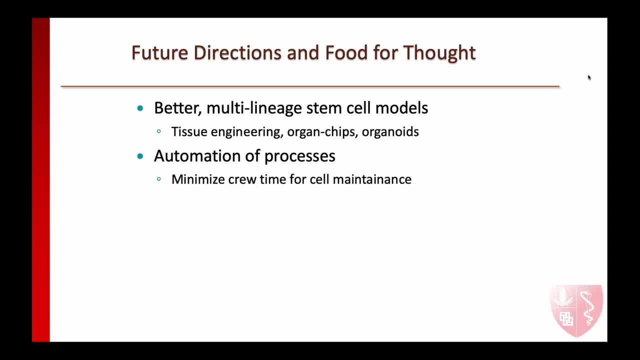 So if we can further facilitate the automation of some of these cell culture processes for maintaining these cells on orbit, that would be advantageous not only for the astronauts but also for the scientists as well. And finally, scalability and in-orbit production. 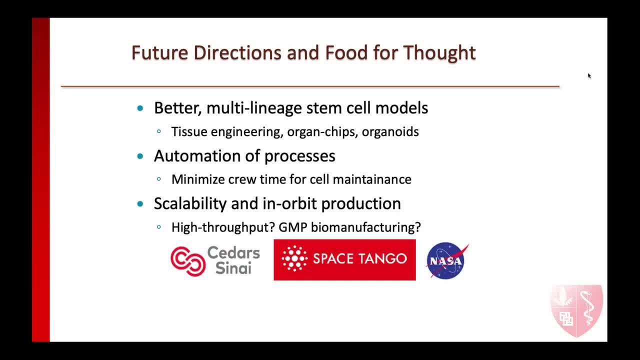 Is this something that would be feasible? There is some interest in potentially utilizing the station in microgravity environments as a means to, for example, to facilitate the production of stem cell populations and stem cell derivatives. This is something that you would have to examine. 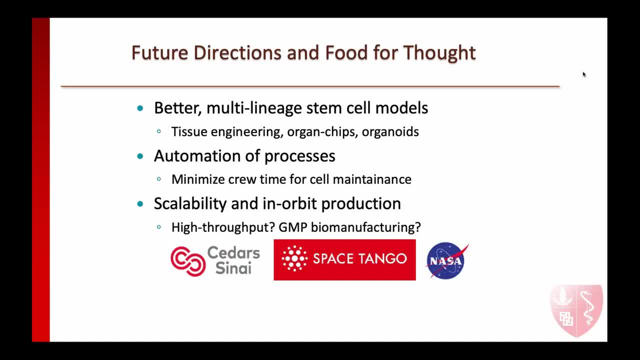 in the context of throughput as well. Can we manufacture these cells at a GMP or good manufacturing practices level, so that we could biomanufacture these cells and potentially use them for translational purposes back on the planet? And we've actually had the very good fortune to obtain a recent grant from NASA. 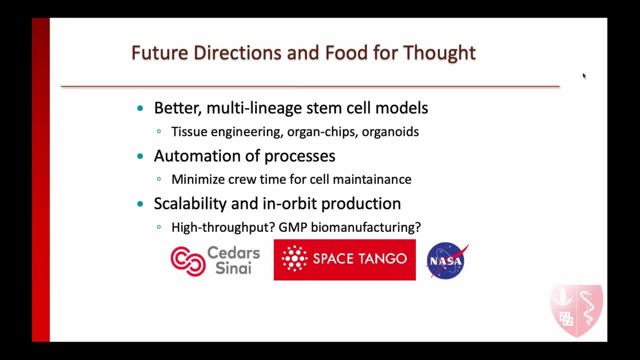 to further investigate this. This is with our team here at Cedars-Sinai, in collaboration with Space Tango, who has been developing a number of these automated platforms for facilitating cell culture on station, And so we're in the process of commencing that particular project. 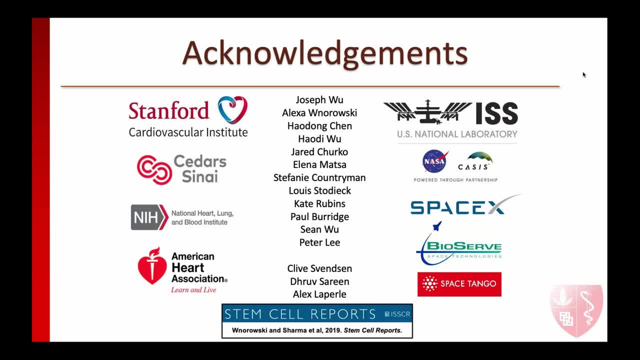 And with that I'd like to thank everyone who has been instrumental in helping get these projects off the ground- no pun intended, Of course- collaborators at the Stanford Cardiovascular Institute for the two-dimensional IPS cardiomyocyte projects, as well as collaborators here at Cedars-Sinai and Space Tango. 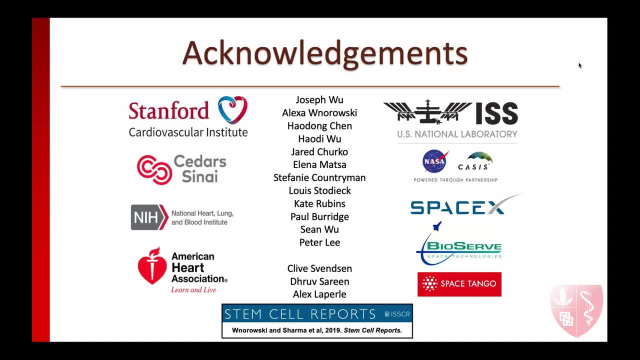 our implementation partners in BioServe, SpaceX and, of course, the Center for the Advancement of Science in Space, which has helped fund this particular work. And again for additional information on our IPS cardiomyocyte project, our two-dimensional IPS cardiomyocyte project. 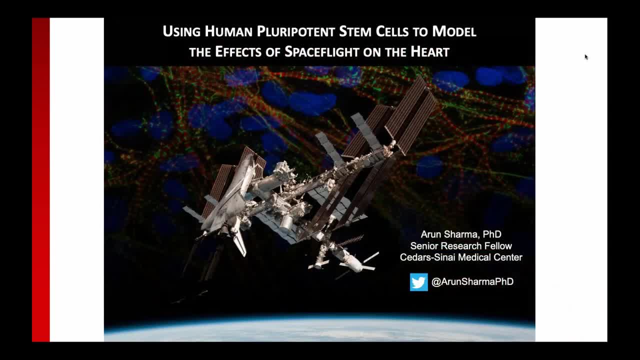 I would refer you to our recent publication in Stem Cell Reports. So thank you again for your time Fantastic. Thank you, Arun. You know that first heart cells experiment you described was really a pathfinder for the field and space And now we see that you're very much involved in the future. 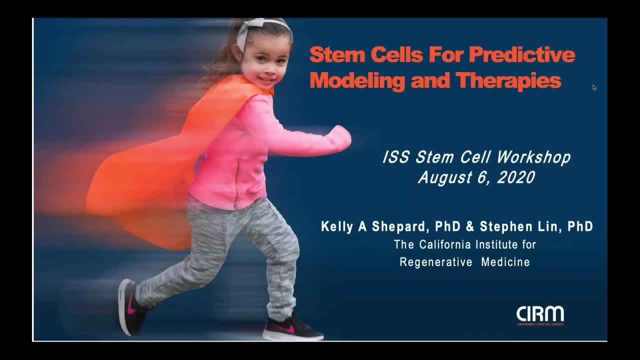 as well. Next, we have Kelly Shepard and Stephen Lin from the California Institute for Regenerative Medicine, CIRM. Kelly is the Associate Director of Discovery and Translation And Stephen is a Senior Science Officer. The mission of CIRM is to accelerate stem cell treatments. 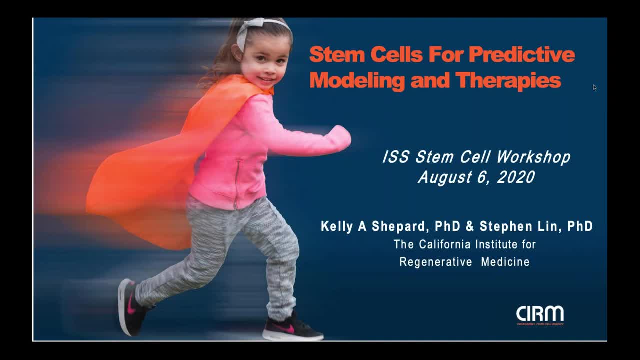 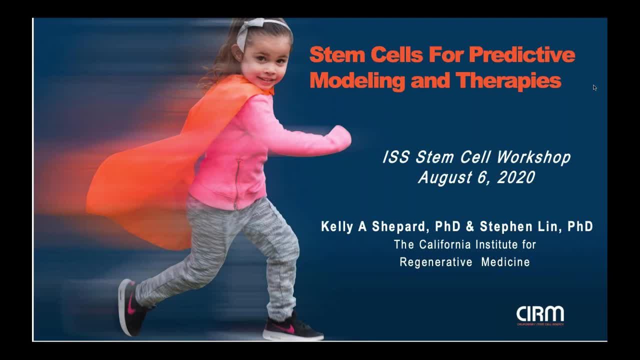 Thank you very much. Everybody can hear me. I assume I'm going to be asking for help with advancing my slides, because my connection may be a little bit slow, So I'll try to remember to ask for that. Anyway, I want to begin by thanking you for inviting us. 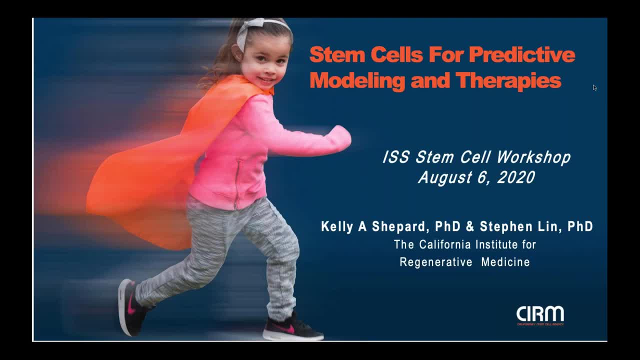 Stephen and I are program officers, as was mentioned, at the California Institute for Regenerative Medicine, or CIRM, which is a California state agency that was established by a ballot initiative in 2004 to fund stem cell research in California. Primarily, it was established to support 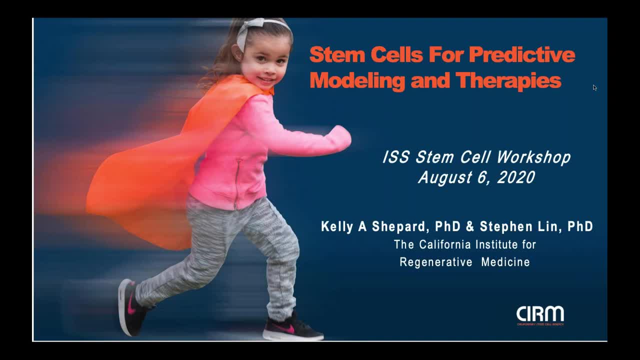 the use of human embryonic stem cells, but it actually supports stem cell research in a much wider variety of areas And we've been funding over 1,000 projects since 2004,. over the past 15 years is tag team. our presentation a little bit today. 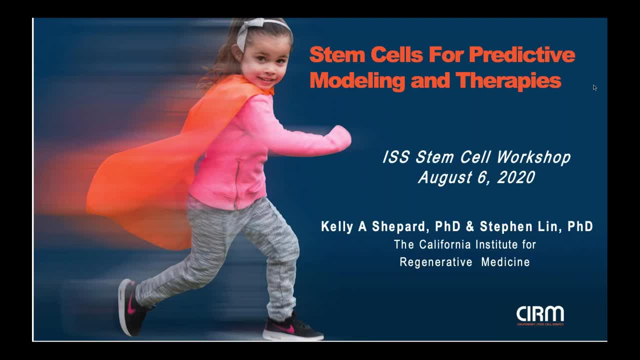 I'm just going to start things off by providing a bit of background on our activities over the past five, six years or so, since this is more relevant to what we're talking about today And this will provide some context for how our perspective has been informed. 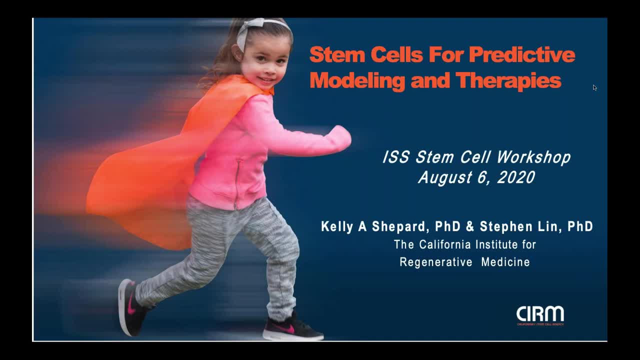 by what we see as current issues and needs in the stem cell field And then, after I go over that, I'm going to transition to Stephen, who will provide some specific anecdotes and examples of some projects from CIRM investigators and their relationship to projects that have been done. 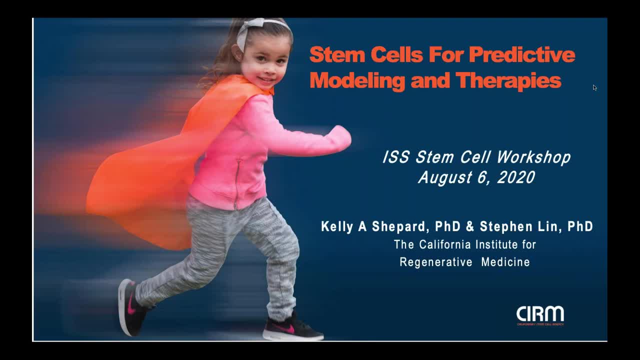 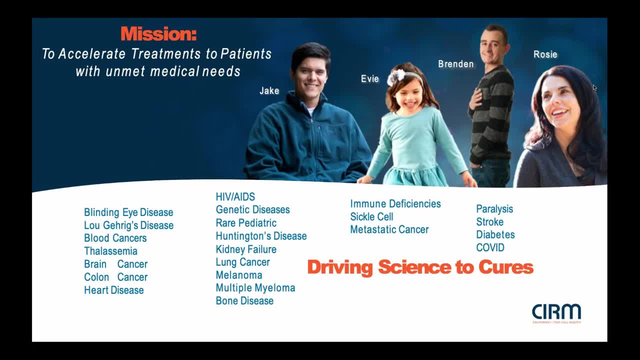 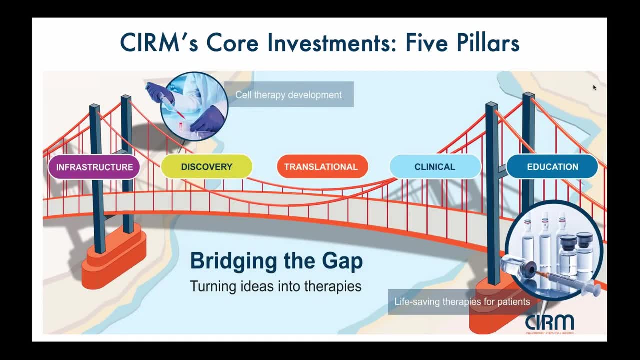 with unmet medical needs And our goal is to use stem cells in any way possible. to do this Next slide, please. Specifically, that means we fund research and development And we focus our research in five core areas which are depicted on this bridge. 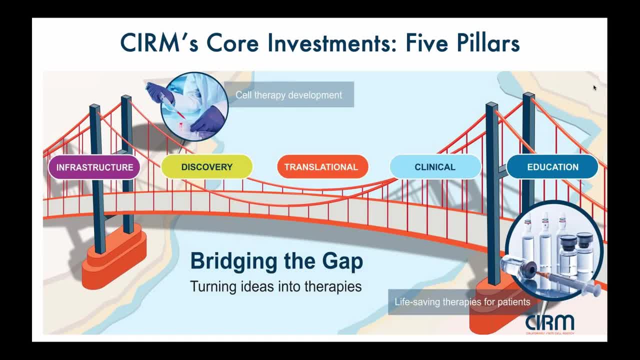 Sorry, I forgot to say came slides, didn't I? So I won't really be talking much about our educational pillar today, but I will be telling you primarily about some of the work done through our first core pillars here: infrastructure, which is to create resources. 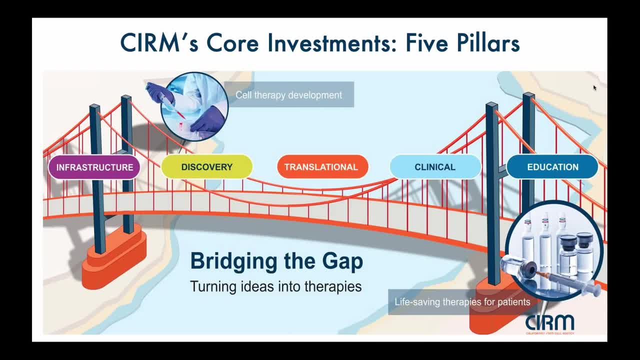 for the scientific community to use, And then our pipeline programs which fall under three different stages of maturity: discovery, translational and clinical. So by discovery I mean the earliest stage of research, And we have supported both from the very get go. 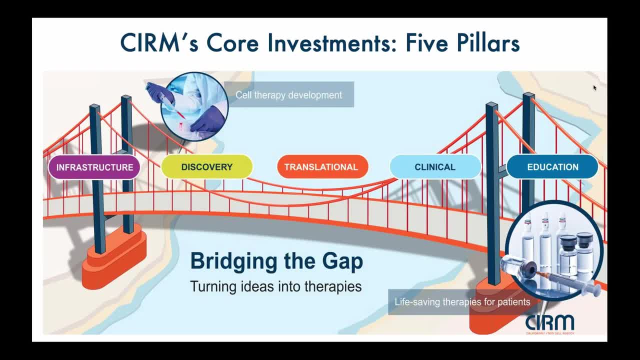 no preliminary data, hypothesis, testing new ideas, figuring out what happens, how to make things work To candidate discovery, looking for something that can be used as a potential therapy or as a potential tool for identifying therapies And knowledge generation. The translational stage is where somebody 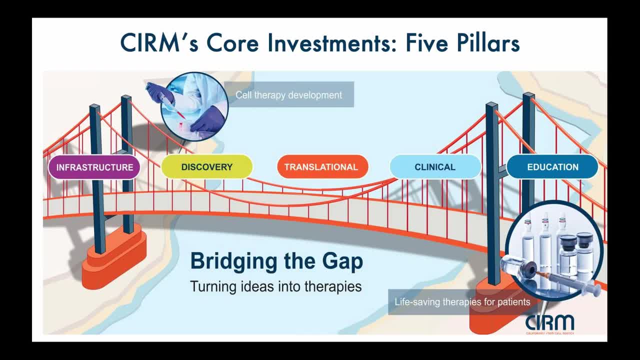 has made a promising finding in the lab, a development candidate, and they need to take it through the steps that is necessary to begin discussions with the FDA about bringing to a clinical trial. And then, of course, there's the clinical stage which, to CIRM, begins at IND, enabling, which is 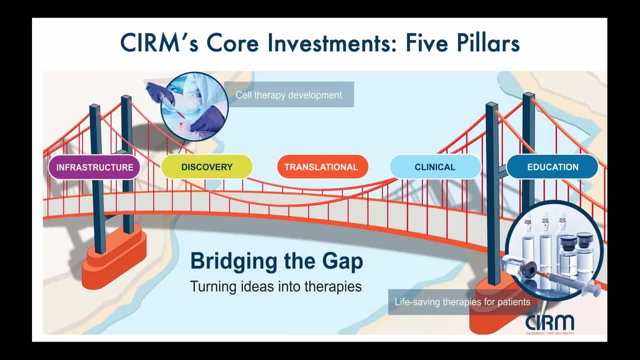 after you have agreement with the FDA on a promising set of studies that could lead to an IND filing to phase one, two and three clinical trials And ultimately- we don't have anything at this stage yet, but ultimately, hopefully, a drug approval. 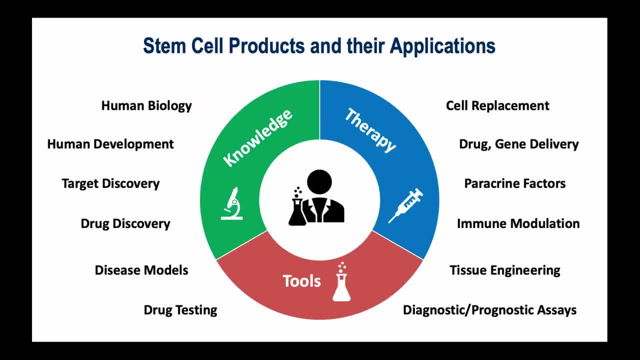 or commercialization. Next slide, please. So the types of projects that fall into these pipelines are quite diverse, as you can see. They cover a wide range of activities, but they kind of fall down into three basic areas. So knowledge generation using stem cells. 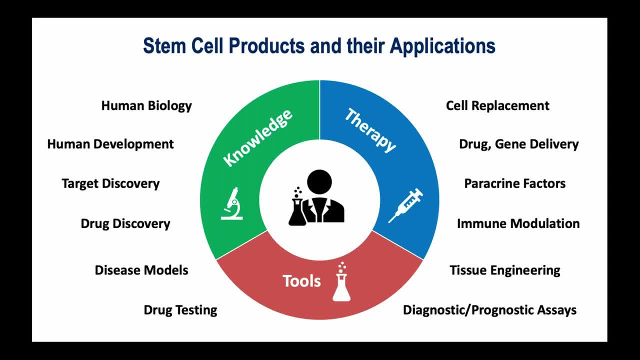 to understand basic human development and embryology, to understand the basis of human disease, to discover new disease targets. We also support a variety of projects where stem cells are used as a tool of discovery, So, for example, to develop a screening platform for drugs. 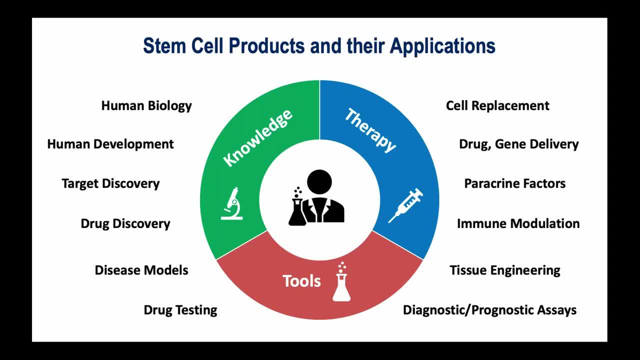 to model disease, disease in a dish, these types of studies. But we don't just fund stem cells as a tool, We also fund traditional tool development that can be used to enable the stem cell field, such as novel imaging modalities, new cell editing. 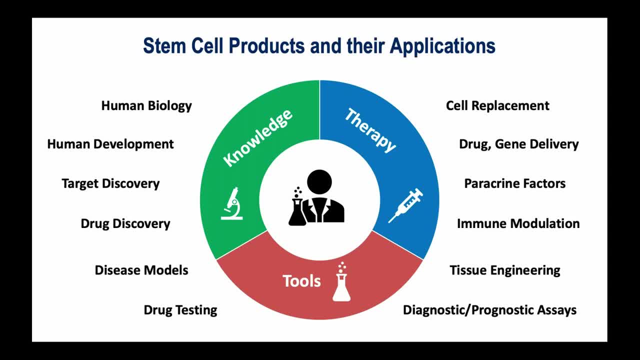 technologies- CRISPR-Cas9D, sorts of things directed towards editing stem cells. So basically, funding tools and technologies that can make stem cells more useful. We're also interested in developing things that can make automated processes because ultimately, to bring therapies based on stem cells. 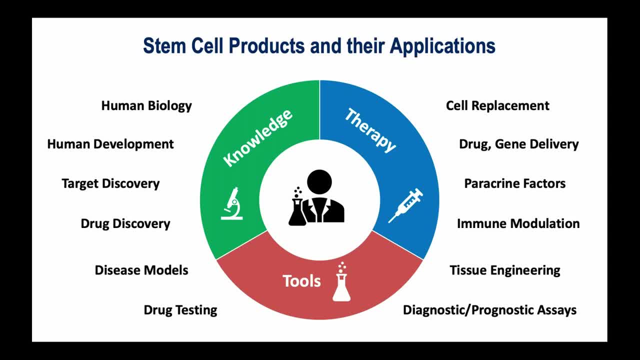 to the clinic. we need to make them more extensive and practical, reproducible and consistent, And so I see a lot of common ground there in the needs for what it takes to bring a study into space to what it takes to bring a study into the clinic. 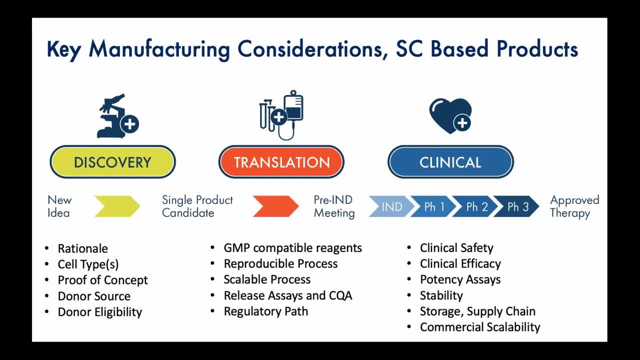 And so next slide, please. When we think about the types of these projects that I've just shown on the slide, across this pipeline, going from the earliest stage to the clinical stage, you're going to see a lot of common ground, as I said. 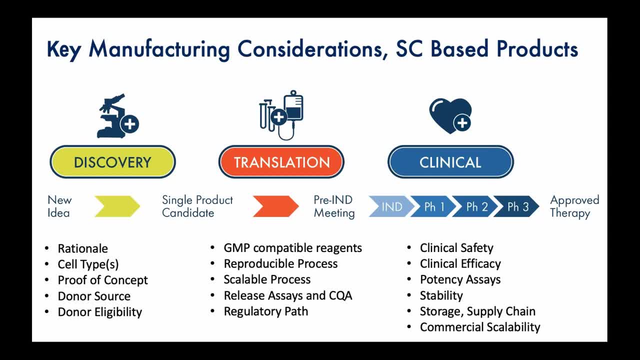 with some of the types of studies that are being conducted in space and being contemplated, and some of the studies, indeed, that we've heard about today, So at the very early end of the spectrum. some of the most significant questions then, when CIRM was founded, and now relate to the rationale. 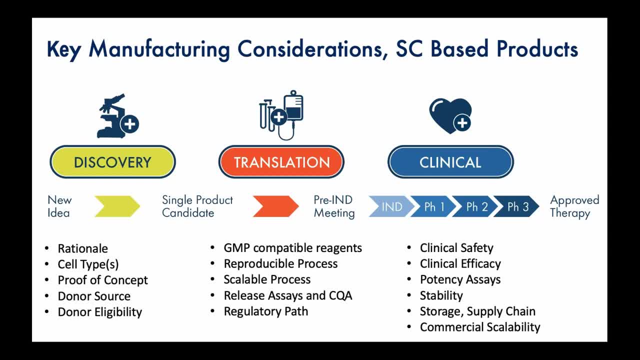 If you want to develop an application for a stem cell, what is the right stem cell type to use, or derivative of a stem cell? Do we know what our target cell is? Do we know enough about human biology to know which the right cell is to study? 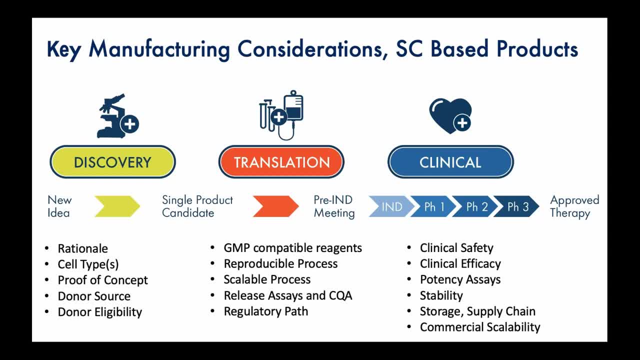 or is responsible for a disease? Is it one cell? Is it a group of cells together that are necessary? So, even if you know that cell, how do you procure that cell? A lot of the work that CIRM funds are trying to procure these cells. 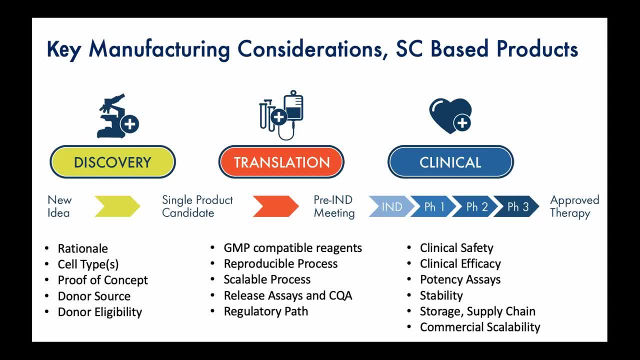 by differentiating them from a pluripotent cell starting point. That's a scientific process of discovery to be worked out on its own. In addition, stem cells can be obtained from tissues, from adult tissues. But being able to study human stem cells such as those, 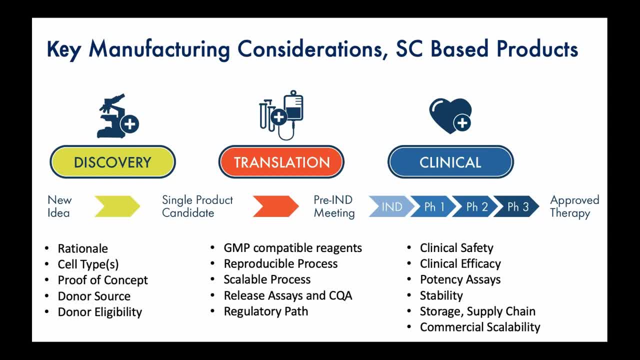 which have to be removed and propagated in the lab. there are a whole bunch of challenges around culturing and maintaining them in the lab. while they maintain their potential and functionality, It's very hard for many adult stem cells to maintain their ability to be expanded or even activated. 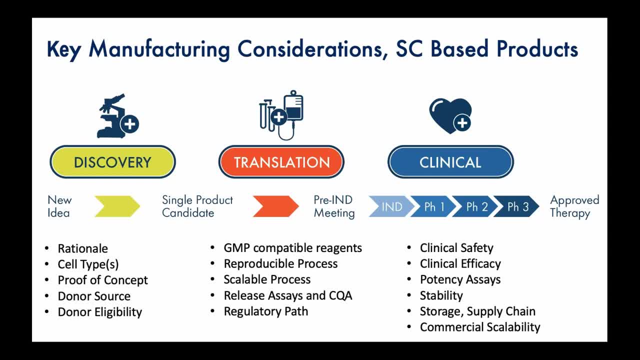 outside of their niche, which is normally in a tissue inside of an adult human organism. So other considerations that we have to think about, of course, even at the earliest stage, are donor source and eligibility. Eligibility because if you're going 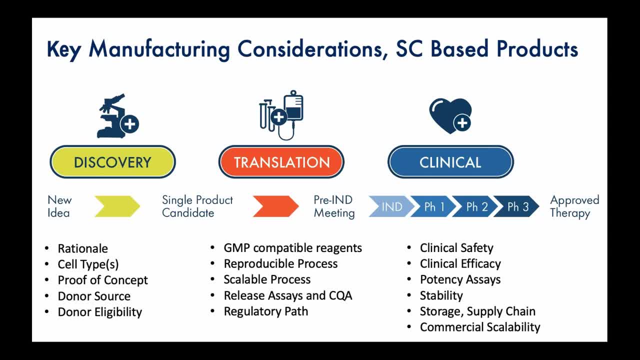 to eventually use one of these cells as a therapy, it has to be consented appropriately to get through the FDA approval process and to be ethically sound Donor source. we have genetic background of the donor. that comes into play. This is also important if you're interested in studying. 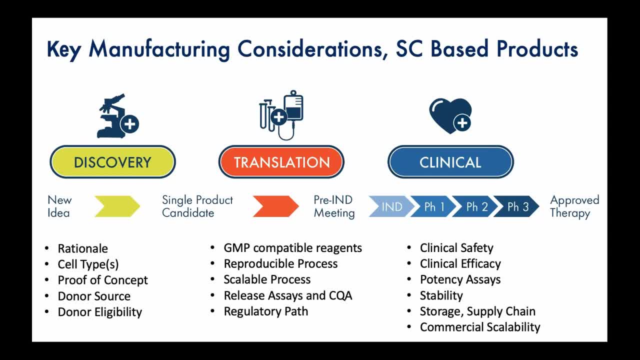 disease processes. You want to, as Arun mentioned in his talk, the possibility of taking cells from individuals with specific diseases so that you can model them in vitro. So those types of concerns As we move along to more mature science, getting into translation or early development. 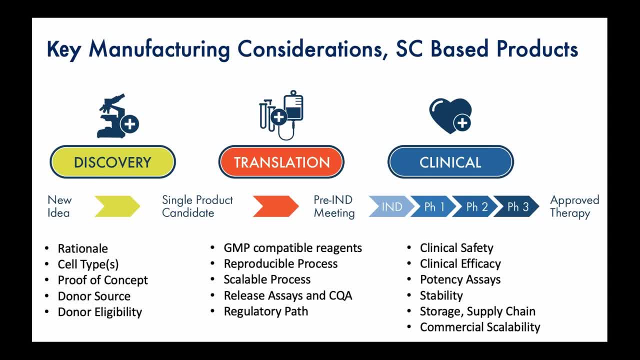 and eventually clinical trials, the challenges become quite different. So at this point you've already identified a promising stem cell-based candidate that you want to eventually test in a more broad use application. Here are the challenges developing, And we heard about this a little bit in our first presentation. 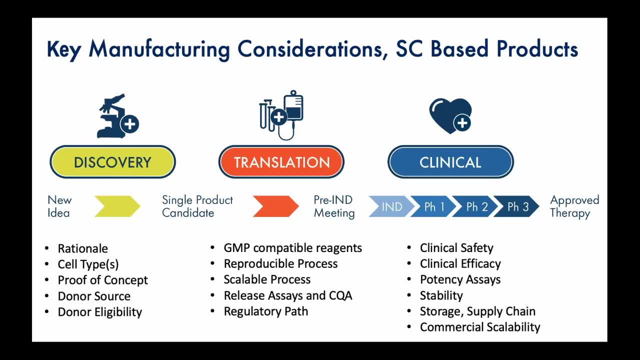 as well is the scaling up. You're going to have to go from a dose that might have worked in a rodent to a dose that is going to be effective in a person, So you're going to have to be able to grow the cells. 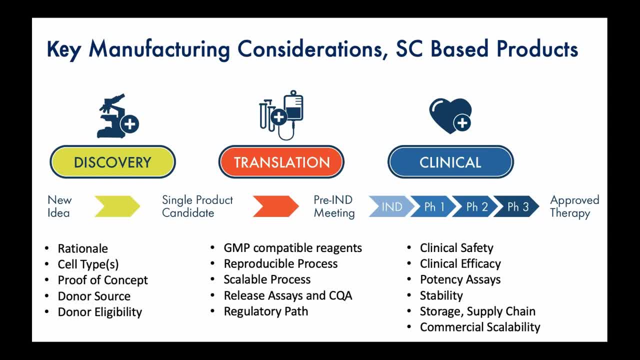 in much larger numbers, while maintaining their functionality and potential. And not only that, you're going to have to change your process so that it meets GMP compatibility requirements, so that it can be produced in a gene-compatible manner. And that can change. 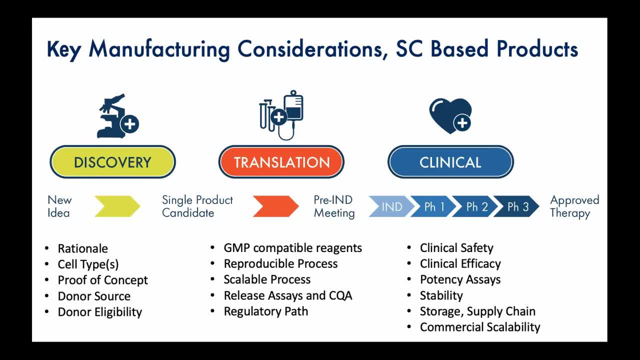 That can have effects on yourself. So a great deal of challenge, especially in our field, is centered in this space, Right here and right now, And that's developing the GMP-compatible process and scaling up process And, although some projects have made it into clinical trials, 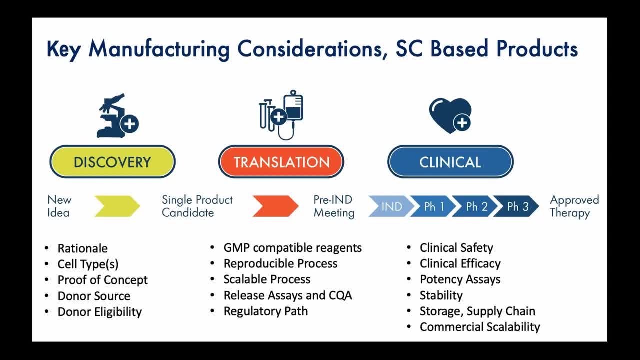 of course, there are a whole new set of challenges that they're facing and navigating now and will continue to do so, And there's even more scale-up that will need to happen If this is going to be something that is going to be offered. 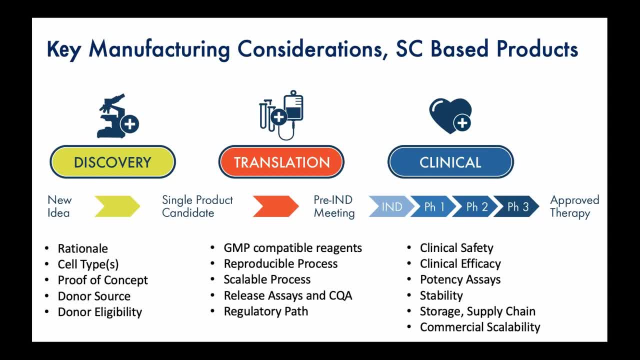 as an approved drug to a more widespread disease. you can't just make enough cells for one patient. You are going to want to treat a lot of patients, So you have to be able to develop a commercial, scalable process. You have to figure out how are you going to store and ship. 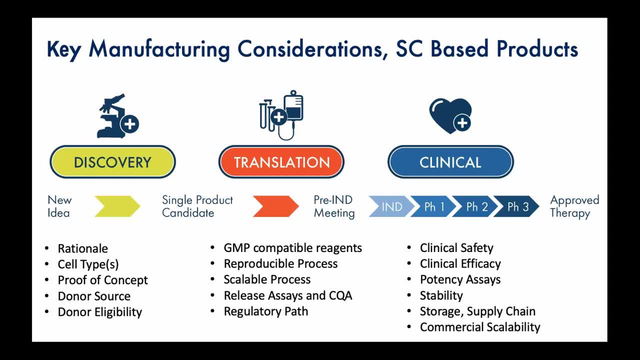 your cells And all of this. you have to maintain the integrity of the cells, And so we're not quite there for most of the types of projects that CIRM funds, but these are the challenges that we see as looming on the horizon. 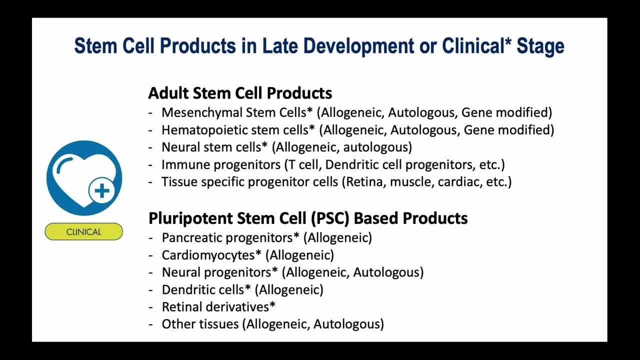 Next slide, please. So this is the state of the field today. There are a number of stem cell projects that are in clinical stage trials or very close. The more mature therapies that have been worked out, longer are the mesenchymal stem cell products. 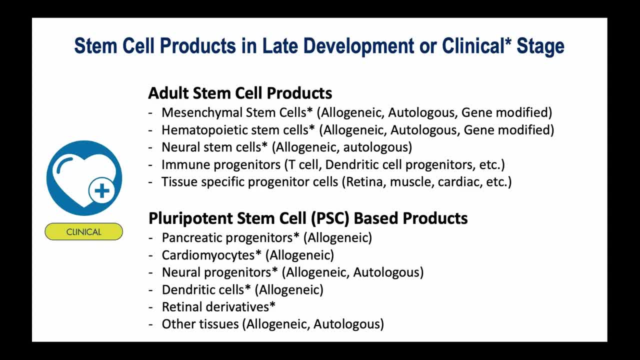 And we also have a long history of bone marrow transplants now, which are basically hematopoietic stem cell transplant. There are also some examples of some primary neural stem cells in the clinical trial, as well as immune progenitors such as T cells and dendritic cell progenitors. 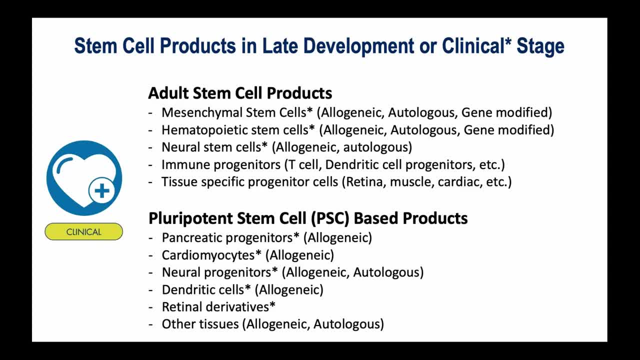 and other tissue-specific progenitor cells. There are also now some pluripotent stem cell-based products that are also in clinical trials. You may be aware of some of these. We have pancreatic progenitors. There are some cardiomyocytes derived from human embryonic stem cells. 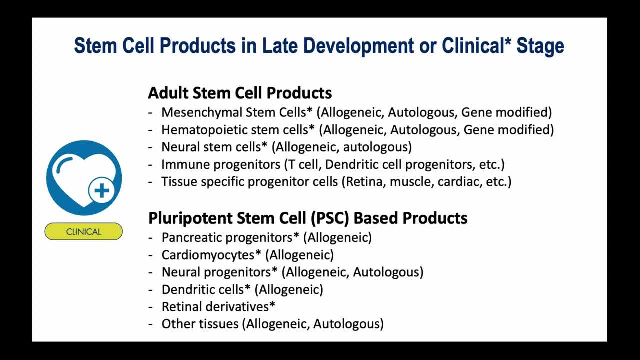 Neural progenitors, dendritic cells, retinal derivatives- The ones with little asterisks are the ones that are currently in clinical trials. The others are getting very close. But, as you can see, the field is evolving And a lot of the technology that was in its infancy 15 years. 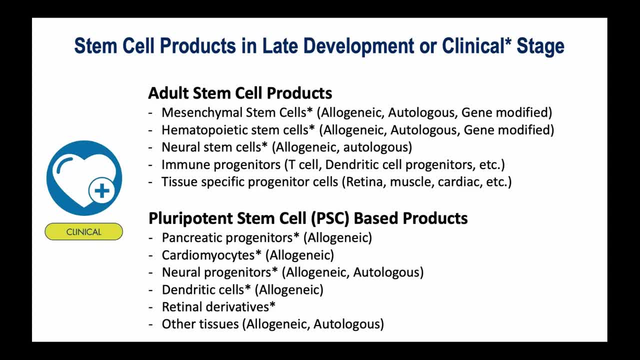 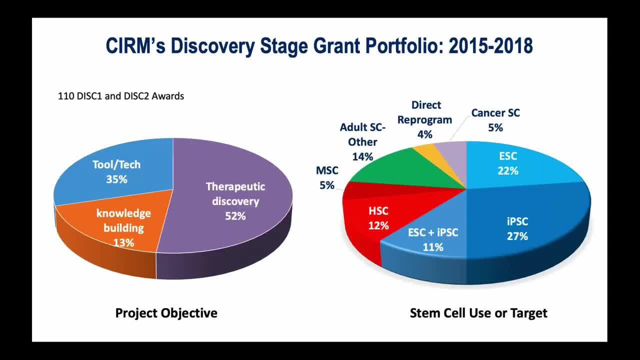 ago is getting ready to a stage where these questions and challenges are a reality And they need to be addressed now. Next slide, please. So this is just a snapshot of some of the earlier stage projects that CIRM's been funding over the past five. 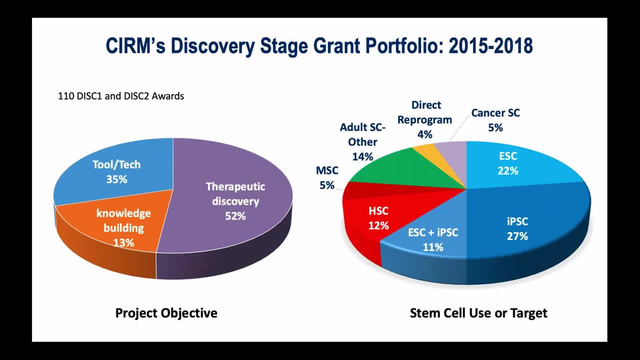 years or so through our candidate discovery program and our hypothesis testing program, which we call DISC-1 and DISC-2.. So you can see on the left that about half of our projects are dedicated towards trying to find a therapeutic candidate, either from stem cells. 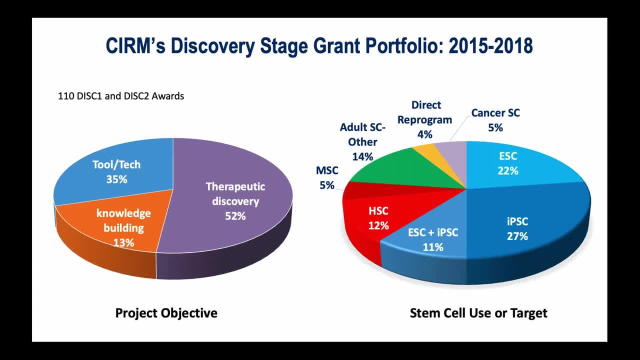 Or that can be discovered through the use of stem cells. We still send a fair amount of projects doing basic knowledge building, hypothesis testing, And about a third of our projects are devoted towards developing stem cell-based tools or technologies or, as I said, imaging technologies. 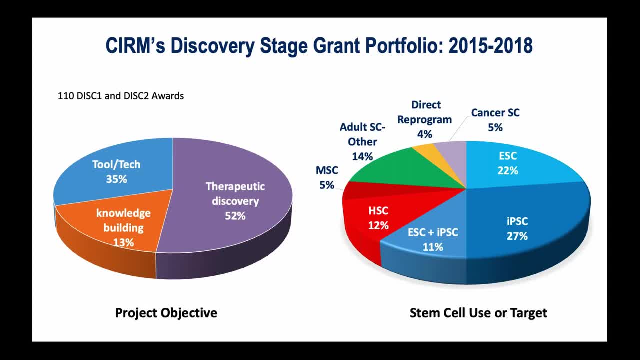 that can be enabling for the stem cell field. Although the majority of our early stage programs are still focused on pluripotent stem cells, primarily embryonic stem cells induce pluripotent cells. Pluripotent stem cells are using both. We do have a fair amount of projects. 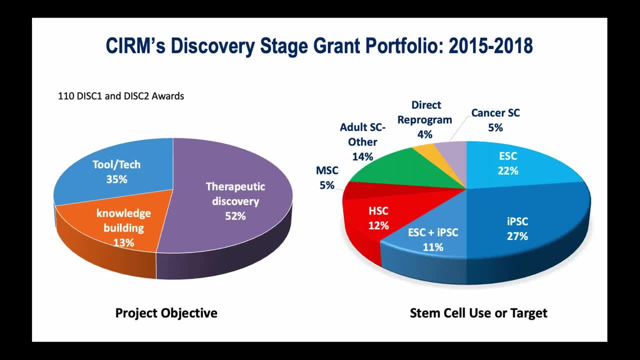 looking at hematopoietic stem cells and a whole variety of other adult stem cell types, And we also have some projects who are looking at direct reprogramming, which is skipping the pluripotent stem cell step and trying to convert one differentiated stem cell. 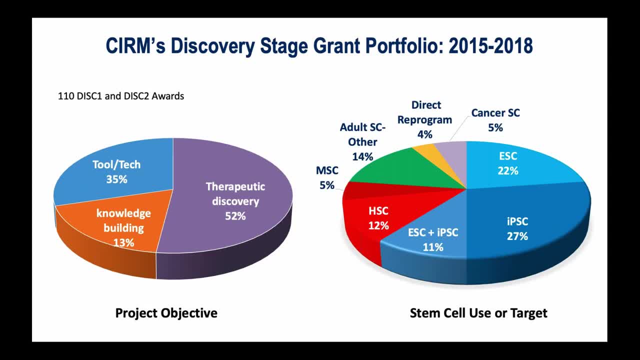 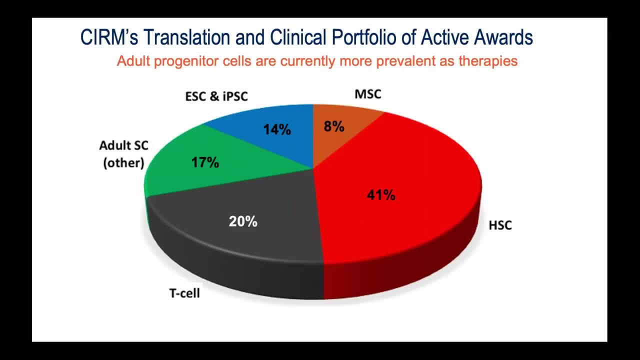 type into a different fate to sort of avoid some of the challenges that come with working with pluripotent stem cells. Next slide, please. As we move down that pipeline, as you can see our translation stage, we still fund a fair amount of pluripotent stem cells there. 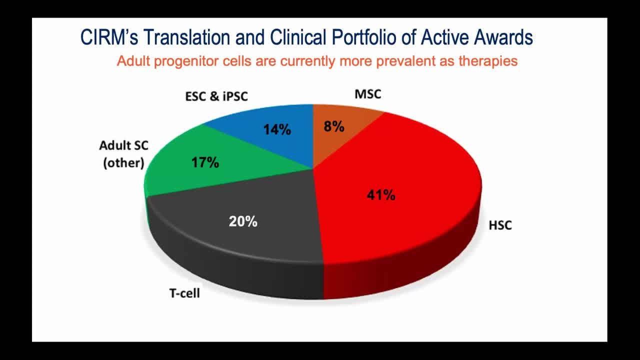 Again, these are projects that are engaged in studies that will allow them to bring a package to the FDA for discussion. Now you can see that a good portion of these are hematopoietic stem cell projects, But these aren't just your ordinary bone marrow. 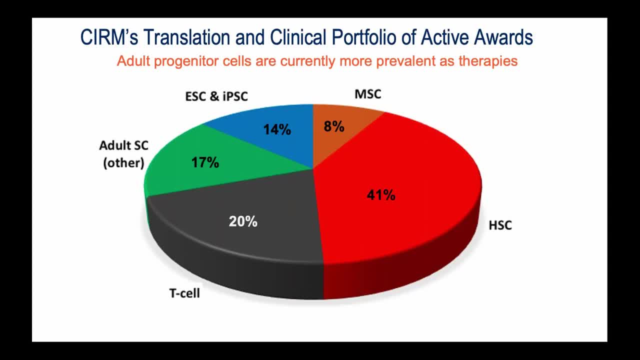 transplant. These are gene-modified hematopoietic stem cells, So CRISPR-Cas9 edited or lentiviral modified. So these are kind of the next frontier of stem cell biology. So there are also a lot of challenges to be worked about to get efficient editing. 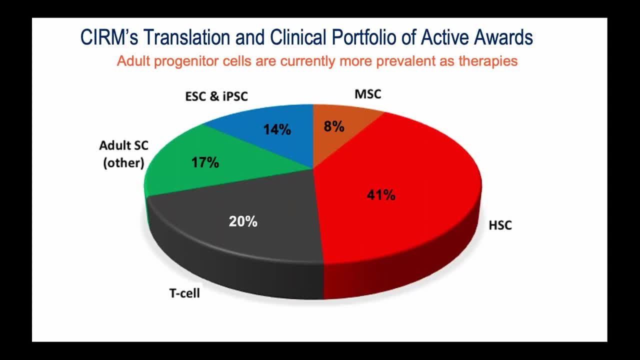 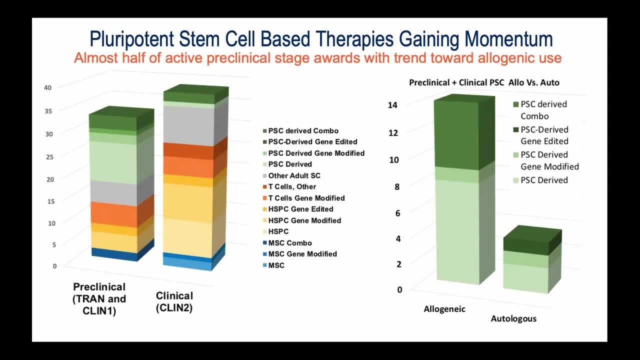 of these stem cells so that they can be used in a safe and practical manner. Next slide, please, And this is the last slide I'm going to share before I transition to Steven, Because what I want you to see is that there really is a lot of momentum in our field building. 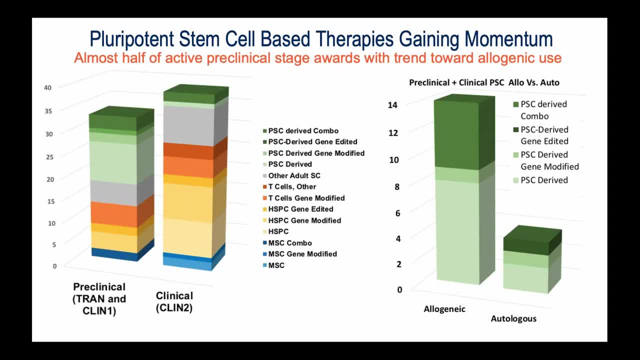 for the pluripotent stem cell-derived therapeutic products, as well as what I just alluded to, gene-modified versions, And what I mean by gene-modified is that we're looking at a lot of these versions of established stem cell products, such as hematopoietic stem cells. 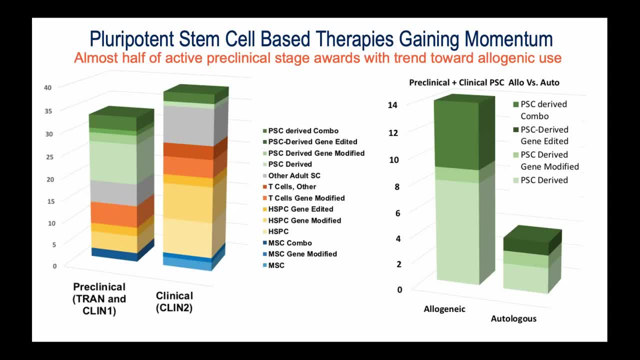 But, as you can see, from this kind of green coloring and on the right here, even these darker green colors here, that even a lot of the pluripotent stem cell products that we're finding are gene-modified And, as you can see, these are primarily 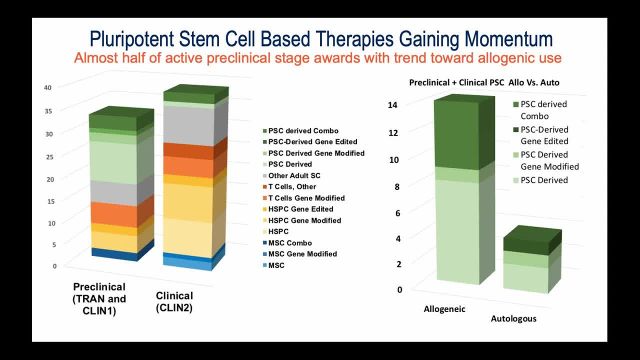 the allogeneic candidates, meaning donor-derived, And, as you can imagine or you might guess, a lot of that gene modification is an attempt to make a universal cell product, something that can be used by people with different immune backgrounds. Now you've talked a little bit about manufacturing cell. 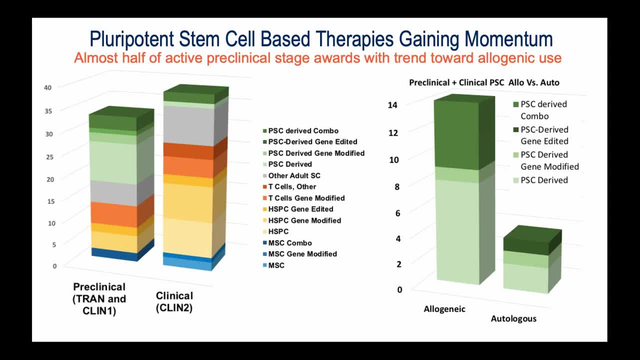 therapies in space, And I think that probably makes the most sense for a product where you could produce a bunch of it and bring it back and have it be an off-the-shelf therapeutic. So figuring out how to create immune-compatible cell types. 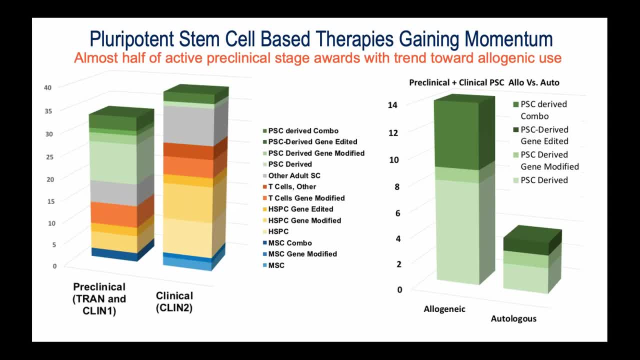 that could be manufactured safely and effectively and inexpensively is going to be something that's going to be something that's extremely valuable for the field as a whole. So I think from here I'm going to transition to Stephen now And he can give you a few more concrete examples. 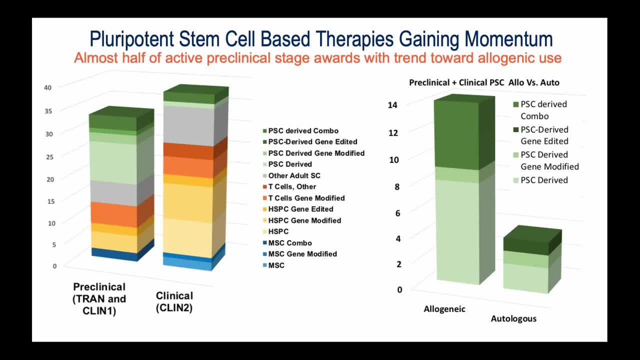 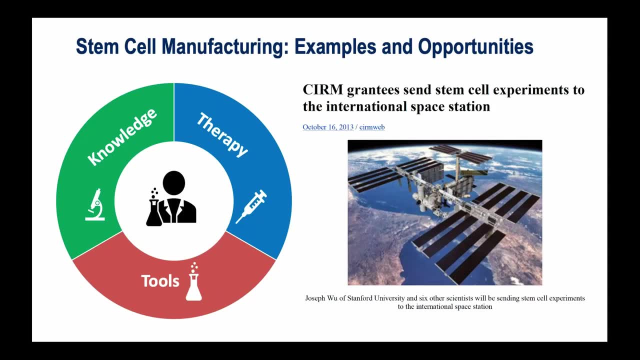 of some of what I've just shared with you in our overview. Great Thank you, Kelly. Can you advance to the next slide? OK, So, as Kelly described, CIRM has established a pipeline of awards that span from basic research and discovery. 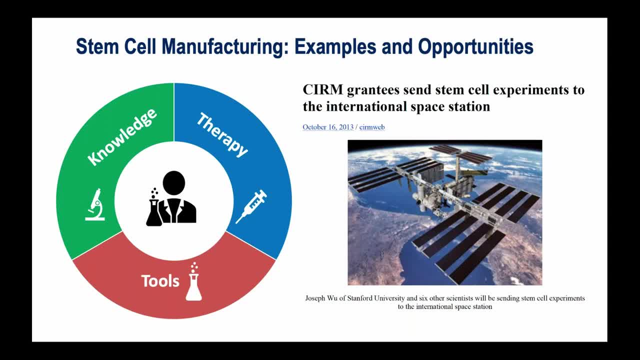 to clinical stage programs, And so I'm going to describe several examples of CIRM investigators that are developing therapeutic products at different stages in CIRM's pipeline, But they've also conducted projects aboard ISS or are planning to do so, And actually there's some overlap. 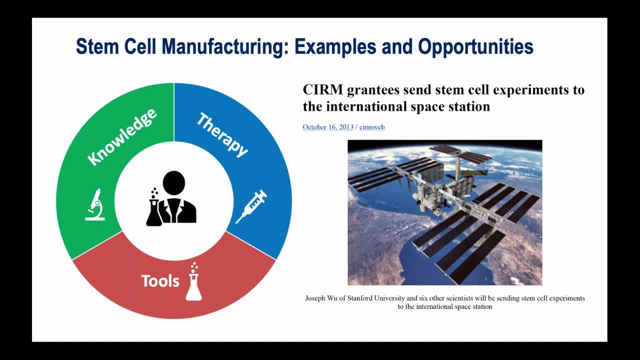 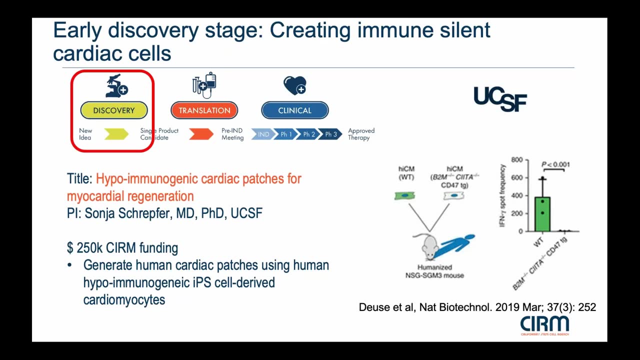 from the previous presentations to some of the examples I'll give, And so I'll also describe some scientific questions related to space research that we've seen arise from the programs that we've supported at CIRM. Next slide, please. So beginning with our discovery stage awards. 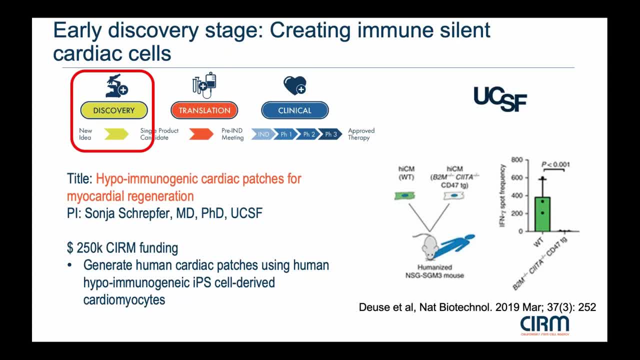 Sonja Schreppfer at UCSF had a project to develop hypoimmunogenic cardiac patches from iPSCs, And so one important hurdle that has always existed with cell therapies is rejection of the graft by the immune system. So we've had several CIRM projects. 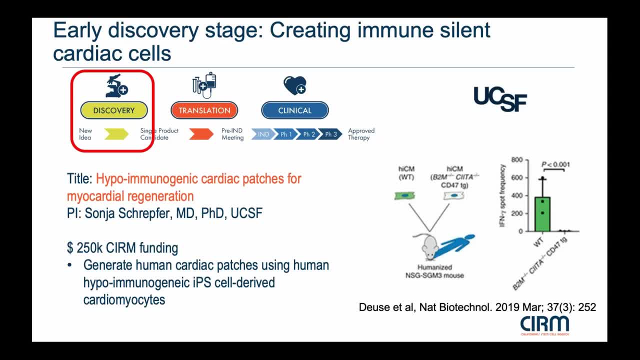 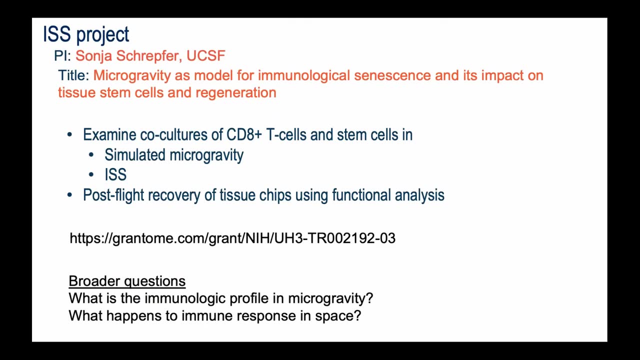 that attempt to engineer cells to evade the immune system, employing different methods to protect the cell therapy from B cells or T cells and the innate immune system. Next slide. So Sonja Schreppfer also has a project with a board that will go to the ISS. 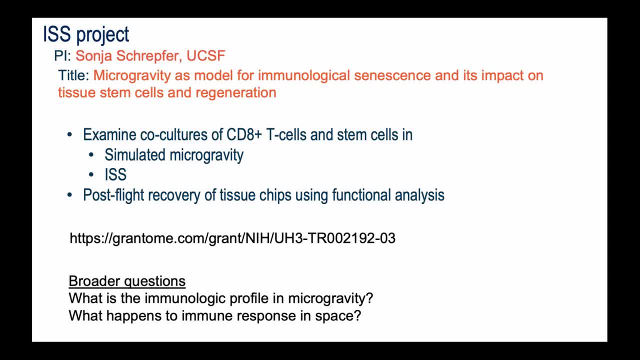 She has a project to look at the effect of immunosenescence from CD8-positive T cells on mesenchymal stromal cells as a model for bone healing and endothelial progenitor cells as a model for vascular regeneration. So microgravity is a model for aging in this case. 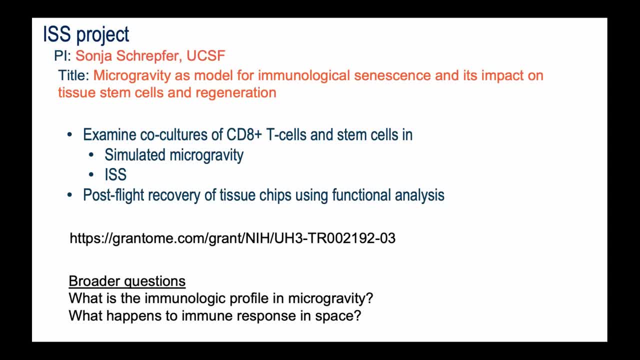 And the hypothesis is that in microgravity there will be an increase in terminally differentiated CD8-positive affected memory T cells and that can impair stem cell-based health in tissues. So these experiments set up broader questions that you may ask in space, including. 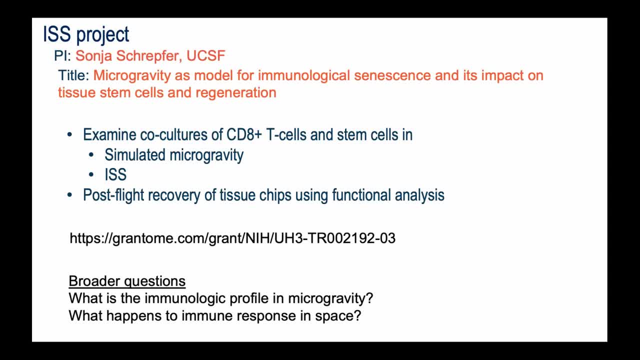 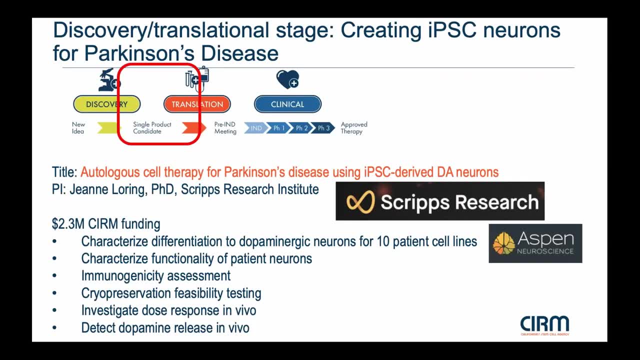 what is the immunogenic profile in microgravity, or what happens to the immune response in space? Next slide. So Jean Loring at the Scripps Institute in Aspen Neuroscience had a later stage discovery award to make an iPSC-derived dopaminergic neuron. that's. 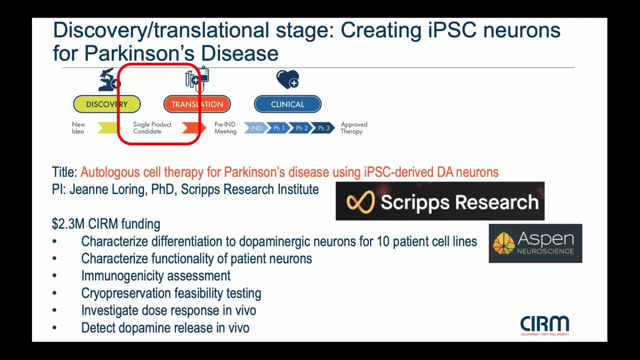 ready for translation. So this is an autologous therapy and she was doing many of the studies in her CIRM award that were needed to establish reproducibility of the product, including establishing differentiation- the dopaminergic neurons- for 10 patient lines. 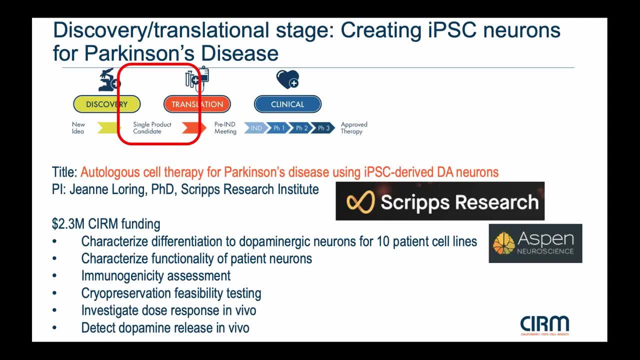 determining the functionality of those patient neurons, assessing the immune response of that product, looking at cryopreservation and then looking at dose response and dopamine release for function in vivo. So a lot of the product attributes that Kelly touched on. Next slide. 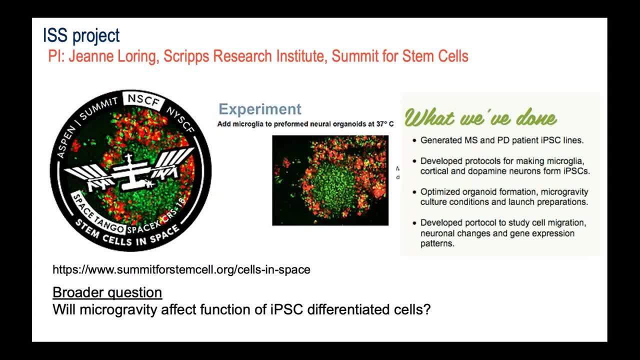 So, in partnership with the New York Stem Cell Foundation and SpaceTango- as Janice Sudemeier, who's going to be talking to you shortly- we have a new product that we're going to be described and also the Parkinson's Disease Patient Advocacy Group Summit for Stem Cells. 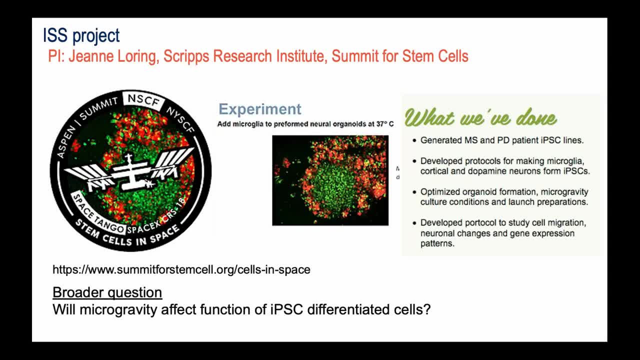 several of the iPSC lines that were created from Parkinson's disease patients are going to the ISS, So neural organoids will be created from the patient iPSCs to determine how microgravity affects their migration, neuronal changes and gene expression pattern, So deriving mature cells. 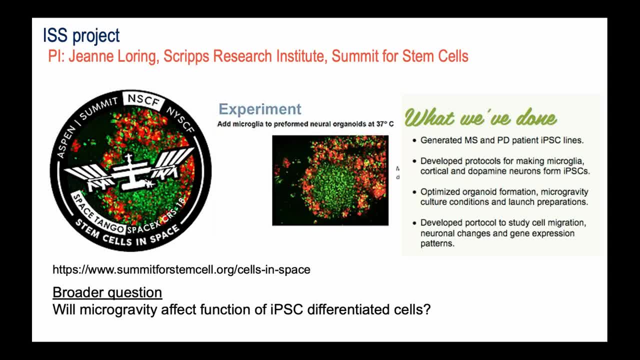 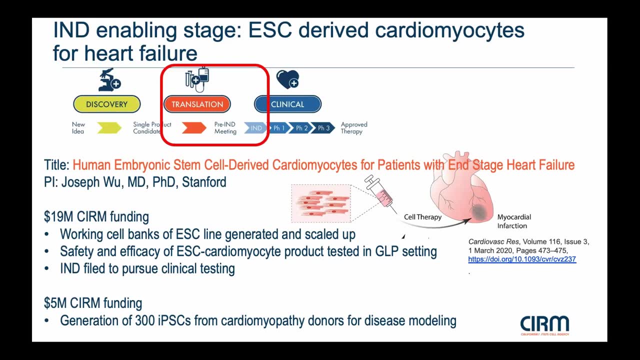 from pluripotent stem cells has long been a challenge in the field, And so a broader question is whether microgravity affects the function of iPSC-differentiated cells such as these, or could possibly improve them Next slide. So Joe Wu at Stanford has been supported by several CIRM awards, including a disease team. 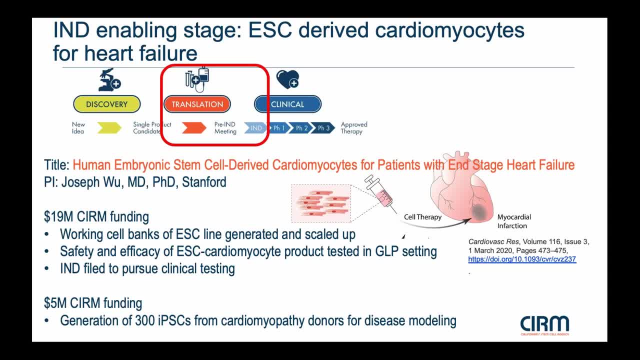 grant to get embryonic stem cell-derived cardiomyocytes scaled up and tested for clinical gli miteinander, And he's also been prizewан for a number of paid services, including a grant to get embryonic stem cell-derived cardiomyocytes scaled up and tested for clinical 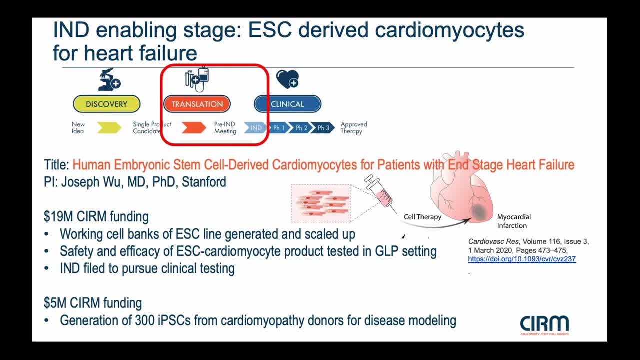 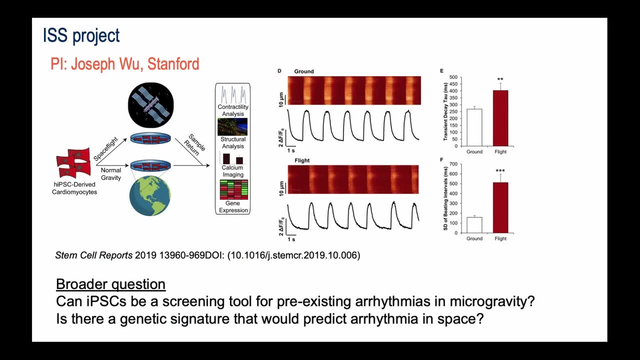 for a clinical trial and a research award to create a bank of ipscs from cardiomyopathy donors for disease modeling and and drug screening. next slide, and so his group has built a large ipsc collection of cardiomyopathy samples and, uh, this is a project. 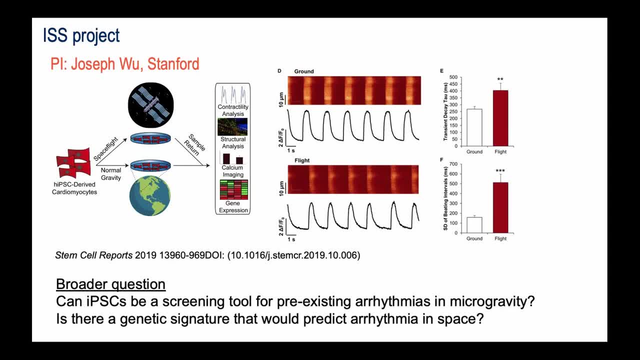 um that the previous speaker, dr arun sharma, described when he was uh in in dr wu's lab um looking at ipsc derived cardiomyocytes that were sent to the iss compared to their effects on on normal gravity, and he went through the data much better than than i could. but 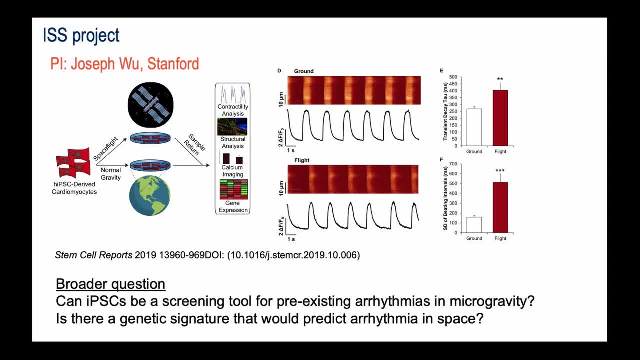 there were. there were some differences between the cells that were sent to space and the ones that were left um and regular gravity on on earth, including some hints of uh, possible differences in beatings, um and and arrhythmias. so one one question is whether stem cell models like this could predict human health with long-term space travel for. 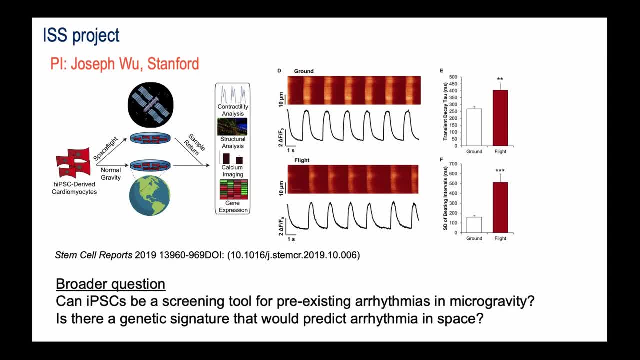 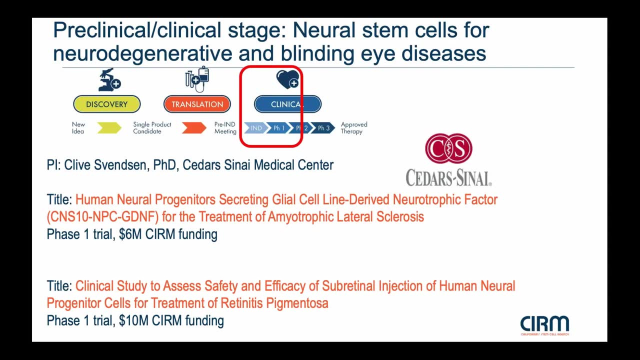 example, could they be used as a screening tool to predict whether a person is at higher risk for heart arrhythmias in space, and is there a genetic signature that could be associated with that next slide? and so in one final example of a stern funded investigator is dr clive. 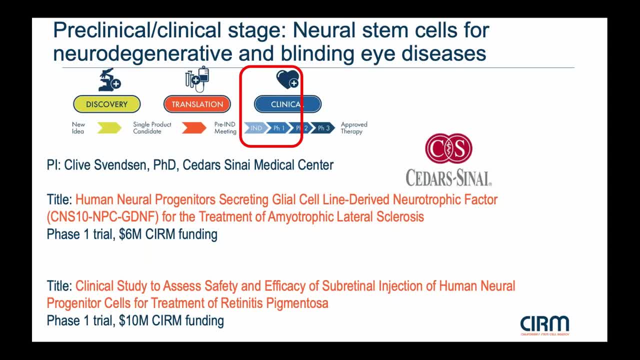 spenson from cedar signing medical center. he's funded uh by cern for multiple clinical trials uh using stem cells. uh one trial involves using human neural progenitor um line that expresses the neurotrophic factor gdnf to treat amyotrophic lateral sclerosis, or als. the other trial uses the unmodified neural progenitor lines to treat 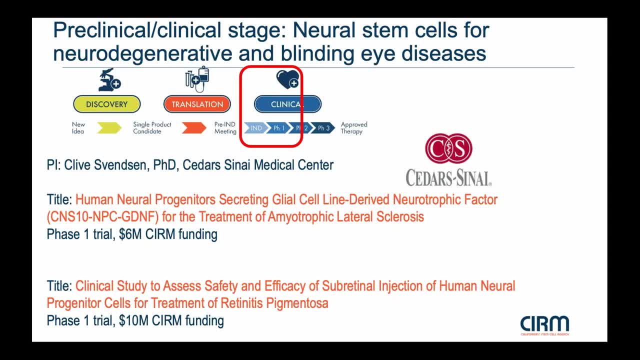 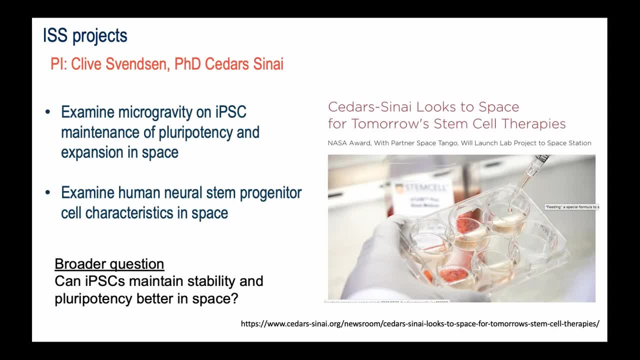 the eye disease, retinitis pigmentosa, next slide, and so the group plans to send two types of cells to the pscs in partnership with space tango: the, the gdnf neural progenitor line used for the als trial, and undifferentiated ipscs and uh. both um janice sudomiro, space tango and uh dr sharma are 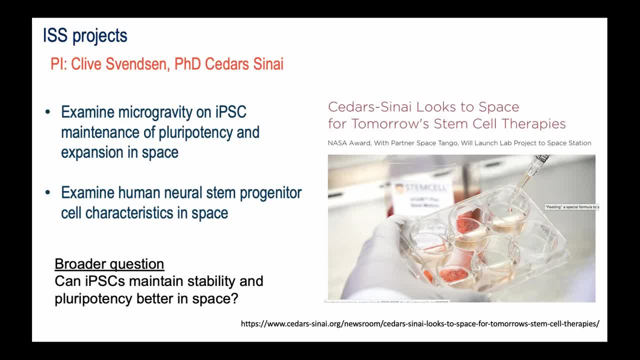 probably involved in these projects. so one one challenge with psc manufacturing is to maintain the stability of of the cells with passage and expansion, so pluripotent stem cells can lose their uh potential and they become- can become stereotypically unstable with prolonged culture and expansion. however, expansion is critical for many psc drive therapies to set up. 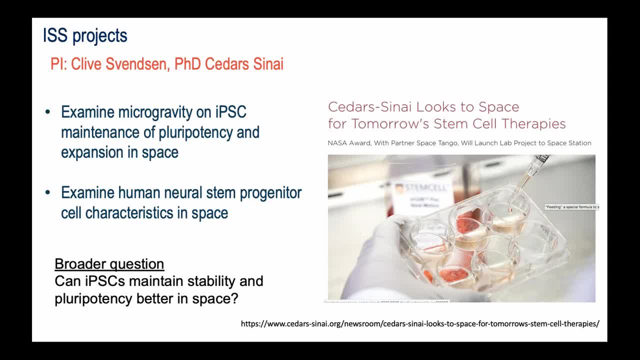 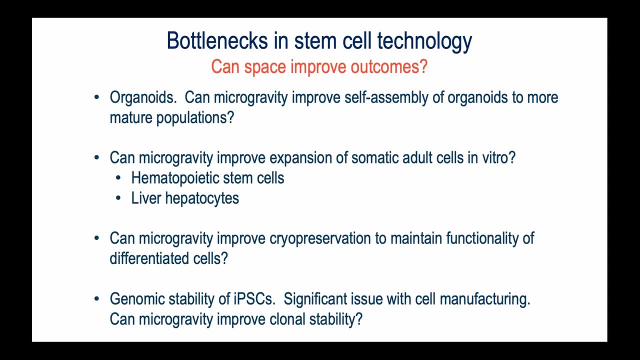 working cell banks so that you have enough to go into the patient, and so one question is whether these characteristics can be better maintained in space next slide. so these are some examples of serum. investigators that have studied various aspects of stem cell biology and space in connection with their translational and clinical efforts on birth at cerm, we've encountered 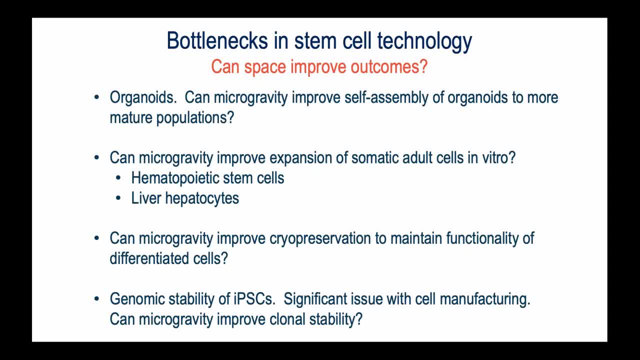 many other bottlenecks over the years with projects that we've supported- kelly has touched on a lot of them, but other other bottlenecks that we we've seen that perhaps space could address our organoids when organoids are put together, and usually they are still in a fairly immature state, and so the question is, if you assemble the 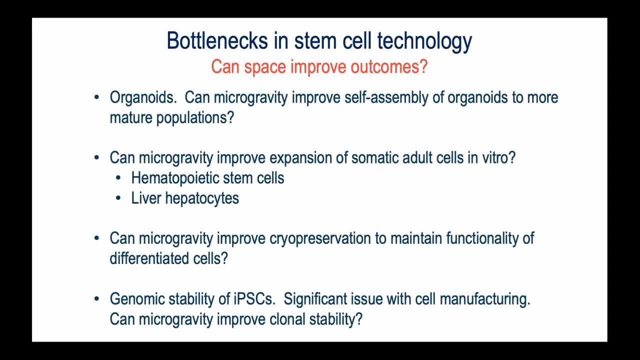 organoids in space? can the? can the, the self assembly of organized, create more mature populations or different populations than you could see on earth? another challenge that we see on earth is is is the bottleneck in expanding somatic adult cells in vitro, So hematopoietic stem cells or liver hepatocytes. they either self-renew or they can regenerate in the body, and that's one of their characteristics. 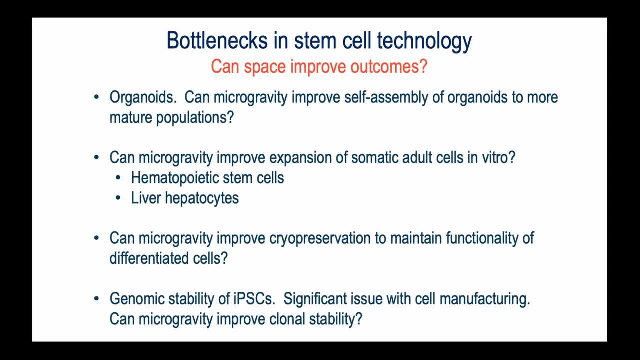 Interestingly, when you take them out and you try to grow them in culture, they act like they're quiescent. They really do not expand and it has been a challenge for decades to get them to do this. The question is: can, if you put this in a microgravity environment, can you adjust the conditions to allow them to do this? 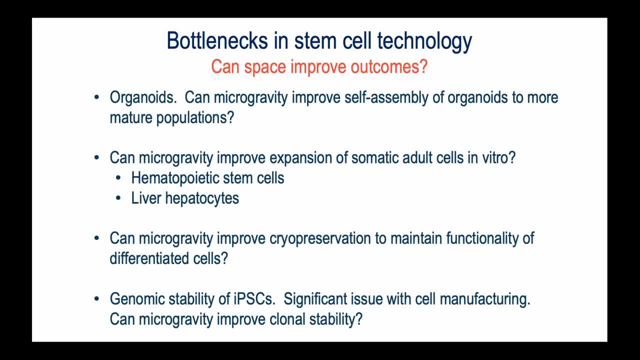 Also cryopreservation. So cryopreservation is a significant issue with cell manufacturing for your product. You want to cryopreserve the cells to make the cells more feasible for distribution And transplantation, But there is a drawback in that cryopreservation also often leads to a loss of functionality. 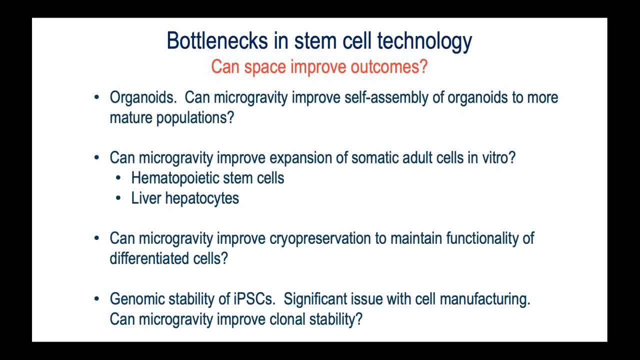 And so if you can adjust the cryopreservation conditions in microgravity, one question is whether it could overcome this loss of function that you see on Earth. And then the final bottleneck. there are several, many, many other bottlenecks, but the final one that I'll just mention. 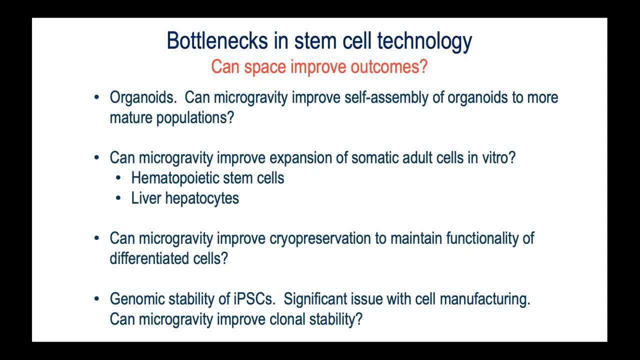 And the final one that I'll just touch on is genomic stability with iPSCs, which we heard of, which I described at the last example with Cedars-Sinai. So this is a significant issue with cell manufacturing and it will be interesting to see, with this Cedars project, if microgravity can improve that clonal stability. 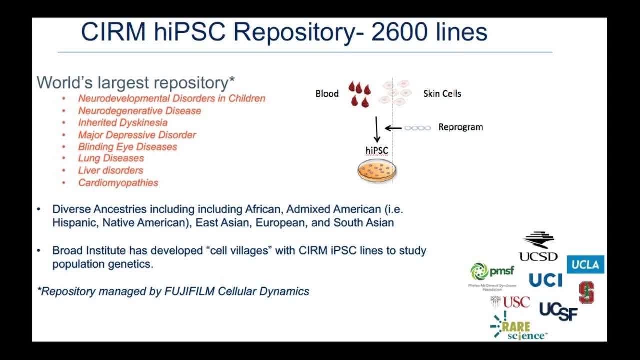 Next slide. Next slide. So another reoccurring issue that we see is that phenotypes can vary significantly Among cell lines. So one cell line may respond very strongly to an experimental condition and another may not have any effect at all. 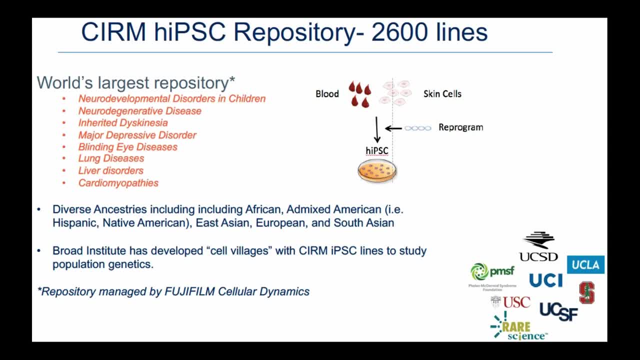 And so with PSC lines, some PSC lines differentiate to certain tissue types better than other lines and it's really not known why. So looking at cell line variability is very difficult aboard the ISS because, as was described very well by Janet Sudermeyer, 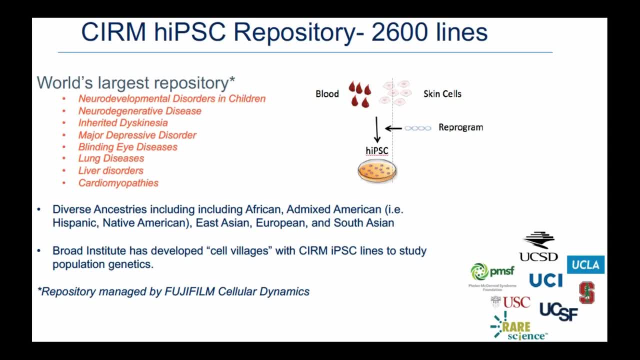 there are very tight confines. So, in addition to funding research investigators with the examples I described, CIRM has also created resources that exist that assist the entire scientific community, and this is part of our infrastructure pillar of programs. So one of the resources that we've established is an IPS bank, and this IPS bank is currently the world's largest collection of publicly accessible iPSCs. 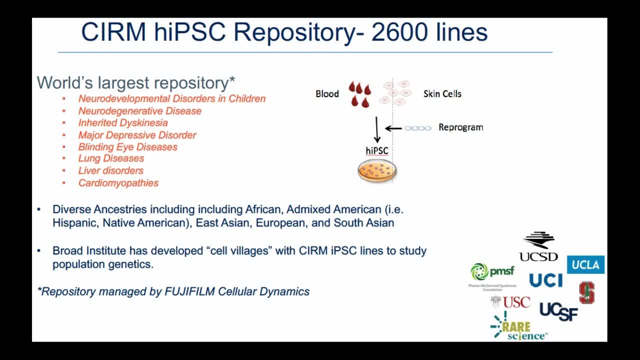 within the United States, And it's also one of the most diverse, with lines represented from African, Hispanic, East Asian, South Asian and European ancestry. So the cell repository is managed by Fujifilm Cellular Dynamics And several years ago CIRM and Fujifilm began a partnership with the Broad Institute in Massachusetts to utilize the breadth and diversity of the collection to create pools of stem cell lines termed cellular dynamics. 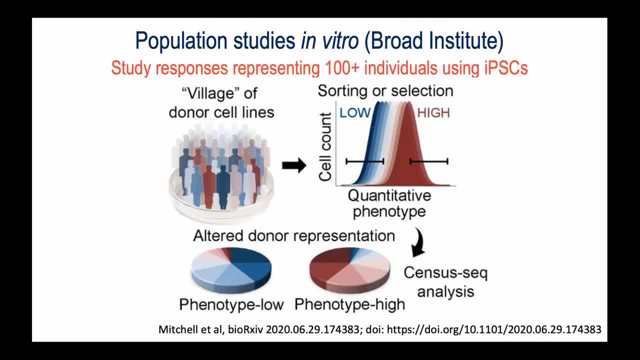 And that's a really, really, really cool tool. So that's a really really cool tool. villages Next slide, So in the system that the Broad established up to 100 lines can be pooled in a single culture and later stored for a specific phenotype, So using natural variations. 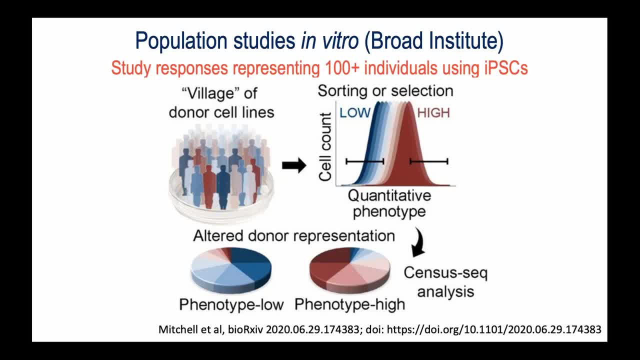 in genomic sequences as barcodes, individual cells can be identified that have low to high phenotype characteristics, and a new analysis technique that they developed, called SensiSeq, can profile rare alleles that are associated with the phenotype. So the proof of concept experiments for this approach map the effects of several alleles on drug responses for spinal 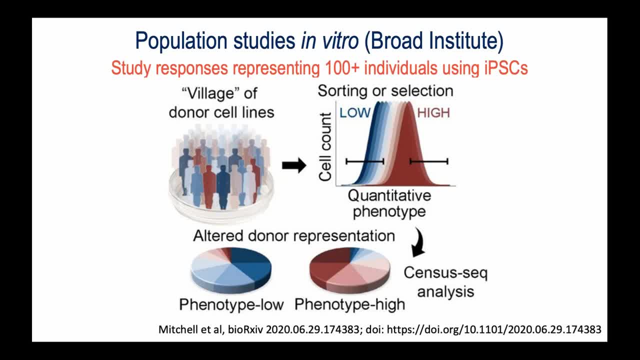 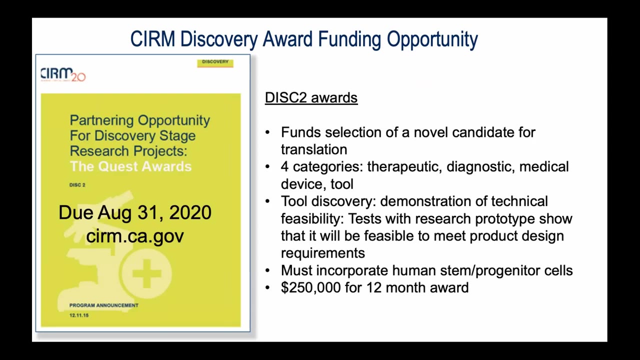 muscle atrophy. And so, because this technique enables population-scale experiments in very small pools with high internal control, one could see it being utilized eventually aboard the ISS to examine genetic effects of diverse phenotypes in a confined compartment. Next slide. And so this is the final slide that I'll go over. As a funding agency, CIRM- wants to. 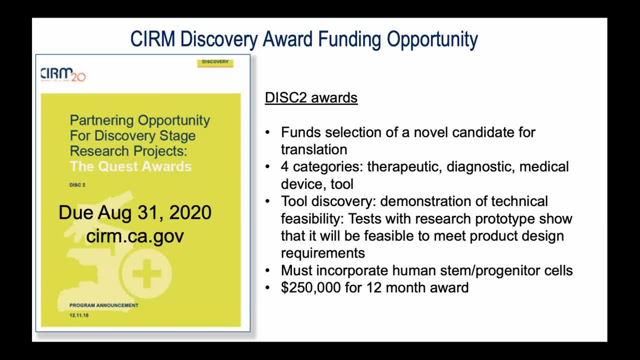 support stem cell technologies to advance its mission And if there are organizations in CIRM that are in California that are developing tools that utilize stem cells for the ISS, the agency has a single funding opportunity this year to support it, As Kelly talked about. 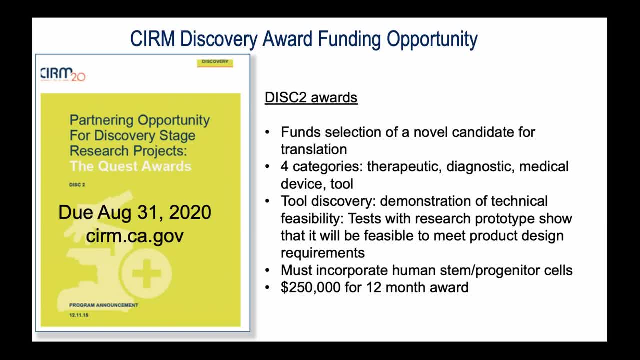 Discovery Tool Awards will support. This is a tool discovery that will demonstrate technical feasibility in a research prototype. So the tool must be used human stem or progenitor cells, but otherwise it's fairly open. what you can apply for This award is $250,000 for 12 months And if you're interested, 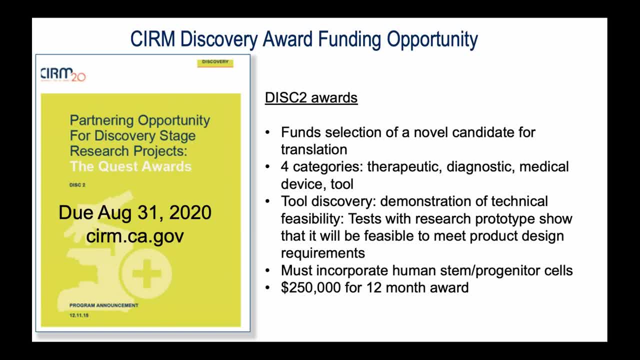 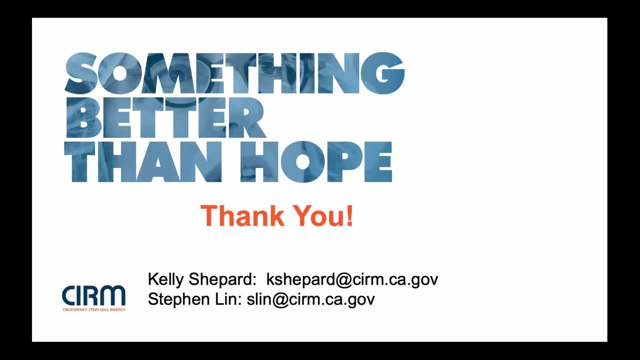 the deadline for these DISC-II awards applications is August 31st And more information can be found on CIRM's website, cirmcagov- Next slide. So if there are any questions, please feel free to ask Kelly or me at the information. 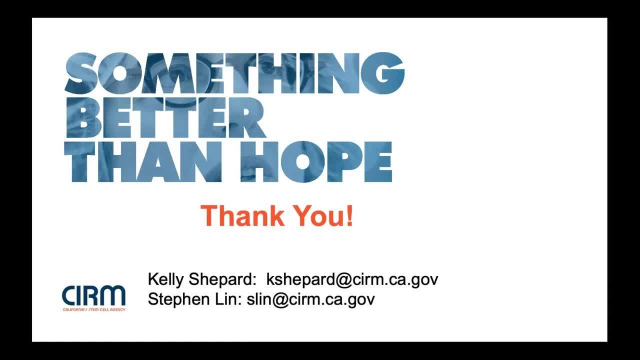 on this slide. Thank you very much for your attention, Kelly Johnson, Thank you, Stephen and Kelly. That was fantastic. I'm sure the entire community appreciates CIRM's support And you also did a really, really nice job of kind of encompassing what a lot of the question posers are asking, which. 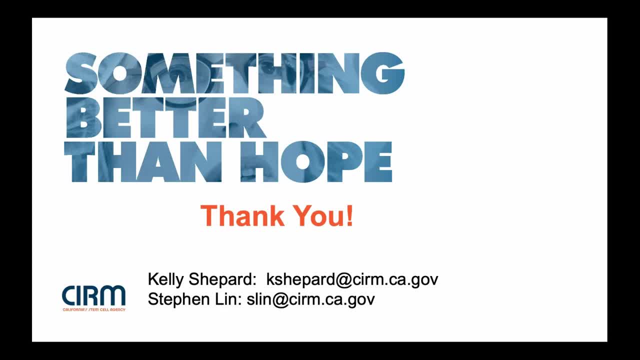 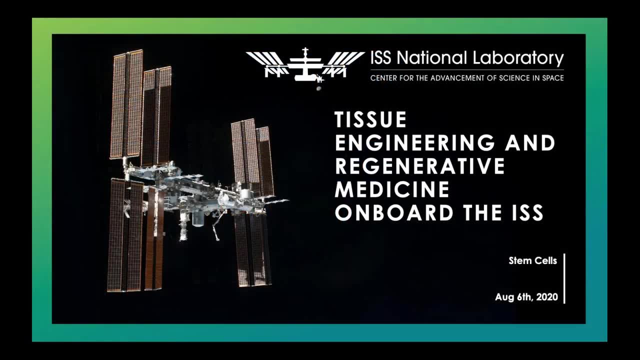 is why microgravity may be able to address some of these very basic questions and enable breakthroughs. So if everyone else will, please turn on your camera so that we can engage with our audience. We've got a number of questions. We're a little short on time, So if possible, we'll kind. 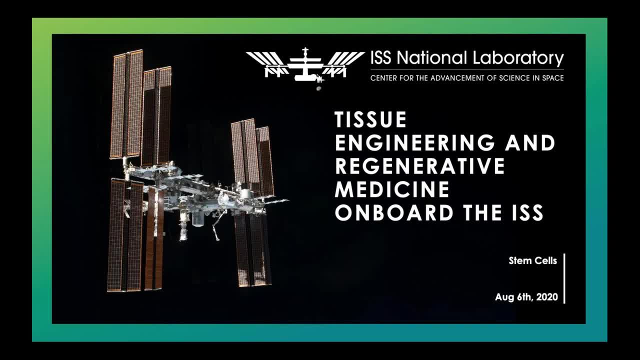 of zip through some of these, We won't be able to get to everyone's questions. I apologize for that. There are a lot of them, Kelly Johnson. Okay, And I want to remind everyone that this webinar will be available on the CASES website, probably. 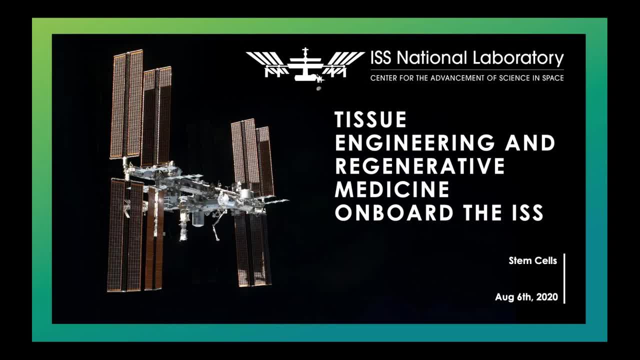 in a couple of weeks we'll get the recording there issnationallaborg, And okay. so first question- I'm going to go back to Dr Zubair, Regarding stem cells in microgravity, could the response, the immunosuppressive response- of stem cells be related to adaptation? 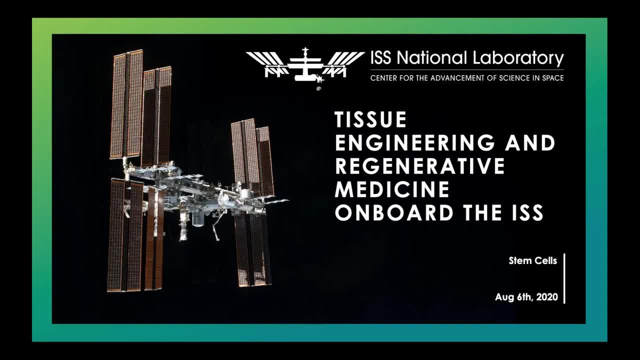 to spaceflight And second part of that, are there benefits to that immunosuppressive potential that could translate to clinical use here on Earth? Yeah, that's a very good question. It's hard to say it's adaptation alone. I think there is more to it. 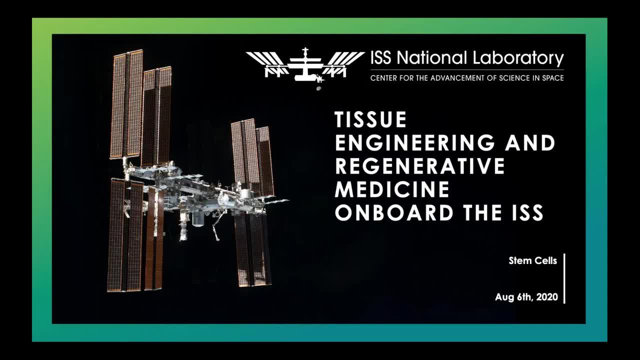 Because so when the cells return back to our lab, I mean that's when we assess their immunosuppressive activity, So probably while they are in space they may not be as much, So the evaluation is done at Earth's gravity. 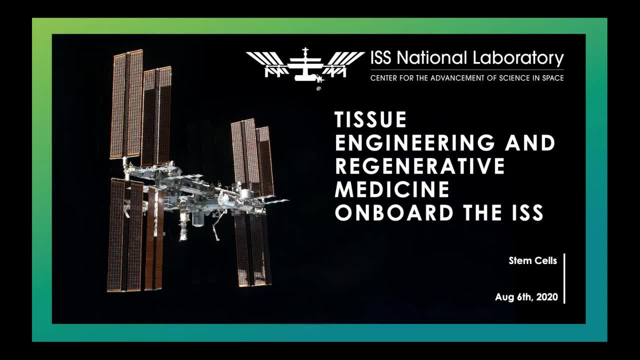 That means, yeah, it could be that something they acquire as an adaptation, But clearly that is maintained beyond the microgravity. But again, more to be done. Obviously, as you all know, one experiment doesn't cut the chain, So 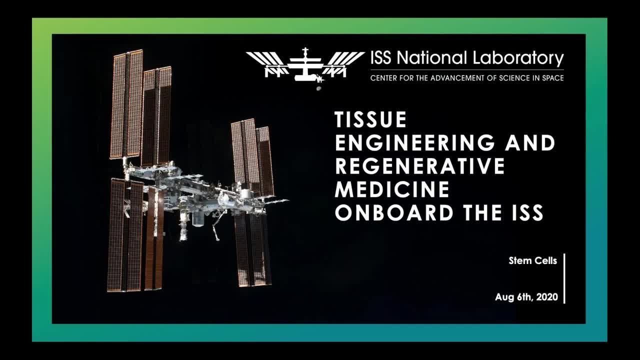 Well then, let me add a follow on. If you were to conduct a follow on experiment Abba, what kind of an additional experiment would you like to do that would kind of improve on or build upon your results already? Absolutely. The first one is the question that was raised. 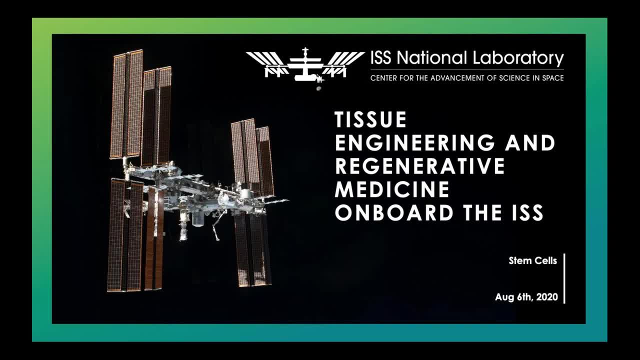 Is MSC mesenchymal stem cell more immunosuppressive in real time at ISS compared to the ground control? Obviously, we want to also to really go deeper into looking at T cell subsets, what T cells are impacted, and do real time analysis looking at T regulator T cells, even the cytokine that we assess. 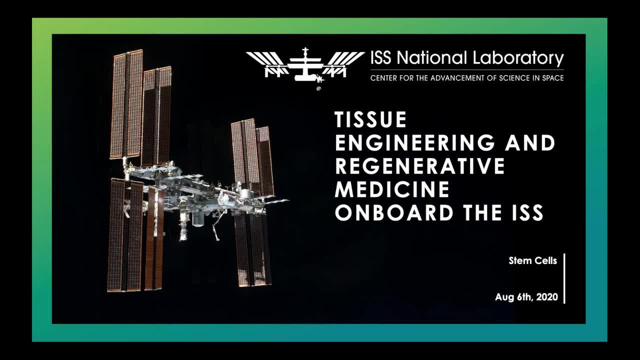 Of course, the cytokine condition media. So it's a snapshot of what is going on in space. because the cells were approached, the condition media was frozen In space but, if you noted so, like CD40, ligand is known to be immunosuppressive, but the level went down. 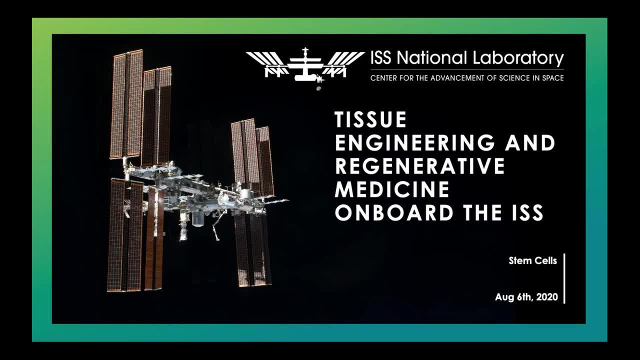 So it's kind of, of course, the immunosuppressive nature of the that we have, or even IL-10, which also went down. So There is more to be done and we would love to do real time analysis rather than post-flight analysis. 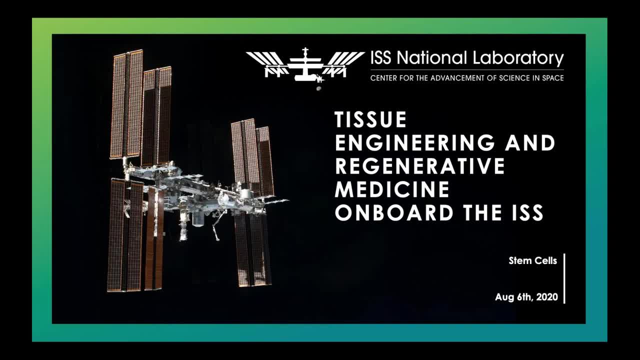 Okay, One more final question for you, Dr Zabair. Would you or have you considered using spheroids in your research, And do you consider that there's a possibility that the results might be different with spheroids? Absolutely. 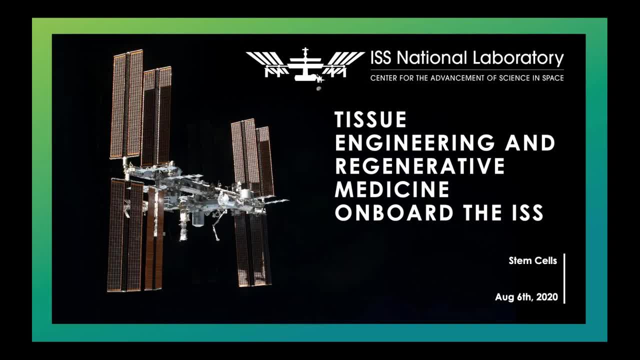 I think it would be different because with spheroids, you know it's, it's a very complex process. You know it's a multicellular environment and you can. that would be interaction of the cells, Obviously just having cells by themselves. we know in real life it's an ecosystem rather than single. 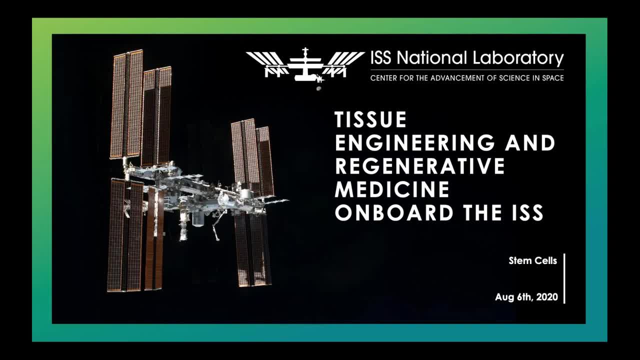 So yeah, absolutely spheroid is something that we would like to do. Okay, And a couple of questions for Dr Sharma Arun. did you have a question for Dr Sharma Arun? did you observe higher levels of de-differentiation of your human induced pluripotent stem cells in the space group when compared to ground? 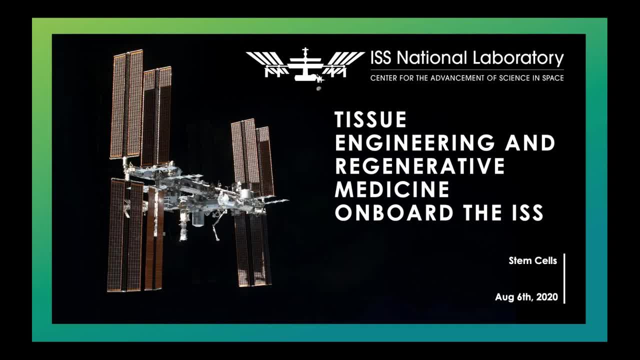 And how do those changes that you mentioned in the mitochondrial pathways correlate with maturation of the cardiomyocytes? And third, is it possible to pharmacologically recover the differences? And you're muted, sir. I'm sorry, I'm sorry, I'm sorry. 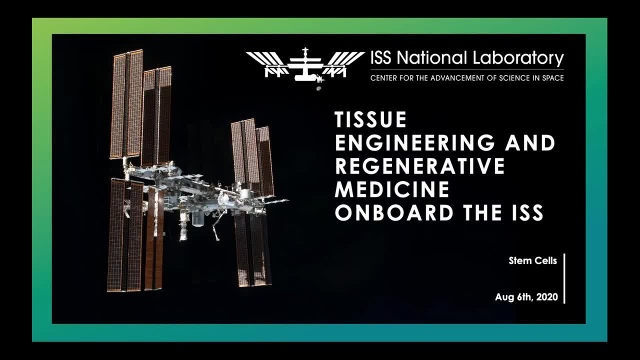 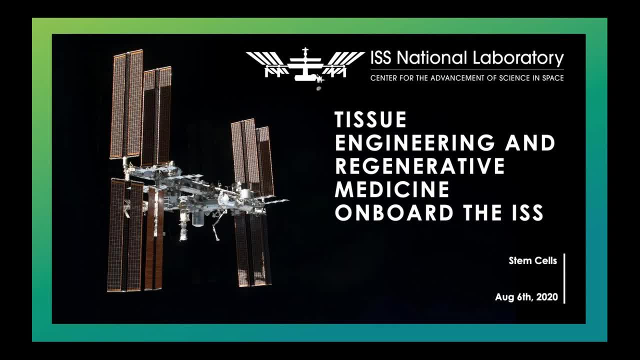 Okay, Can you hear me now? Yes, sir, Okay, So I'll see if I can answer some of those questions. Yes, So the question about de-differentiation, that's actually not something that we observed on the space flown samples. 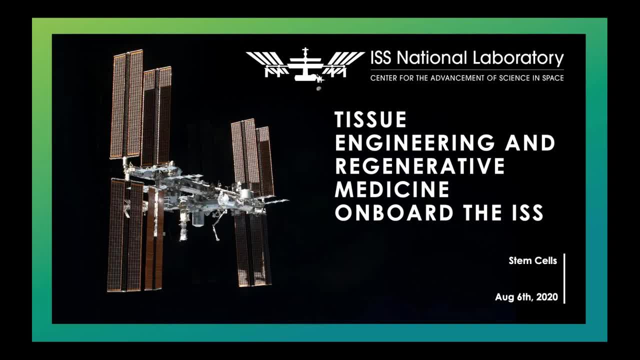 Of course there are plenty of other samples that are observed. So the question about de-differentiation, that's actually not something that we observed on the space flown samples. Of course there are plenty of other samples that are observed, other examples of RNA sequencing done on stem cell populations that have shown a more immature 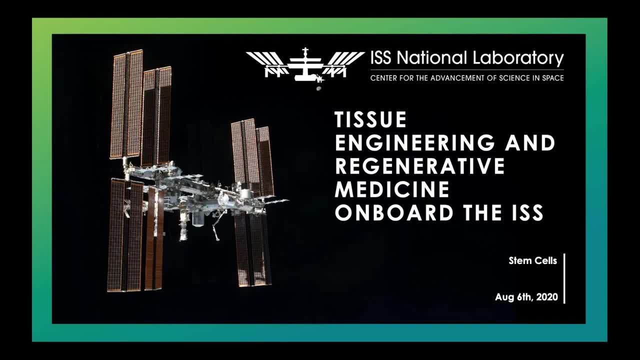 femur type of cells in microgravity. That's actually not something that we observed in our populations, perhaps because these cells are terminally differentiated, so they're months and months old. These are aged cardiomyocytes, but that is in a progenitor population. that would be. 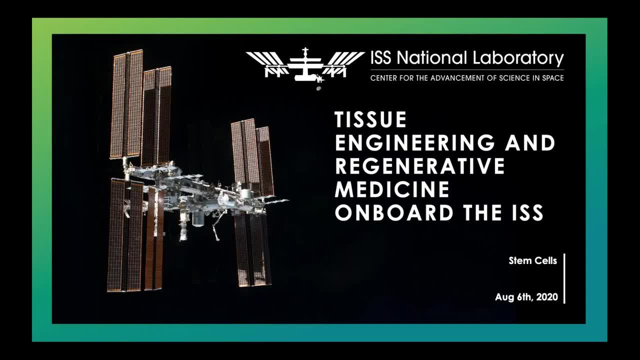 definitely a more relevant question. In response to a small molecule or something that would be able to mimic some of these effects. yes, I think that is an absolute natural next step. You want to be able to harness some of these biological phenomenon that microgravity might be able to. 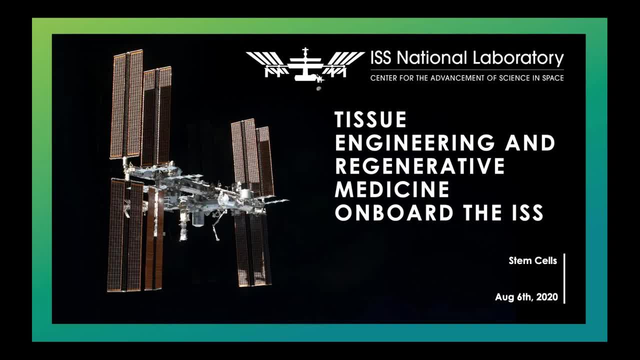 elicit and distill them down to a small molecule format, because that is ultimately something that's very translatable. If you can take some of those observations, some of those discoveries from the microgravity environment and actually replicate them on a ground-side level, I think that that would be a tremendous use for commercialization. 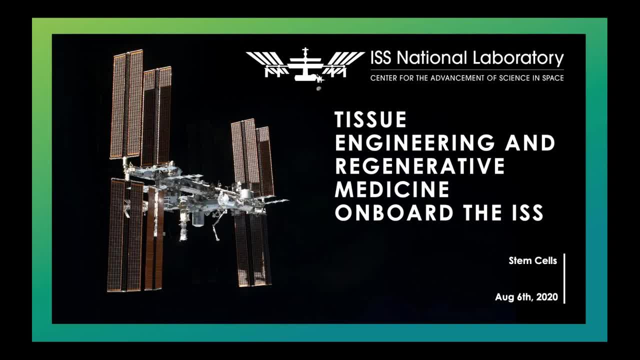 in a small molecule approach is, of course, a good way to do that. Okay, fantastic. Another question for you: How might the changes you saw in microgravity compared to those seen in patients- Patients in heart disease or congestive heart failure? 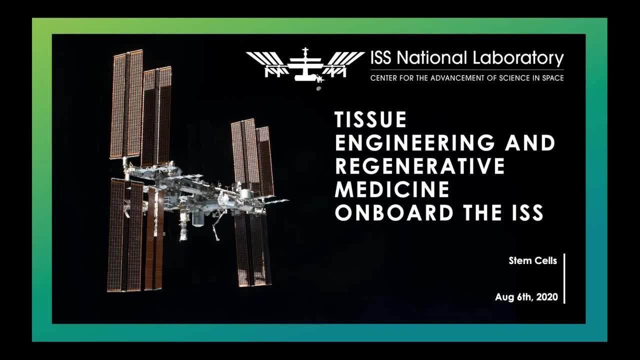 Yeah, so the changes that we're actually seeing in microgravity- and this is not even exclusive to the cardiac side of things- what you see a lot of times in microgravity is an accelerated aging phenotype right, And that is a lot of those same gene expression changes and functional changes. 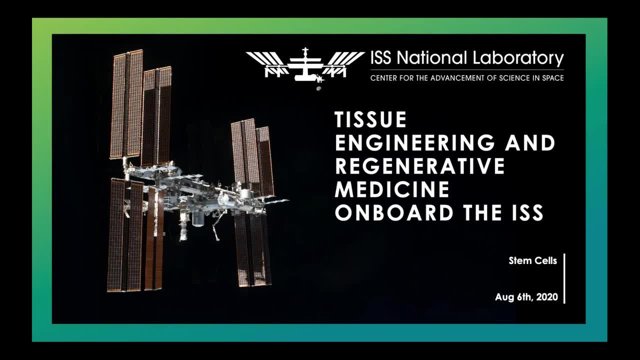 are seen in individuals With congestive heart failure. So there are parallels not only in the functional output of those particular, the functional phenotypes of those two diseases, but also in the gene expression levels as well. Very good, Let's see one other question, and I think you alluded to it, but did you find? 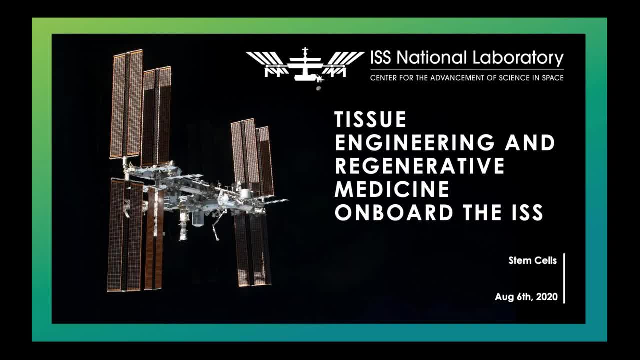 any alterations in the epigenetic regulation of your cells, which were cultured in microgravity? Yeah, That's a fantastic question. It's something that we want to address in the future And I think actually some of the follow up experiments are going to be focused on that. We actually did not. 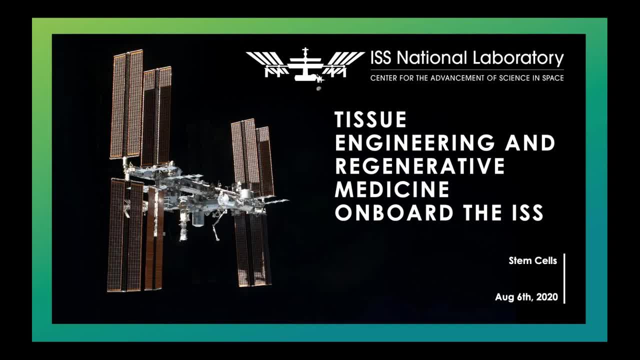 look at epigenetic regulation through, like ataxic and histone methylation those sort of things. But there are a variety of assays that have been developed, actually in the last few years, that would make this much more accessible, much more accessible now than it was when I actually 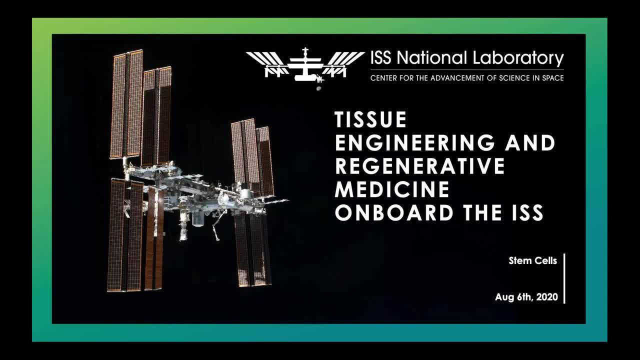 did this experiment four years ago. So that is a reflection on not only the questions that remain to be answered in the microgravity context, but in the technologies that have just been rapidly progressing over the last five years in stem cell biology. Indeed, Thank you for that answer and for that look ahead as well. 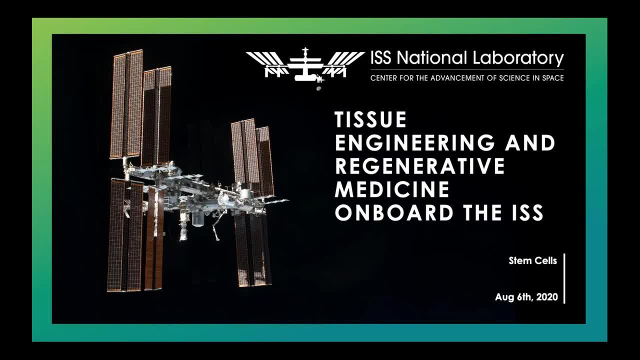 Quick question for Jana. If a researcher is interested in conducting experiments, experiments in microgravity, how do they get access to your system, your hardware, to see if there's compatibility? Sure, Yeah, I mean, we're available, obviously through our website and my email contact. I don't think I put up, but it's at. 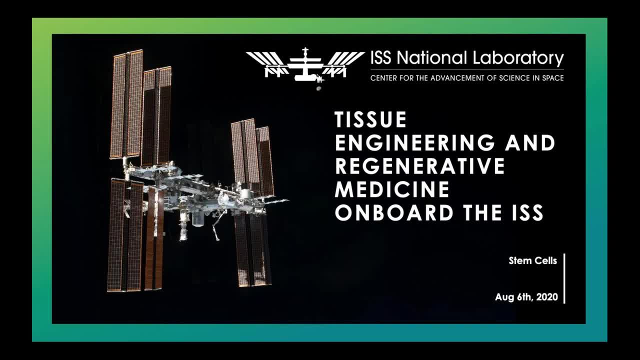 the end of my slides. So certainly feel free to reach out And we're very open to talking to all kinds of teams about the work that they want to do. It's so exciting to see the first experiment, the long-duration culture that was done by Joe Wu's lab with Dr Sharma right, I mean to me. 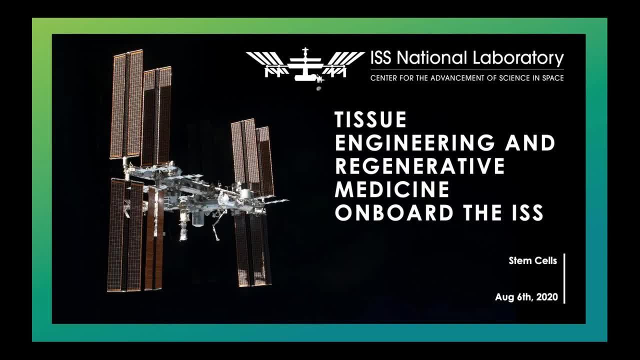 that was one of the seminal moments when I sort of came across from industry to microgravity and to watch the changes in the field and what's happening with the capabilities to support the more complex science on orbit. I just think it's a really exciting time to be able to try to answer. 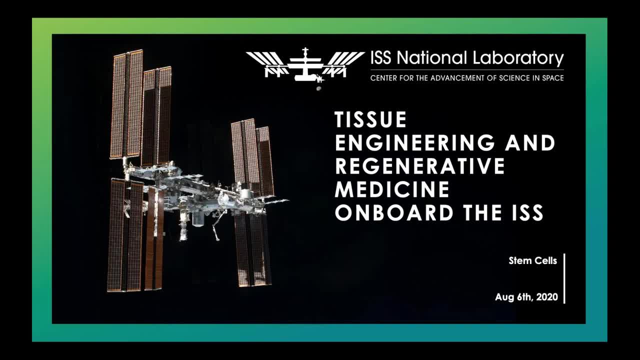 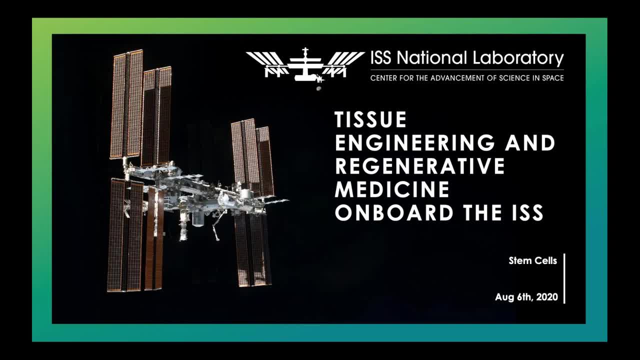 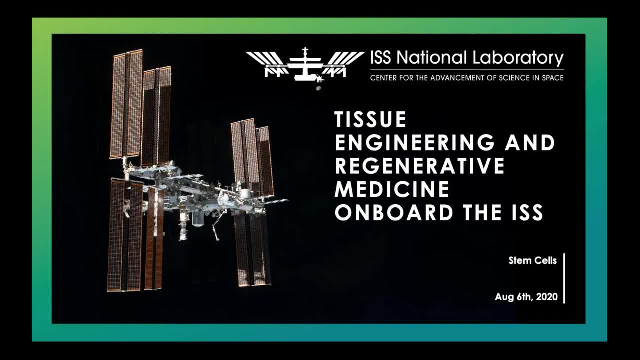 Thank you for your time, your dedication and your inspirational talks and with that I think we will sign off. Sorry we didn't get to any questions for Kelly or Stephen, but I'm sure there's some intrigue and interest with your potential funding opportunity that you might see. So thank you everyone. Thank you so much. Thank you, Bye. Thank you. 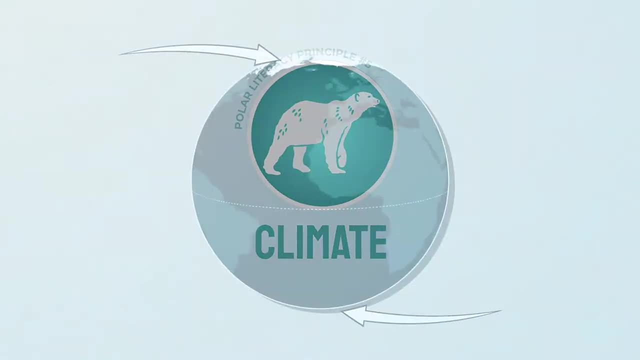 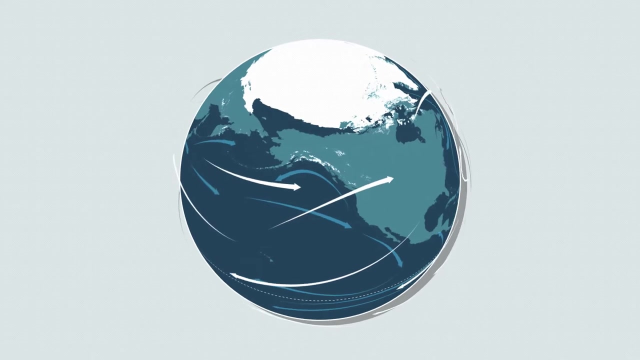 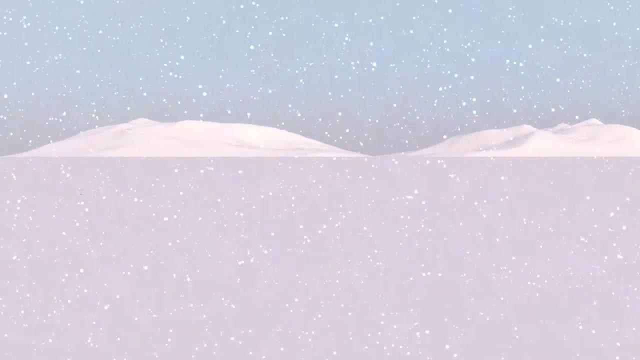 At the poles. climate change is affecting the environment faster than any other place on the planet. Warming air and water temperatures are impacting more than local snow and ice melt. Here are some basics Air. Warmer air holds more water, So a warmer climate means more precipitation in the form of snow and rain. 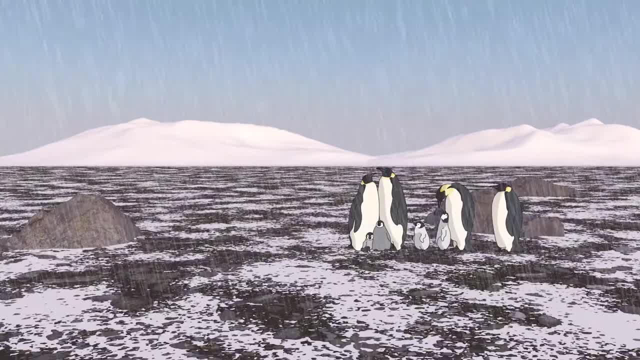 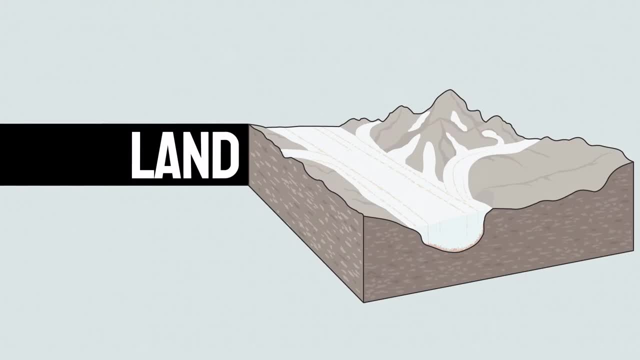 Rain not only speeds up ice melt, it can also affect animals used to snow. Young penguins with wet feathers, for example, get hypothermia and get sick Land. Here, the warming climate is thawing the permafrost which releases stored gases like carbon dioxide and methane. 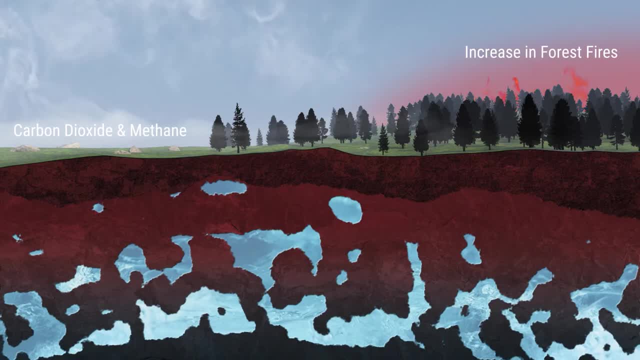 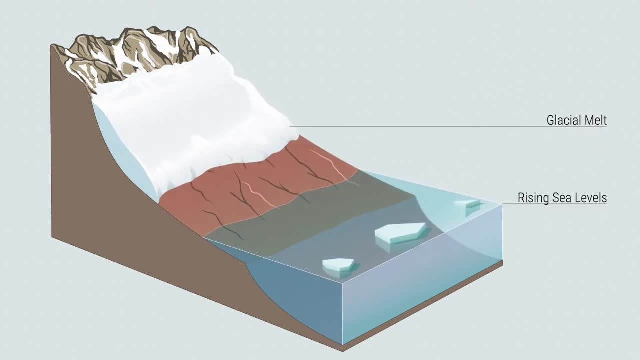 And drier conditions are leading to an increase in forest fires. Warmer climate also melts glaciers and speeds up movement of ice sheets across the continents. More ice then breaks off and falls into the ocean, causing a rise in sea levels. Oceans. 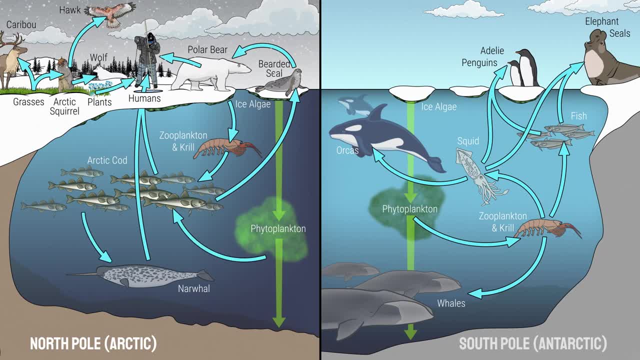 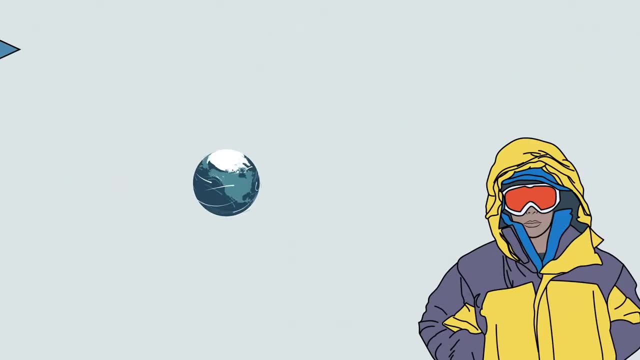 Loss of sea ice disrupts the polar food webs. This isn't just starving polar bears. Less ice also means less plankton, An important food source that a lot of species currently depend on. Climate change is happening all over the world, But the things happening at the poles are important indicators for the future.